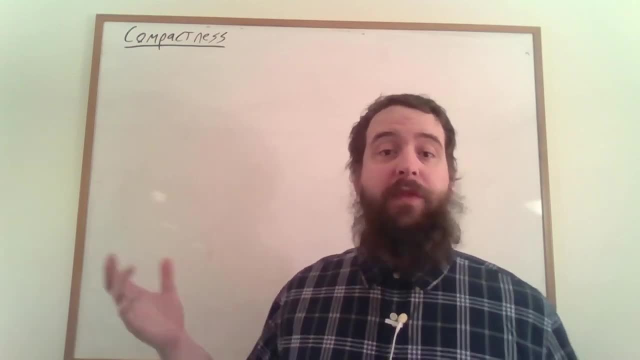 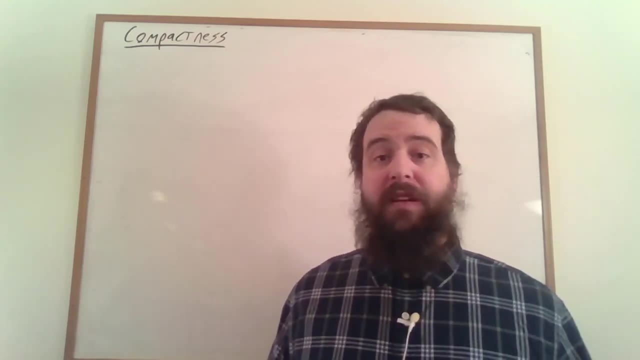 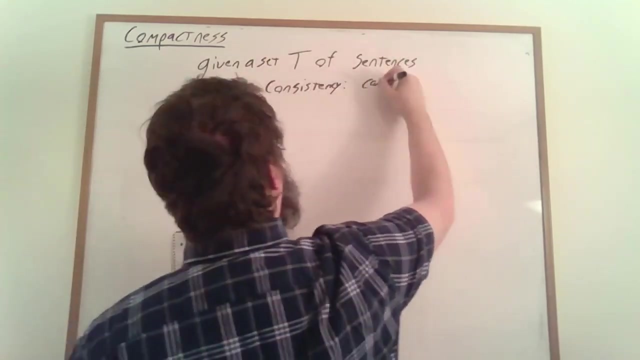 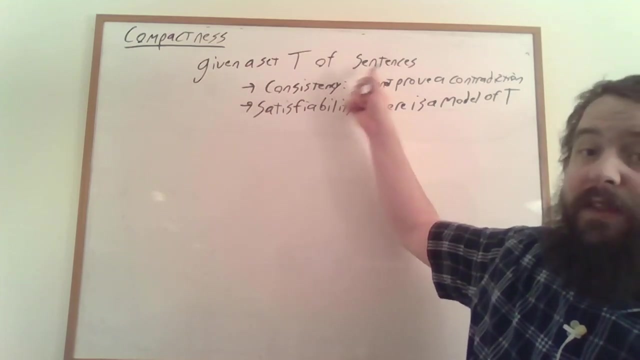 concerned as logicians. compactness is a theorem that allows us to prove that certain models exist that have certain first-order properties. In this video, I'd like to contrast two important concepts: consistency and satisfiability. So, given a set T of first-order logical formulas without any free variables in them, 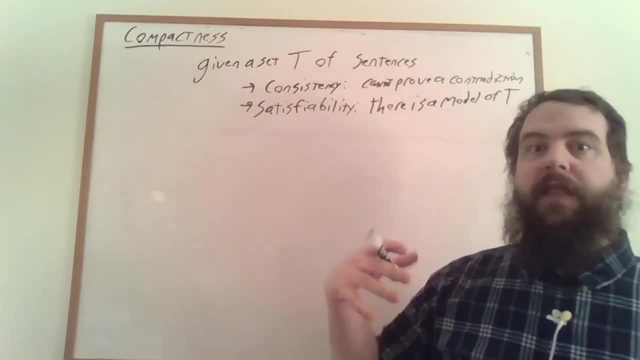 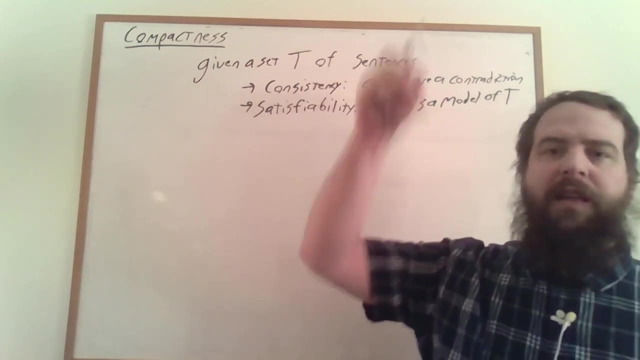 we're going to call these sentences, And so a first-order logical formula with free variables in it is meant to be something that you can plug things in In for those free variables, and it winds up either being true or false of the values that. 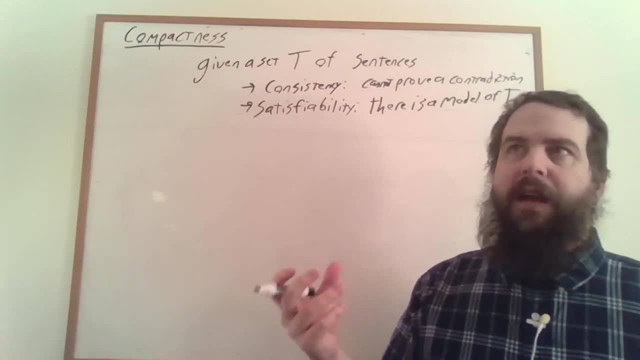 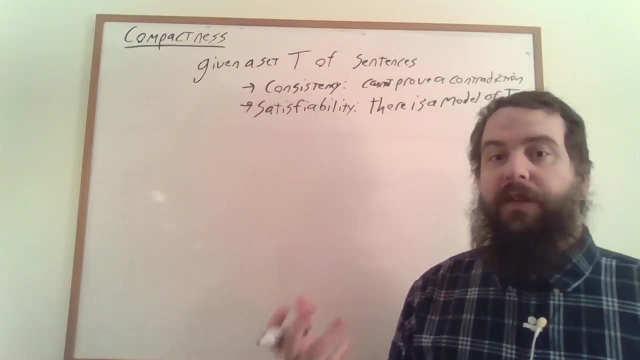 you plug in. So really, it's something that it depends on what structure you're working in, but it also depends on what values you plug in. If we don't have any free variables, the sentence is either true or false for any one particular structure. For instance. 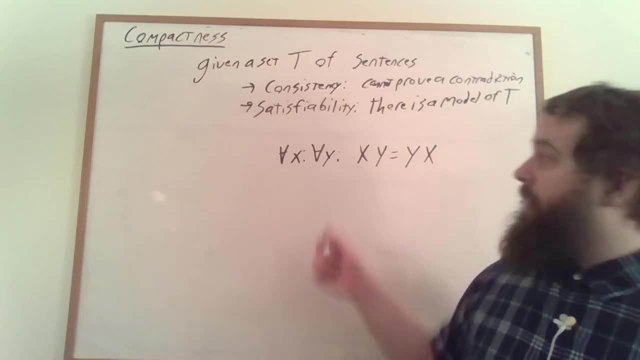 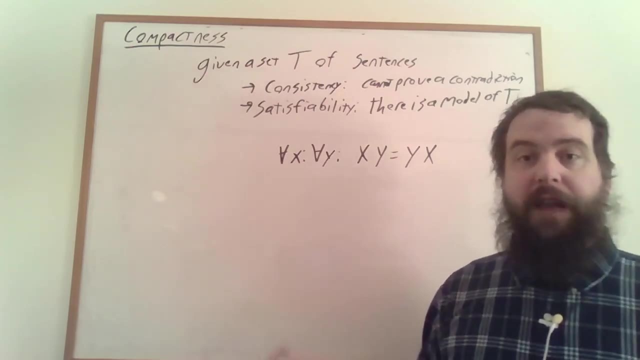 if we have this sentence in the theory of monoids, that for any x and for any y, xy is equal to yx, well, there are some monoids where this is true, such as the natural numbers under addition or multiplication, and there are some monoids where this is false, such as the word monoid. 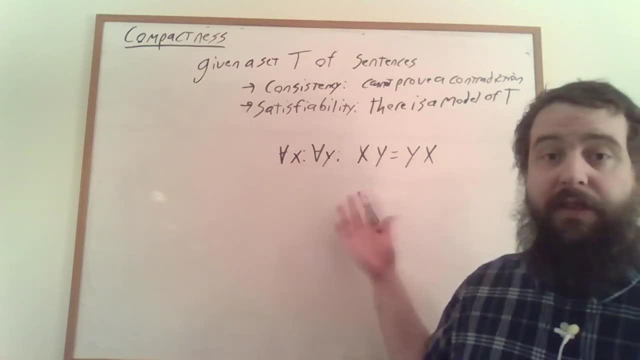 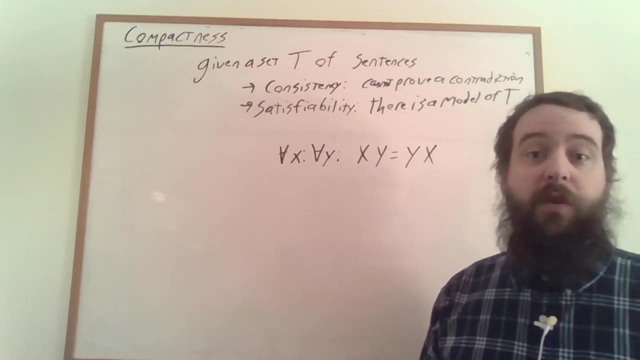 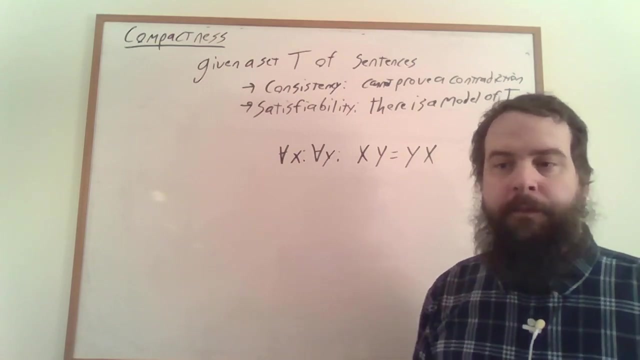 So this sentence here- because it doesn't have any free variables- is true or false, depending on what structure we're looking at. When we're talking about sets of first-order logical sentences, we like to call them theories, So I've used the letter T for this collection of sentences. Now there's two things that we could hope. 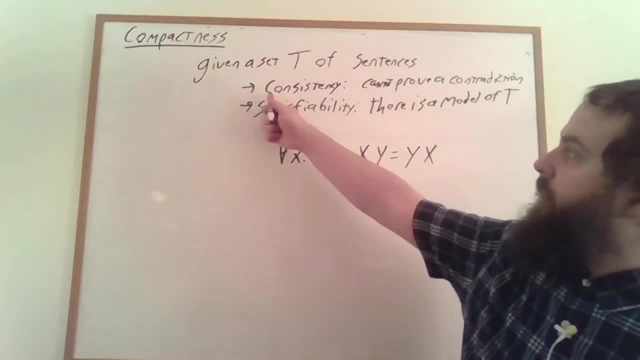 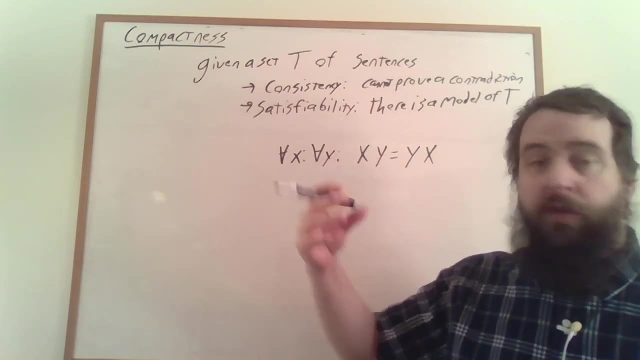 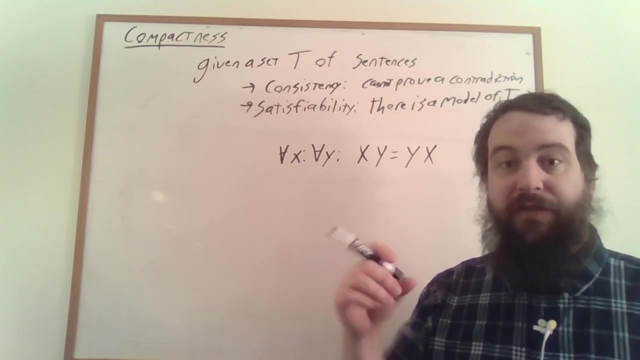 from this collection of sentences. We could hope that this collection is consistent, That is, that we can't, starting with our sentences, prove a contradiction, And you can either have a special Boolean constant for falsehood and a Boolean constant for truth, And you could say: 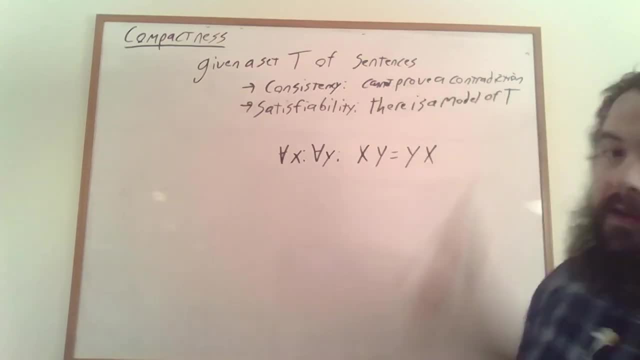 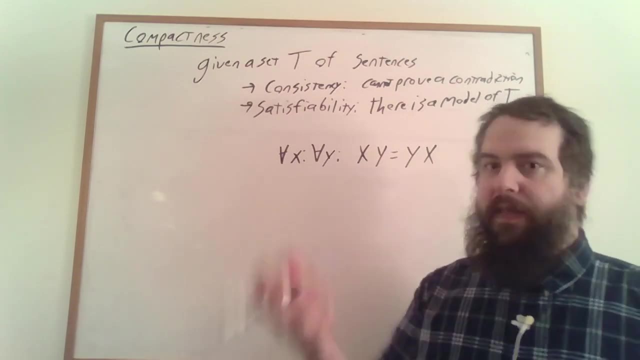 oh well, we don't have a proof of falsehood, Or you could just say we don't have a proof of a formula, of the form. something is true and not that something is true And it turns out. the details of our proof system don't really particularly matter. 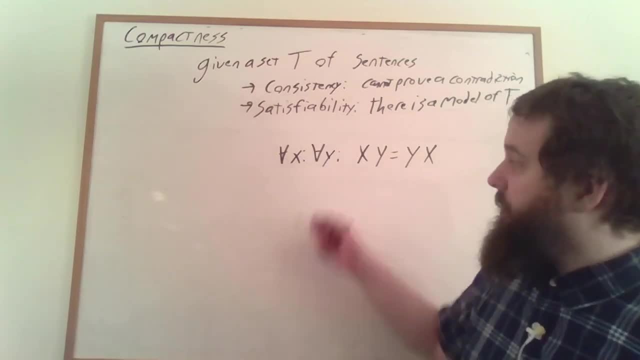 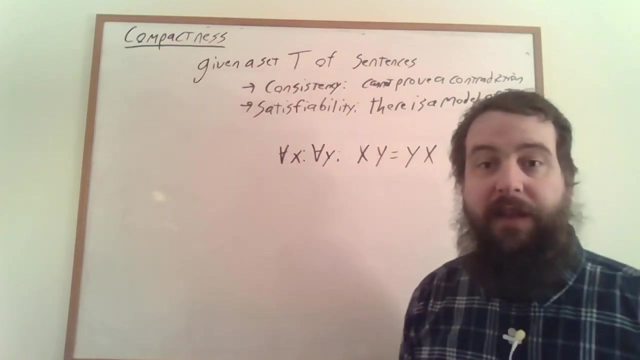 We should simply have in mind that our proofs consist of a sequence of lines. Any of the lines is either an axiom or maybe one of the hypotheses, one of the things that we're trying to prove things from, an element of our set of sentences. 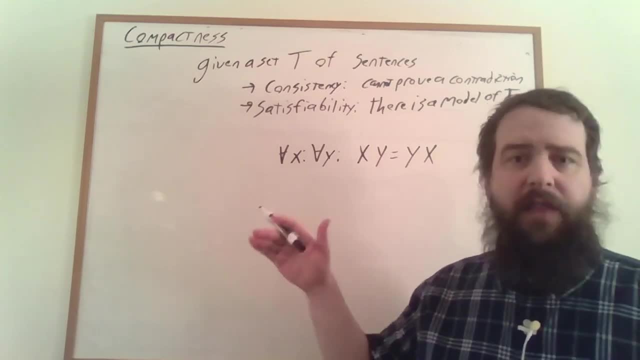 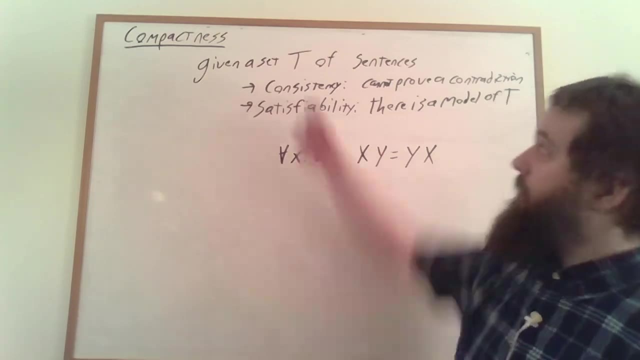 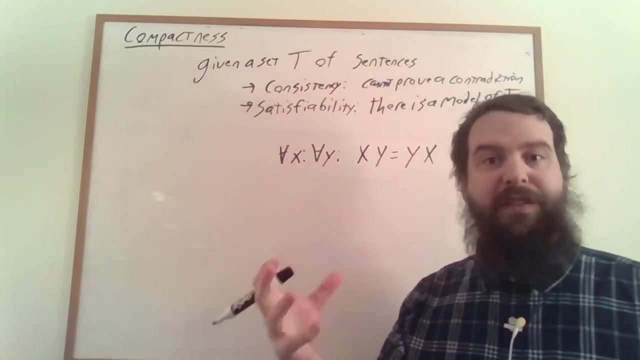 Or a line that follows from previous lines, by a particular deduction rule, from a small set of deduction rules, And so we could hope that, given a set of sentences, that we can't prove a contradiction from those sentences, That those sentences don't contradict each other. 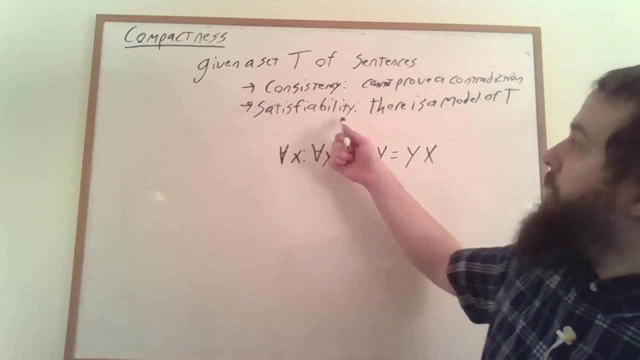 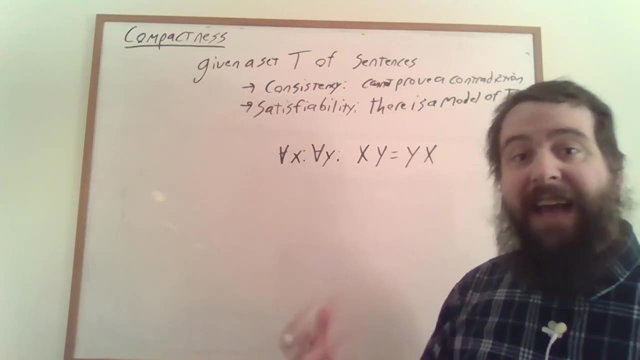 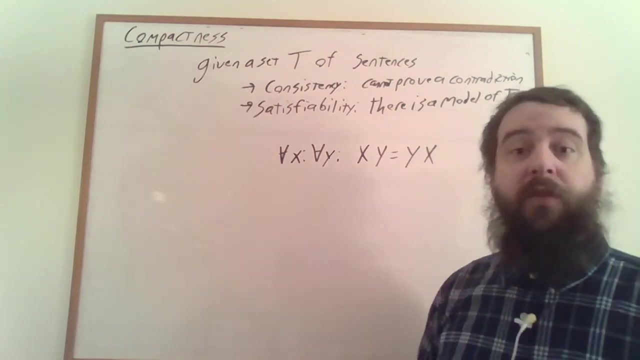 Another thing we could ask for is satisfiability. Is it the case that there's a model? Is it the case that there's a structure that satisfies all of these sentences, Such that all of these sentences are true for that particular structure? Of course, if a collection of sentences is true with very few philosophical assumptions. 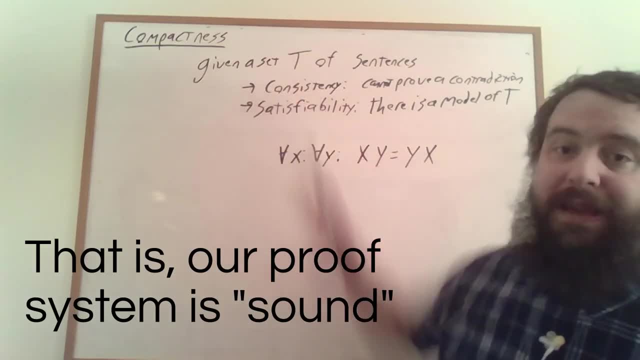 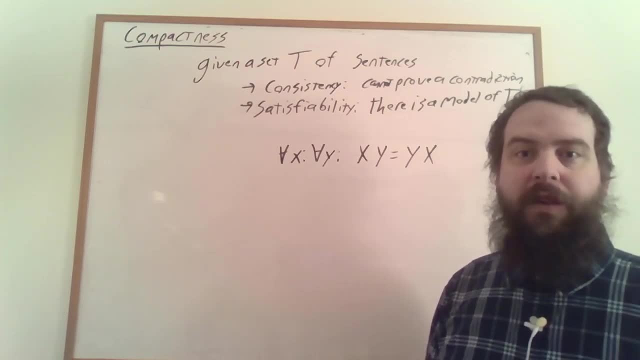 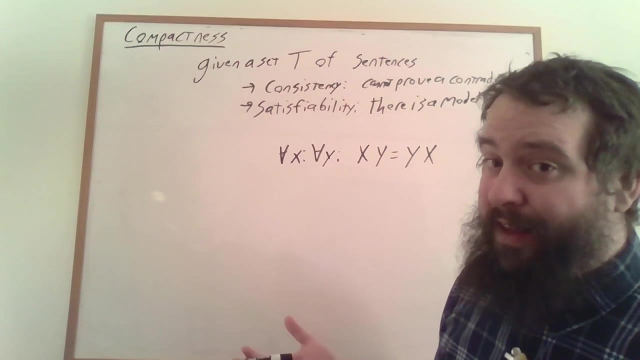 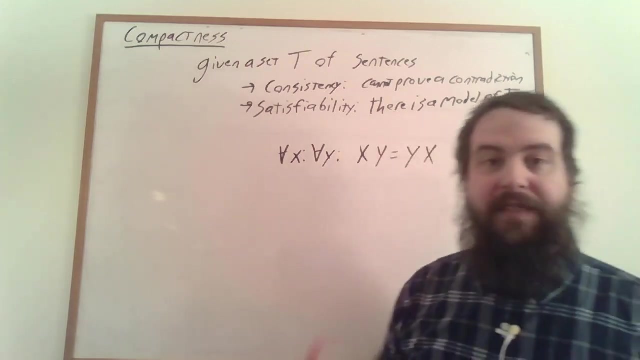 we know that that set of sentences has to be consistent, Because inconsistent things aren't true of actually existing structures. But is the reverse true? If we have a consistent set of formulas, potentially an infinite set of formulas- is it necessarily the case that we can find a structure that satisfies that collection? 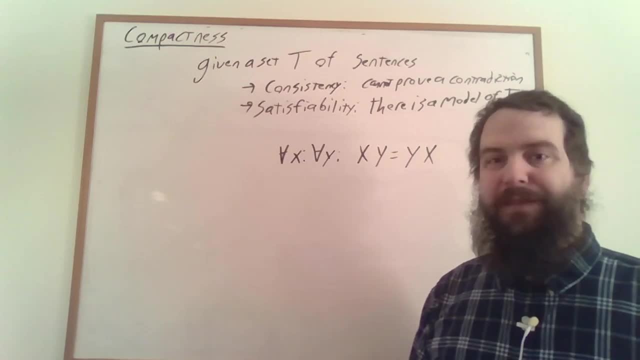 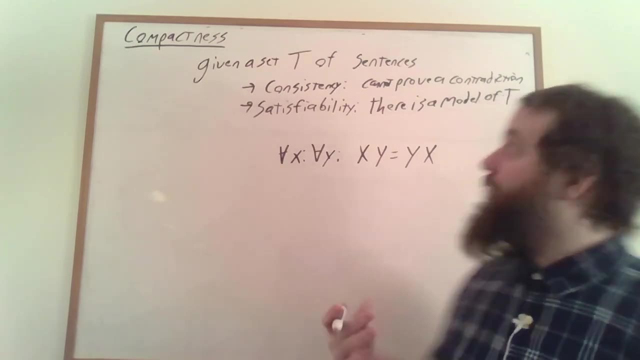 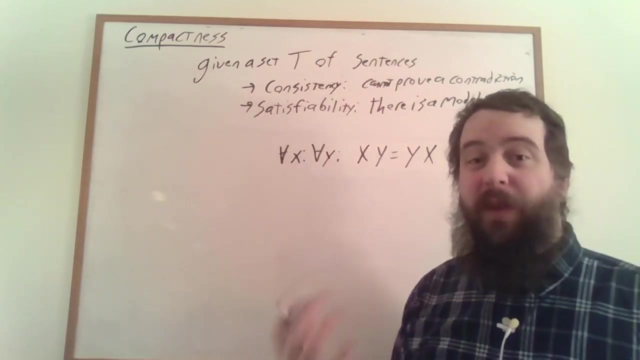 of formulas, It turns out that the answer is yes. But let's take a moment to imagine what would happen, what the world would be like if the answer was no, If there were collections of sentences that were consistent but weren't satisfiable, that there wasn't a structure satisfying that. 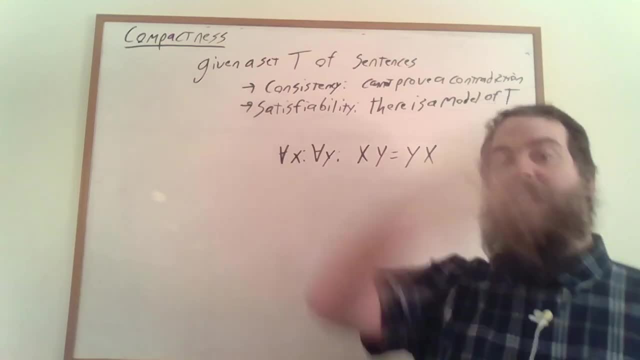 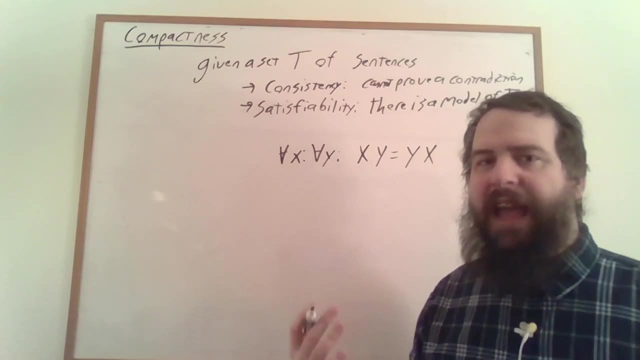 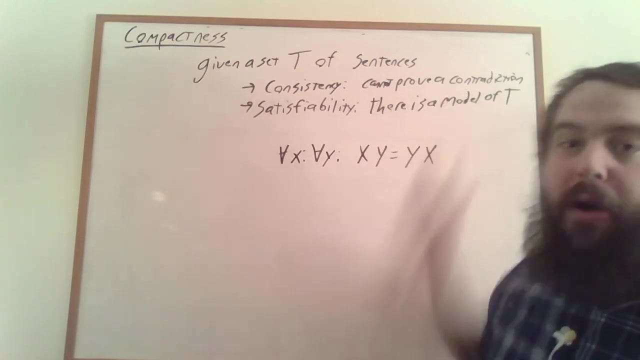 collection of sentences. Then we'd have this difference, but we couldn't find a structure to this collection of sentences that, by virtue of being consistent, behaved kind of like the collection of true things, of an actual model, but there wasn't any model that they were the. 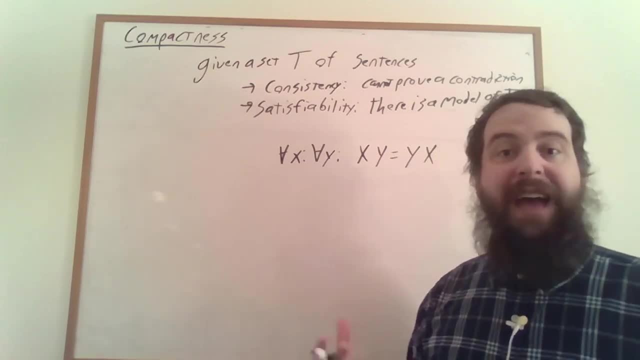 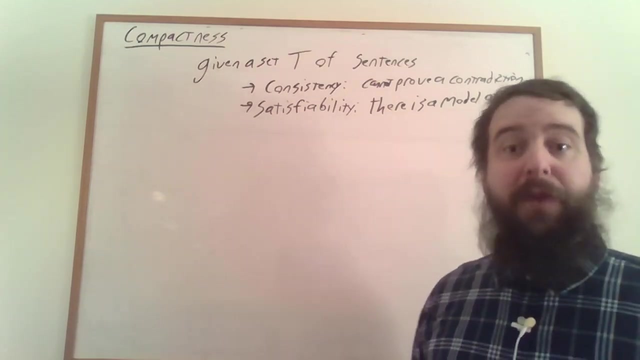 collection of true things, for It would act like a collection of true things for a virtual model in some sense, and it would behave a lot like a collection of true things for an actual model. But no, it is the case that if we have a consistent set of sentences, 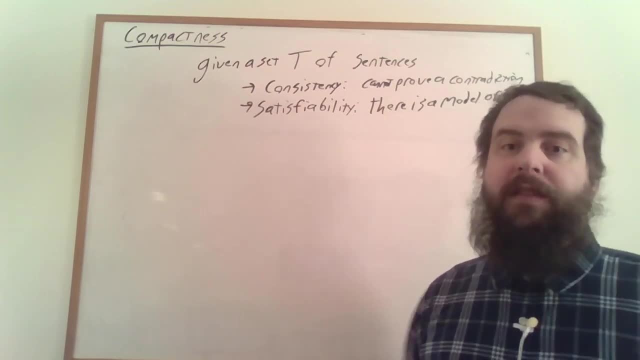 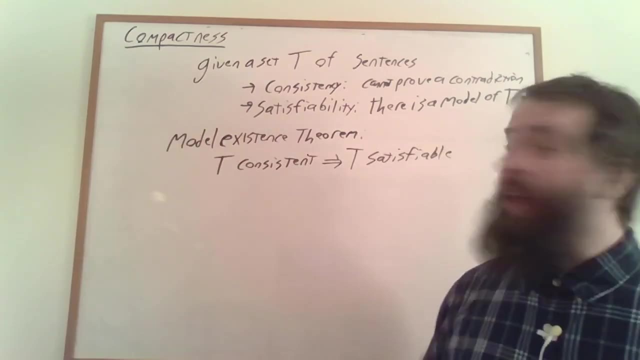 then it must be satisfiable. This is called the model existence theorem, That if we have a collection of first order logical formulas and it just has to be a set, it doesn't have to be a full set, it just has to be a set of first order logical formulas. 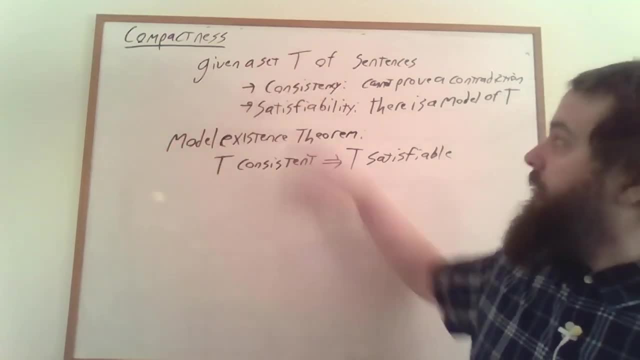 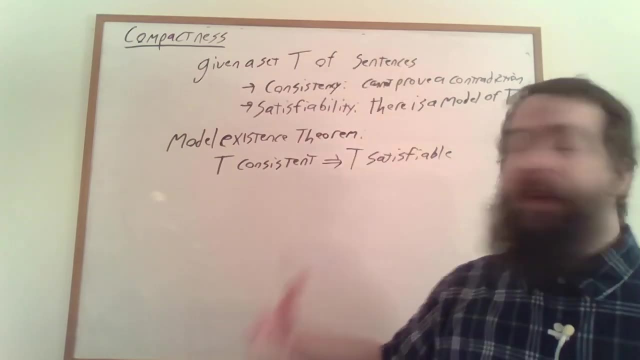 it doesn't have to be a full set of first order logical formulas, it just has to be a full set of first order logical formulas. finite collection: it could be an infinite collection. If we have a collection of first order logical formulas, sentences that are consistent with each other, then we can find. 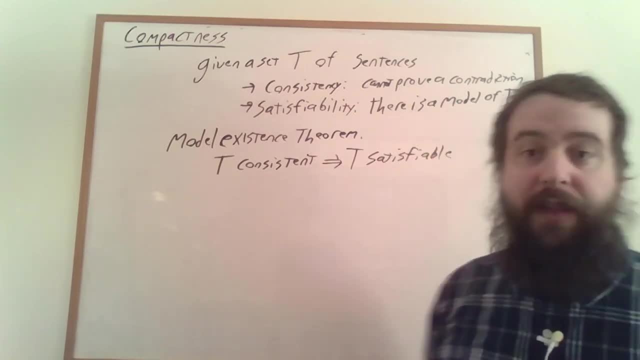 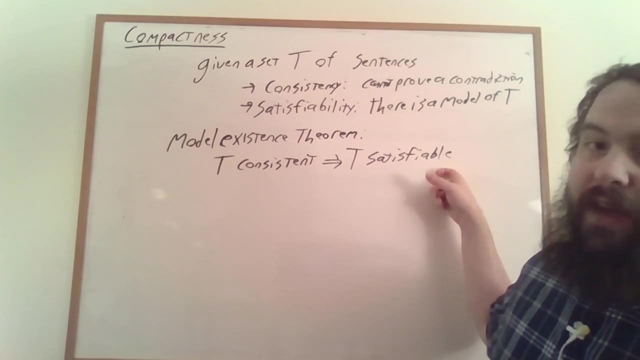 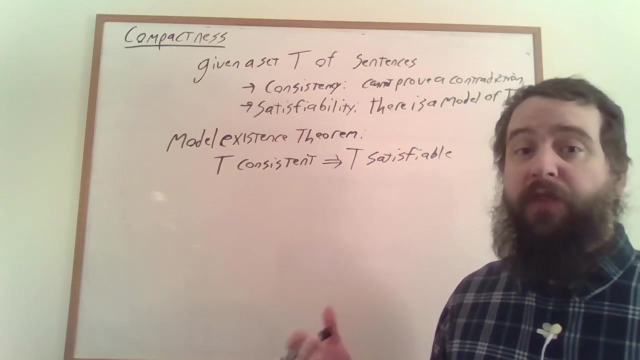 a structure. we can find a model of that collection of sentences, of that theory, And of course this is an if and only if. If it's satisfiable, then it's consistent, because it has to be In this video. I'm not going to bother too much with the proof of the 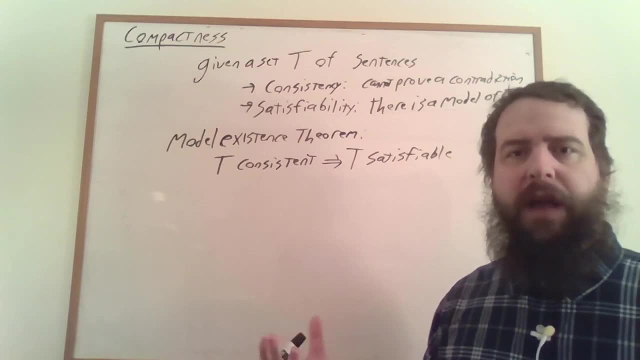 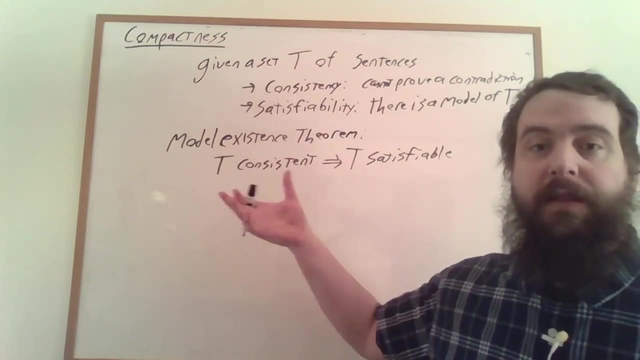 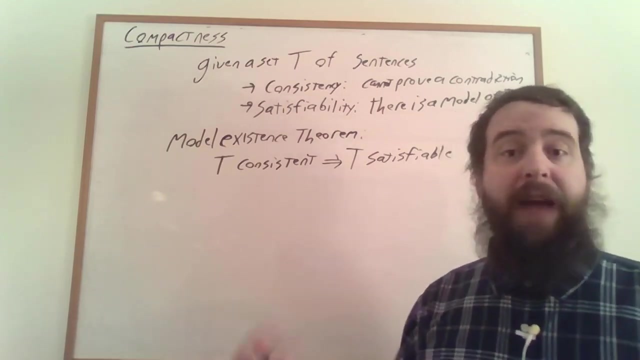 model existence theorem. I'll give you some intuition as to why it's true and I'll link you to some resources down below. But I want to show you what we can use the model existence theorem for, And typically the model existence theorem is used through the compactness theorem. 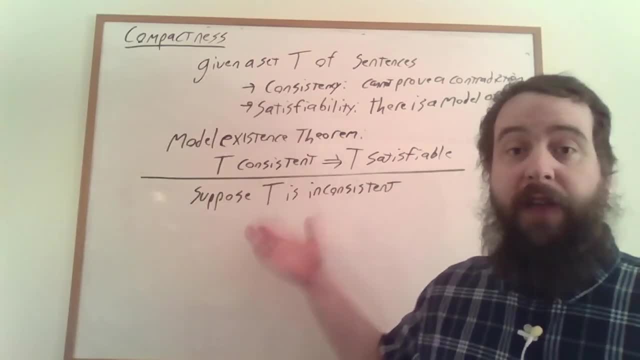 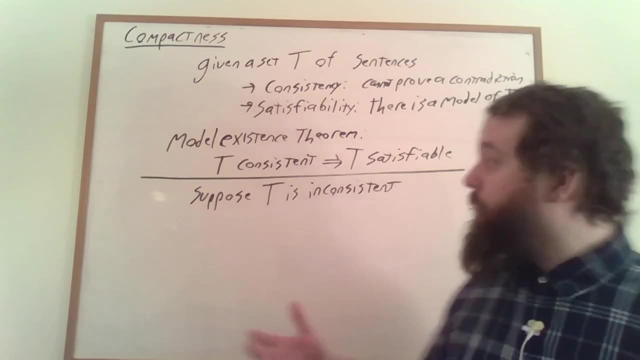 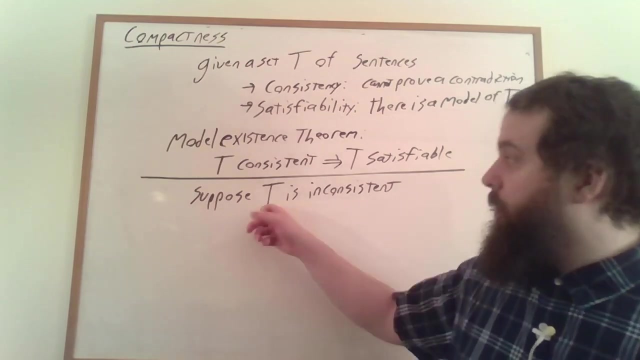 Suppose for a moment that our theory, that our set of first order logical formulas is inconsistent. What does that mean? That means that there's some proof where each line is either a valid deduction from previous lines or one of our axioms or one of our elements of the theory. 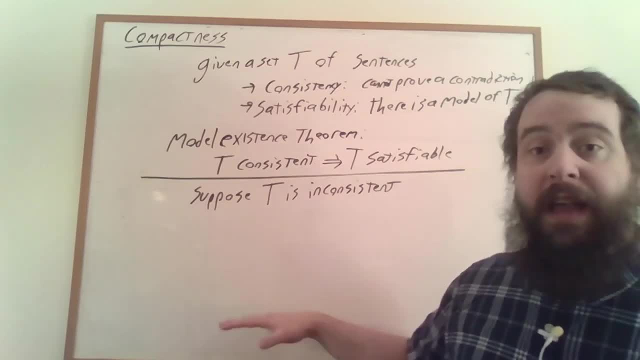 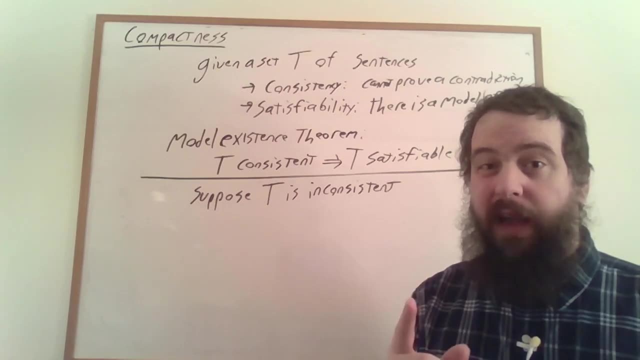 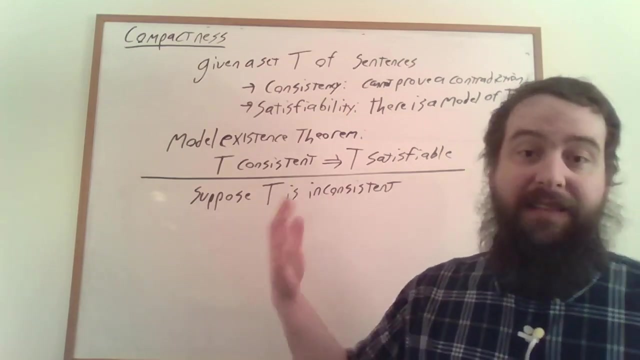 one of our elements of this set, whose last line is some sort of contradiction. But let's think carefully about what that proof is going to look like. Proofs have to be finite. So even if t is an infinite set- and that's something that we're going to be interested- 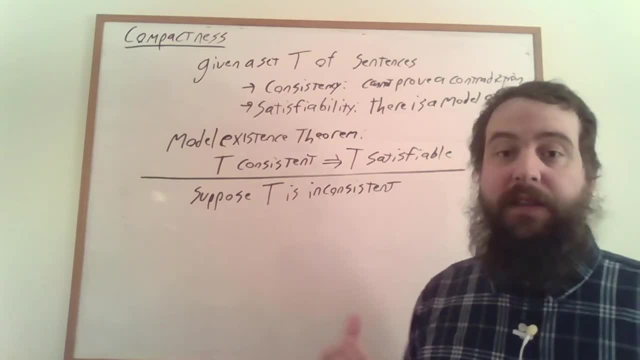 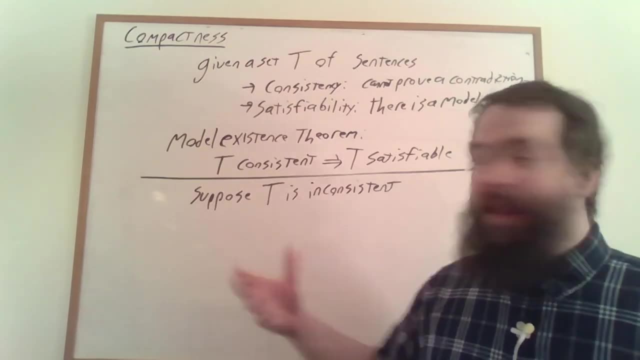 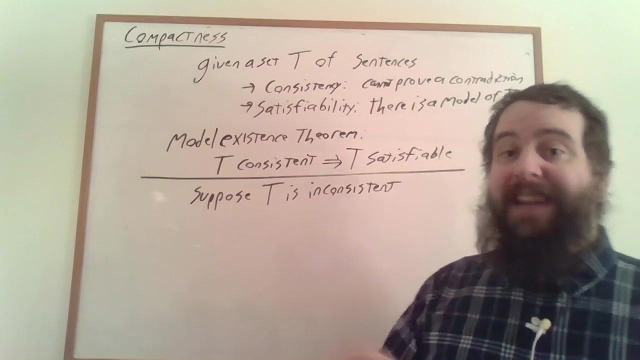 in looking at cases where t is some infinite set. Even if t is infinite there's, we're only going to use finitely many sentences in t in our proof, And so that means that if t is inconsistent, then this finite set of sentences, finite subset of t, is already inconsistent. 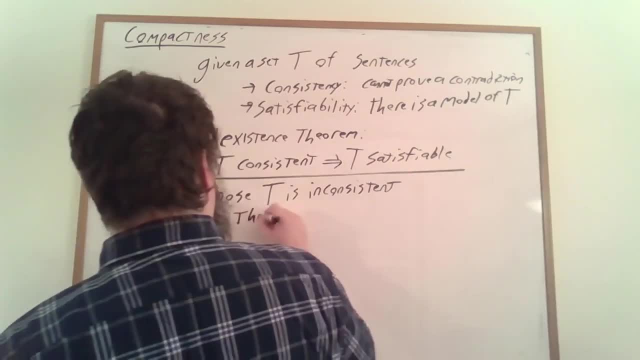 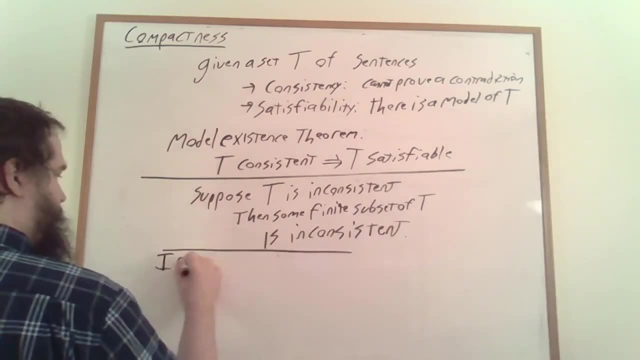 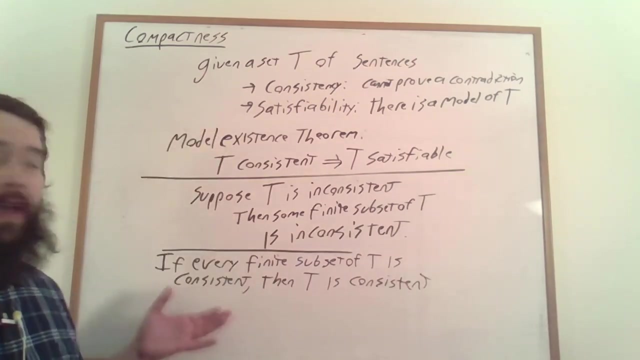 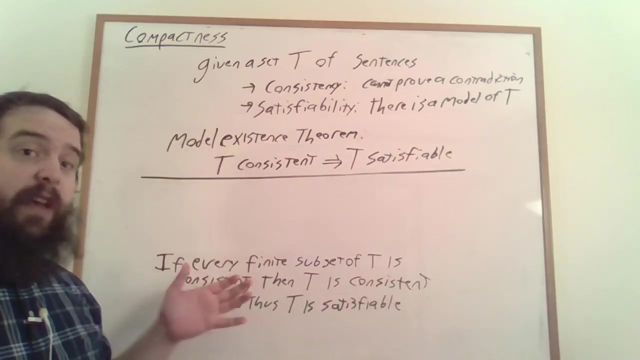 If t is consistent, then t is also consistent. And again, this is just the subtlety of the fact that all of our proofs have to be finite By the model existence theorem. if t is consistent, then t is satisfiable, And vice versa. if every finite subset of t is satisfiable, then 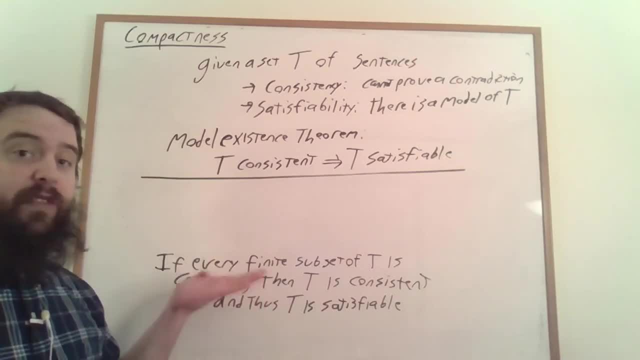 every finite subset of t is consistent because satisfiability implies consistency. So if we have a collection t of sentences where every finite subset of t is satisfiable, then it's going to be the case that every finite subset of t is consistent because 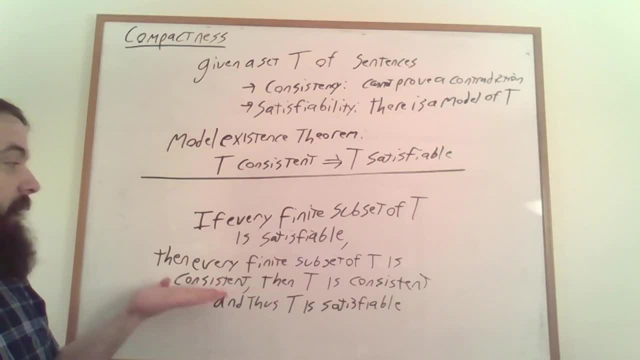 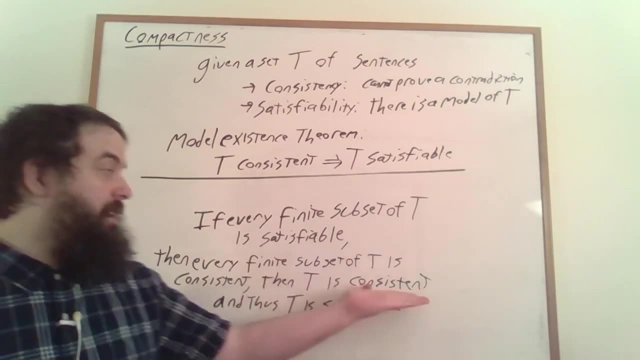 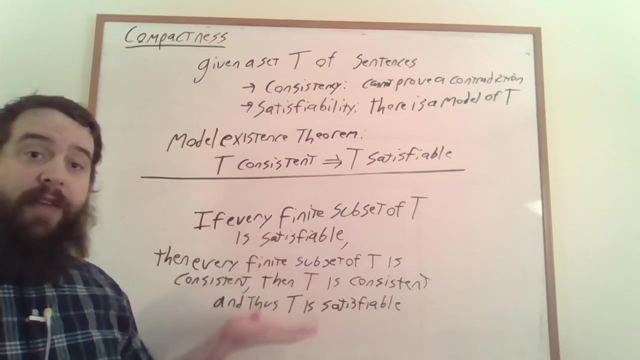 they're satisfiable By our contrapositive. that means that t our entire collection, which again might be infinite, is consistent and therefore our collection t is satisfiable So together. this is the principle of compactness, that if every finite subset of some collection 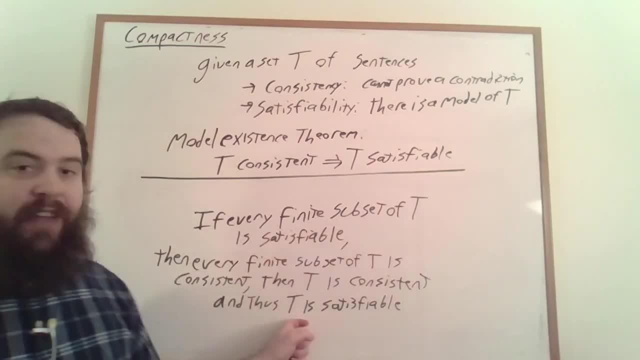 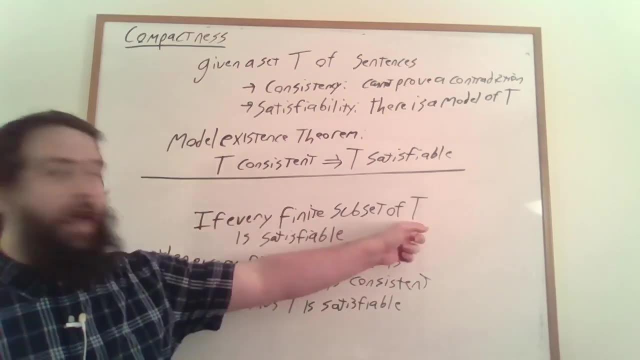 of formulas is satisfiable, then t is consistent. So if every finite subset of some collection of formulas is satisfied, then the entire collection of formulas is satisfied. If we can find a model of every finite subset of a collection of formulas, we can ecfl find. 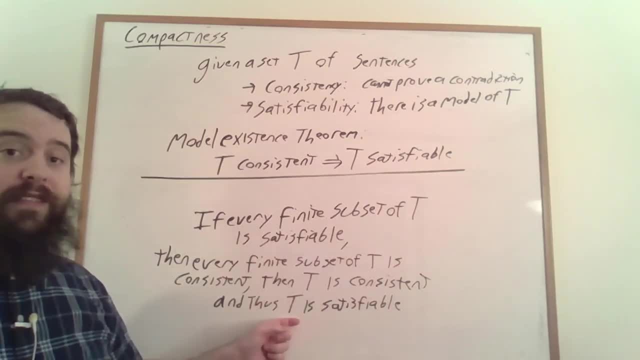 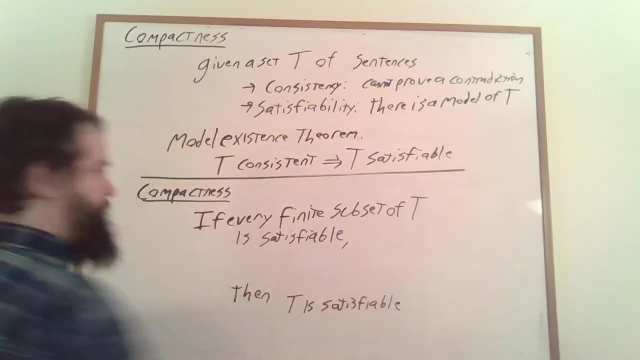 f of the entire collection of maxims whose function is limited to the nostril. so our еш isbb sub t. So this is our principle of compactness. Now, the principle of compactness doesn't tell us much about compa, sanct pt. 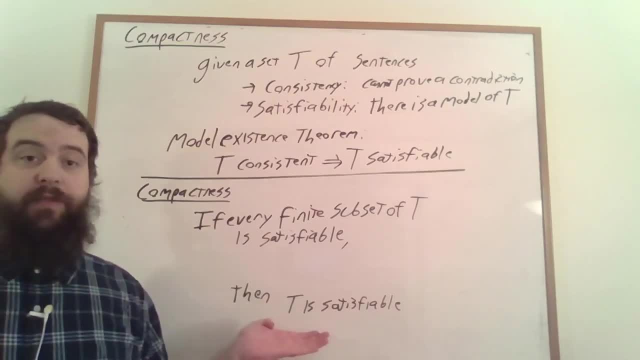 model actually is going to satisfy this particular set of formulas. By looking carefully at the proof you can actually get some nice bounds on the size of the model that's going to satisfy your collection of formulas. They usually wind up not being that big. Very often they'll wind up being countable And it's worth. 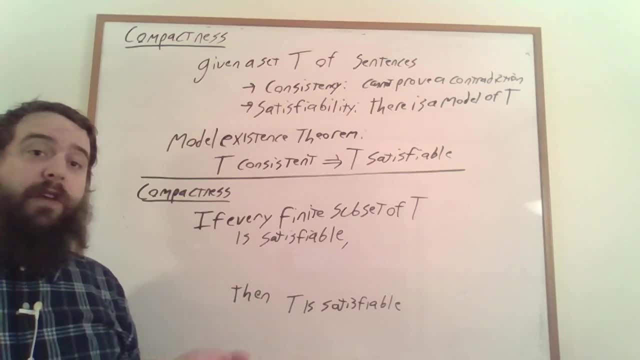 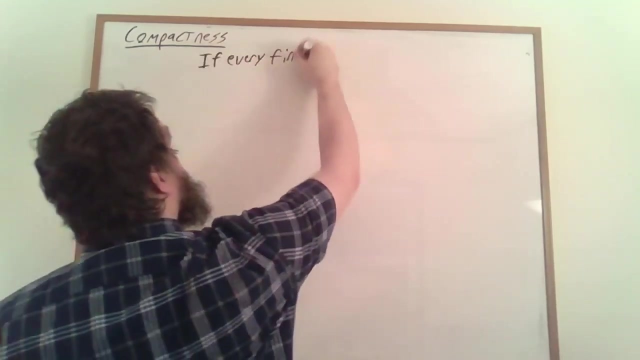 noting that the model existence theorem makes heavy use of the axiom of choice. So this process of producing a model for an entire collection of formulas, the resulting model might be a little bit uncomputable because it's got the axiom of choice in it. 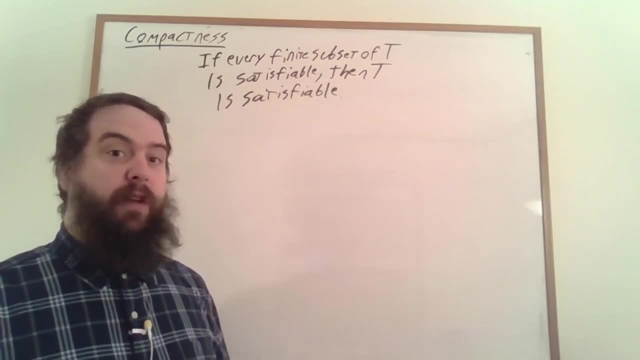 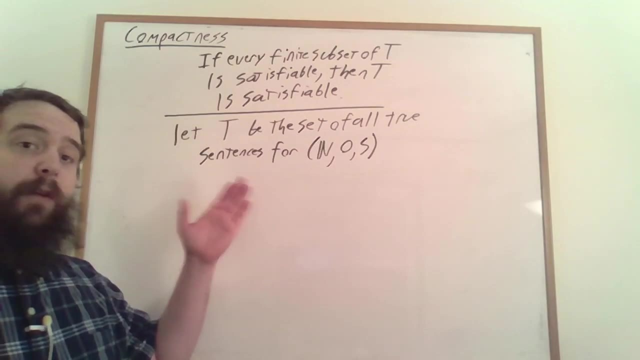 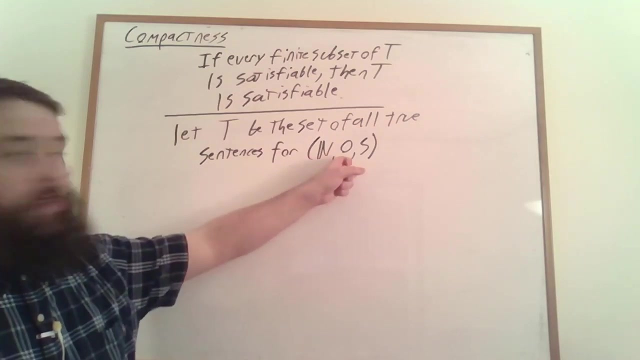 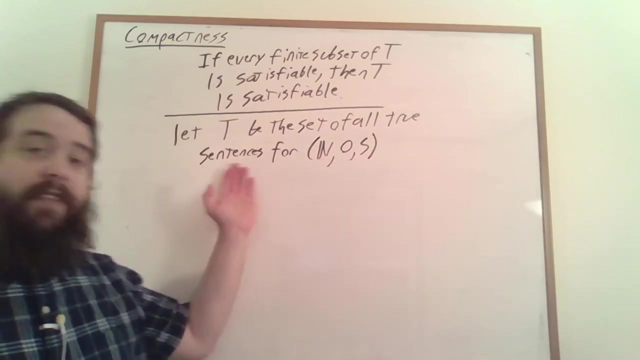 So let's take a look at an example application of the compactness theorem. Let's start by letting t be the set of all true sentences in the structure of the natural numbers, with a special constant indicating zero and the, the successor operation, the plus one operation. Together, this set of sentences is called the. 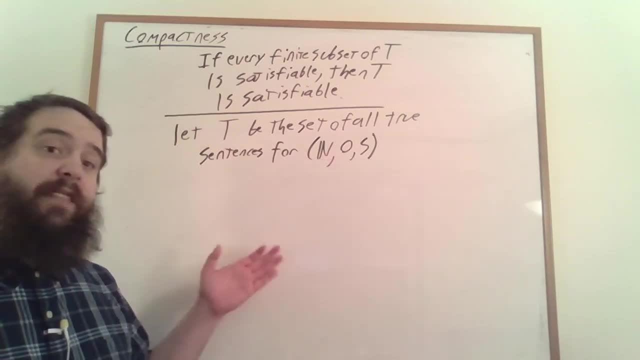 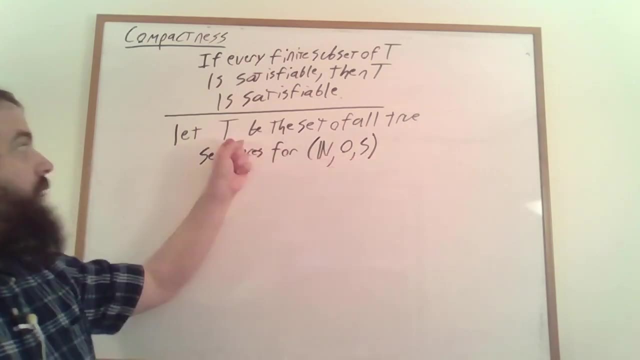 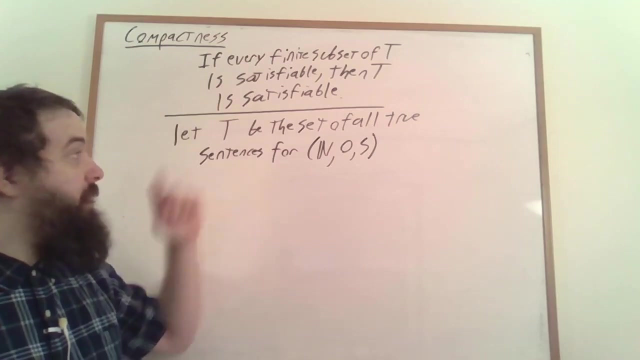 theory of this structure. And this theory is said to be complete because, for any formula, either the formula is true of this structure, in which case it's in T, it's one of the true formulas, one of the true sentences for this structure, or it's false, in which case it's. 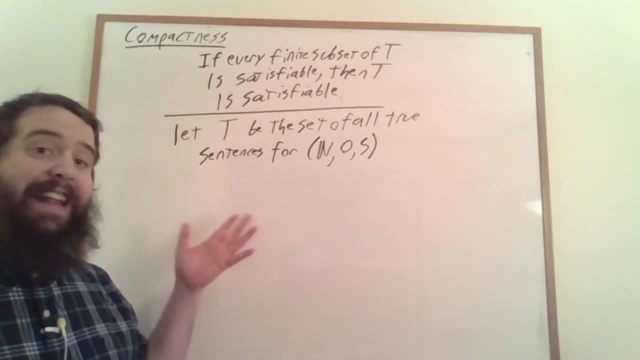 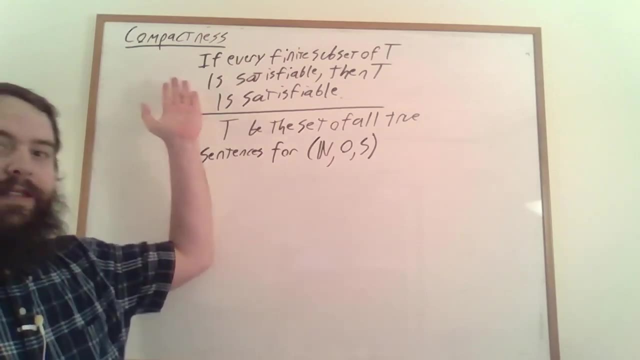 negation is in this collection, So we can't add anything to T without making it have a contradiction in it. Well, this is kind of boring from the perspective of the compactness theorem by itself. We know that every finite subset of T is satisfiable because they're all satisfied by. 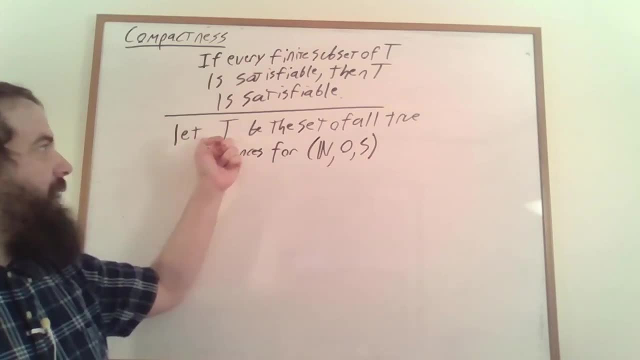 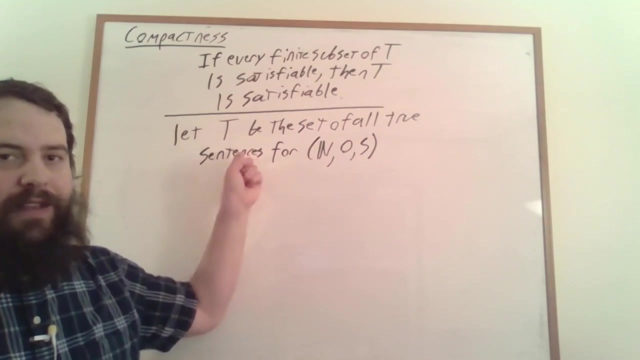 this structure here, right, Any finite set of sentences. that's true of this structure is true of this structure. And the conclusion of the compactness theorem says that the entire collection is satisfiable, that there's some structure that satisfies all of these sentences. Well, that's also the structure. So we haven't. 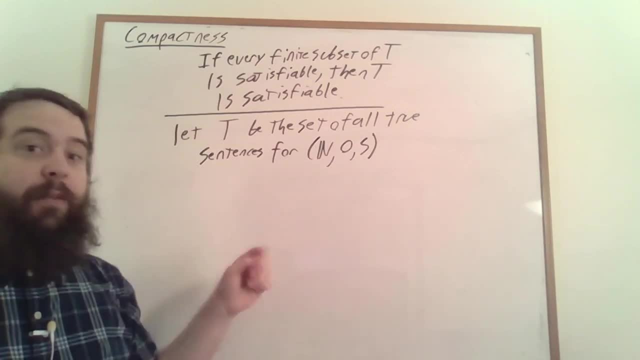 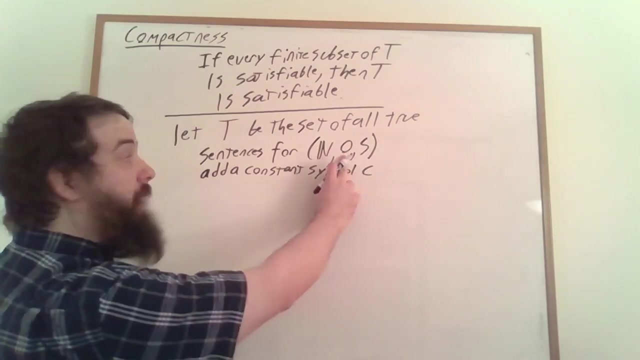 really gained anything from the compactness theorem yet. but let's add some new formulas into T, And in order to do so we're going to add in a new constant symbol, C. So our structure is going to be the natural numbers, with a constant for zero and an extra constant C. 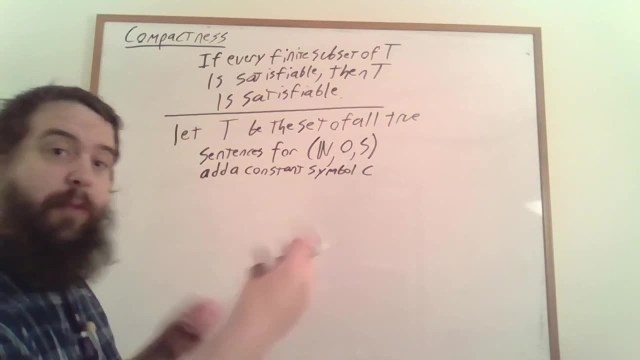 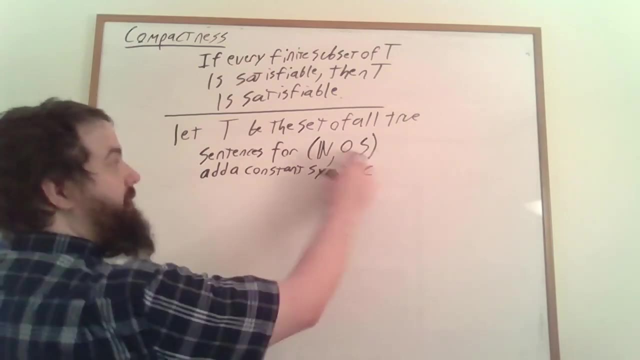 so we'll have two symbols that we can use to represent elements when we're constructing formulas, when we're constructing sentences, in this first order logic, and then we can take the successor of those, we can take the successor of zero, we can take the successor of C. So C is going. 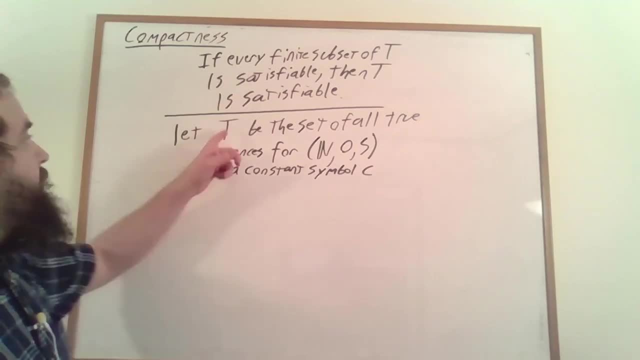 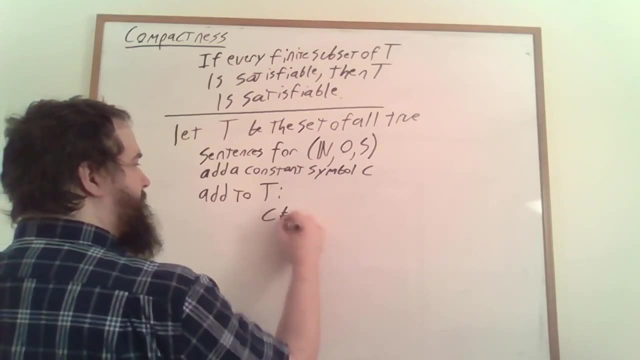 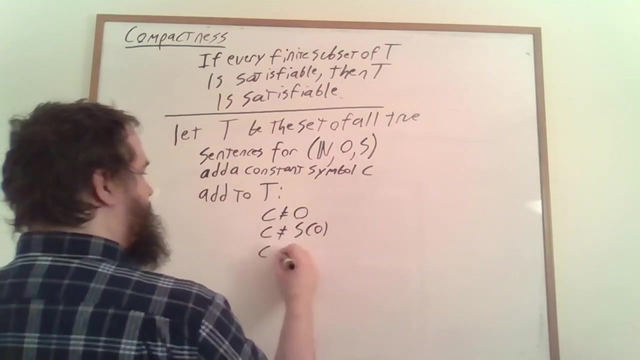 to be some constant and we're going to add a bunch of sentences to T. We're going to add that C is not equal to zero and C is not equal to zero, so not equal to the successor of 0, and C is not equal to the successor of the. 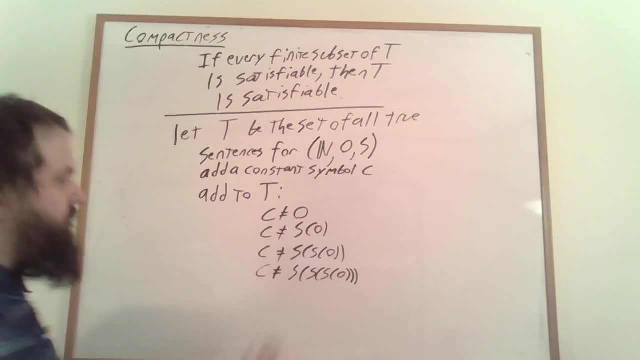 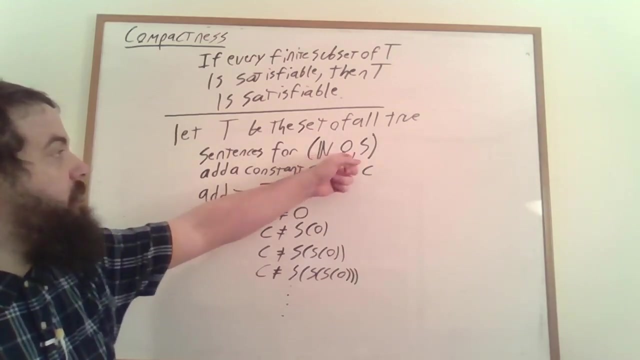 successor of 0, and so on and so forth. Any finite subset of this new collection is going to contain finitely many sentences from the original T and then finitely many of these new sentences that we've added on Together. this finite collection is satisfied by the natural numbers, with 0 and successor, just the. 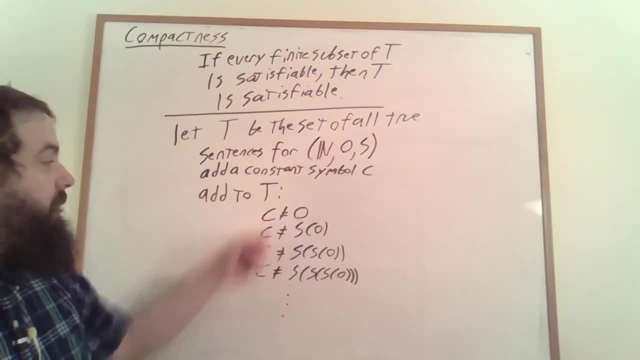 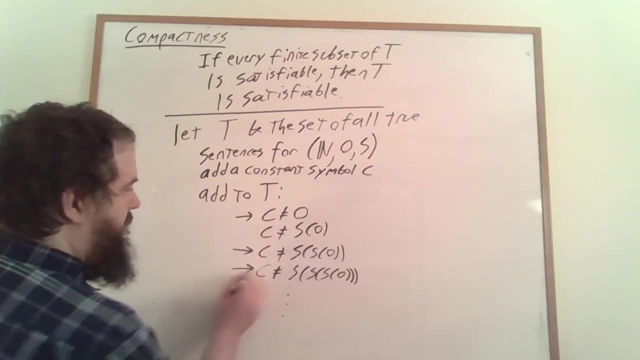 normal structure that we're used to, where C is assigned to be some large value, right? Some finite number of these are in our collection, so we're going to have to avoid, let's say, that just these three are in our collection, then we're going to have to avoid assigning the constant C. 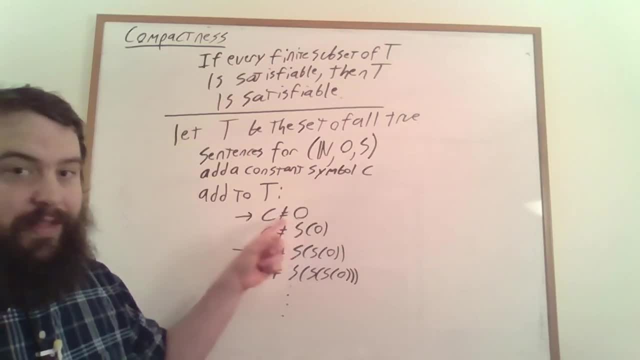 to zero, because that would be inconsistent with this assertion. here. We're going to have to avoid assigning the constant C to the number two. We're going to have to avoid assigning C to the number three, but there's only a finite number of these numbers. 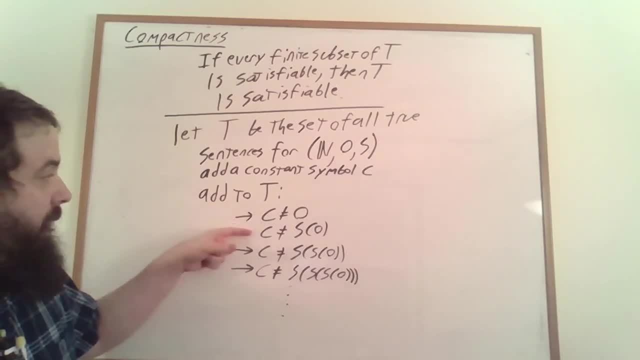 that we have to avoid assigning C, to Pick a number that we don't have to avoid and then assign C to that number, And therefore we can satisfy this finite collection here, along with our finite collection of things that are true for the original structure. 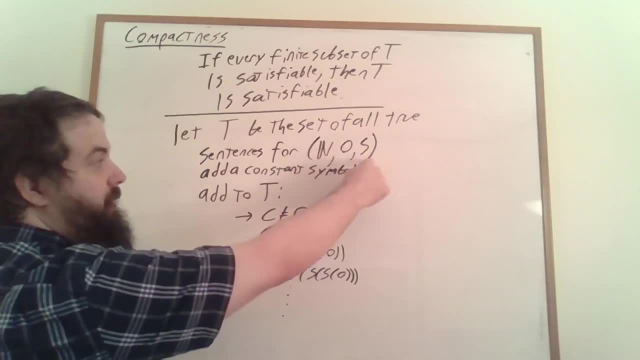 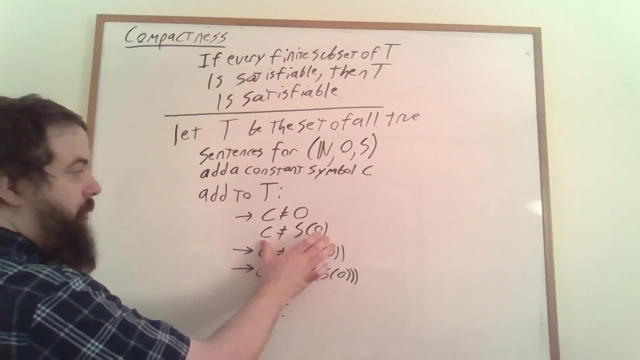 Again with the natural numbers zero successor and our assignment of C. in this case, C equals one, but assigning C to, let's say, the smallest number, that isn't prohibited because we have this finite collection here And this is a very common thing to do. 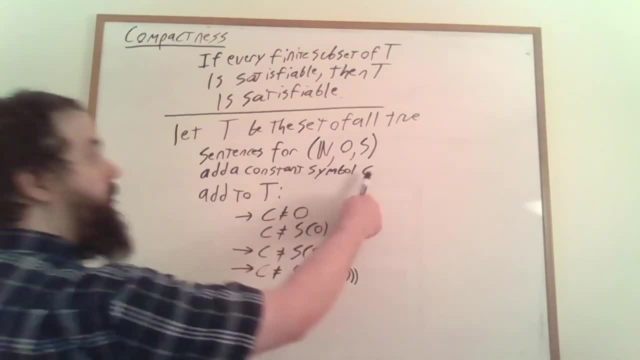 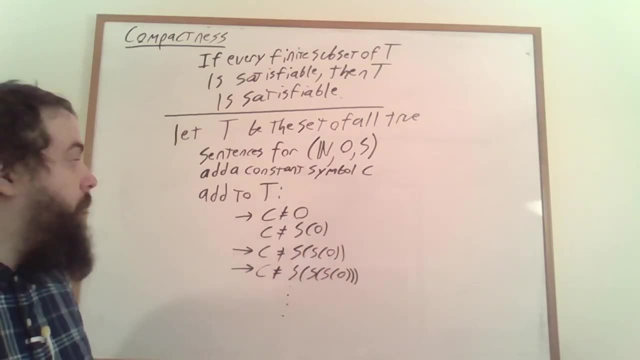 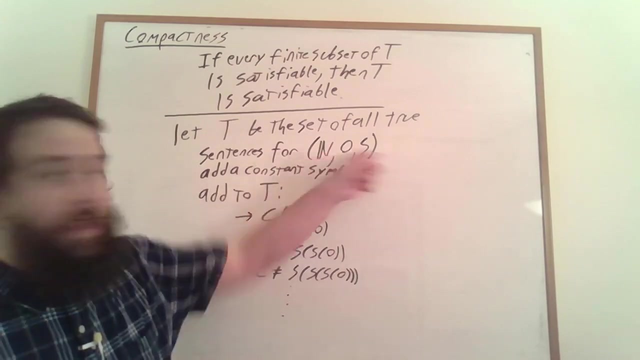 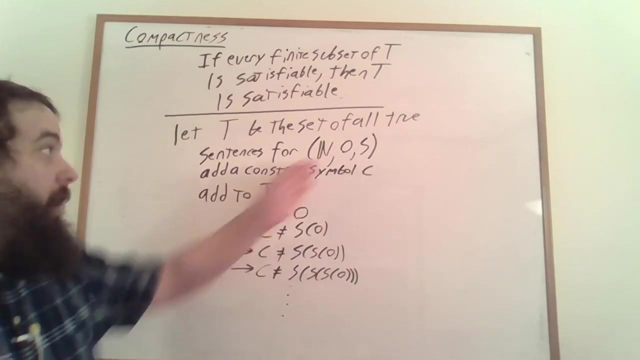 when you're working with the compactness theorem to create a new constant symbol and define a bunch of things that that constant symbol has to satisfy, where any finite collection of them is perfectly fine, is perfectly satisfiable within the original structure, But the infinite collection of them is not satisfiable. 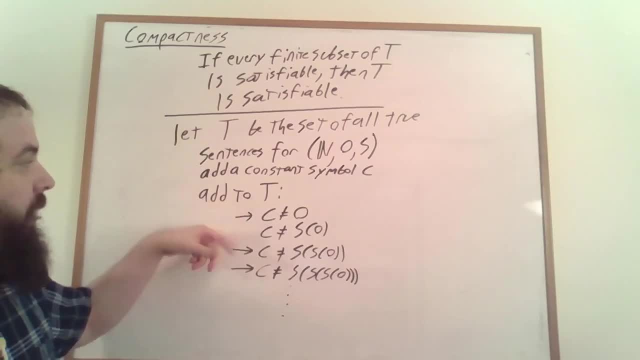 within the original structure, right? So here, if all of these sentences are going to be satisfied by some structure, we're going to have to assign C to some element of our model that isn't zero, isn't one, isn't two. 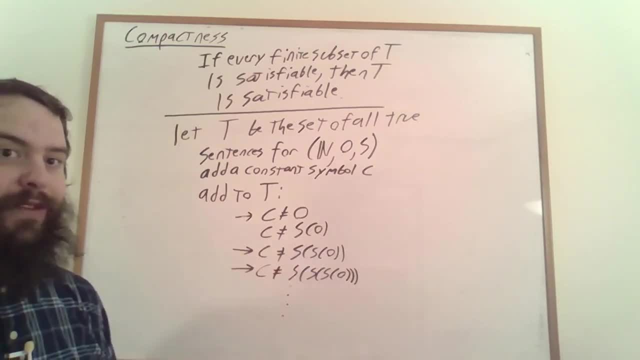 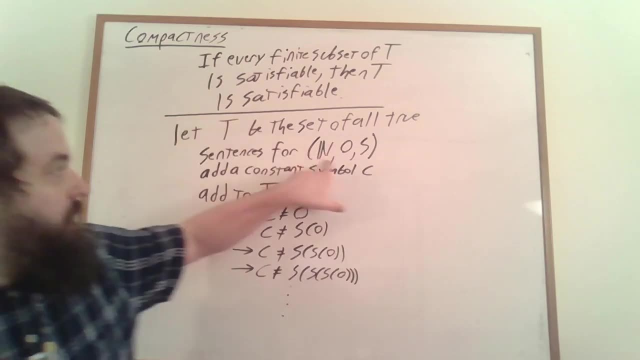 isn't three, isn't any of the natural numbers. So, in order for this collection of sentences, this entire collection, the theory of the natural numbers with zero and successor, all of these sentences, in order for this entire collection T to be satisfiable, we need to have 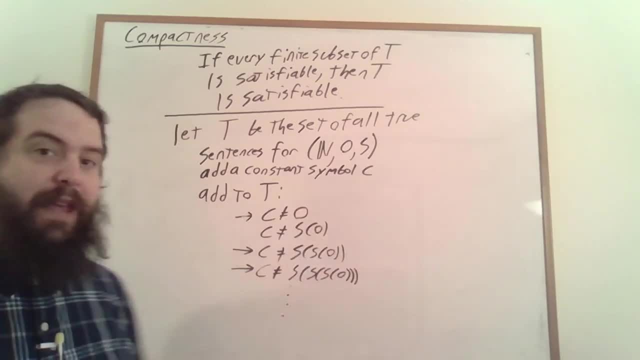 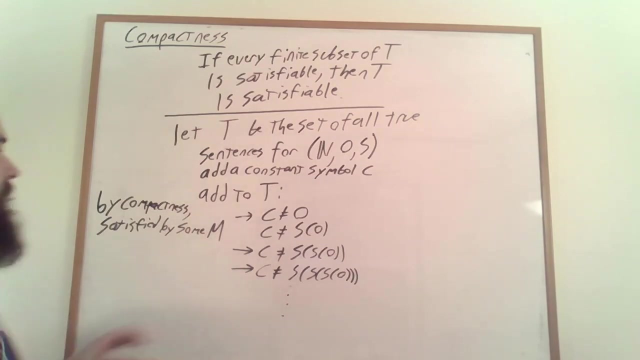 a new structure to satisfy them. It can't just be this structure with a clever assignment for C. So what does that structure look like? It's going to be some structure M, and this structure is going to have its own notion of zero, which we'll just call zero. it's the same: its own notion of successor. 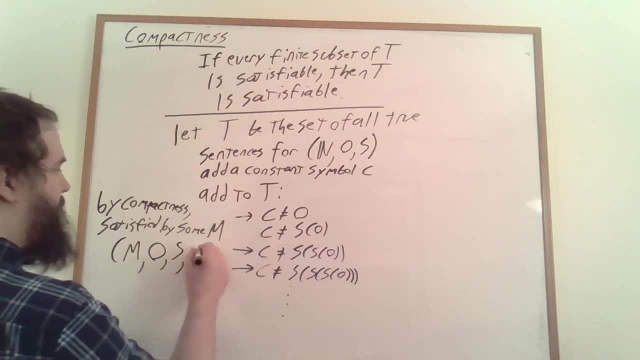 which we'll call successor, and some assignment of the value C. We know that this structure necessarily is going to contain zero and also the successor of zero and the successor of the successor of zero, and so on and so forth. All of these elements are going to be in our structure because, right, one of the sentences: 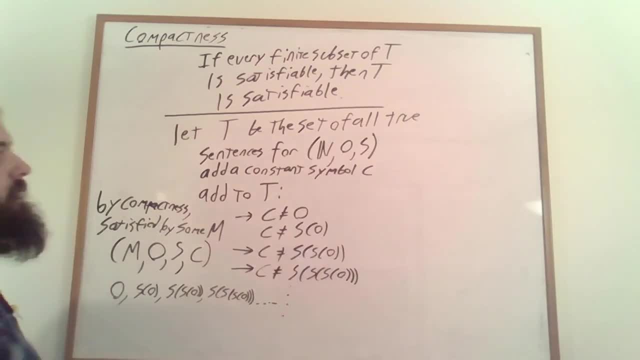 that's true of this original structure is that for any x, there exists a y, which is the successor of x. So it needs to be the case that, zero being an element of this structure and this structure satisfying this property, that the successor of zero 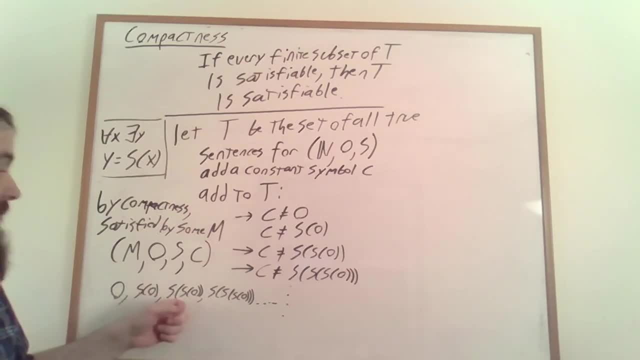 is also an element of this structure, and the successor of the successor of zero is also an element of this structure, and the successor of the successor of the successor of zero is also an element of this structure. Additionally, we know that these are all different elements. 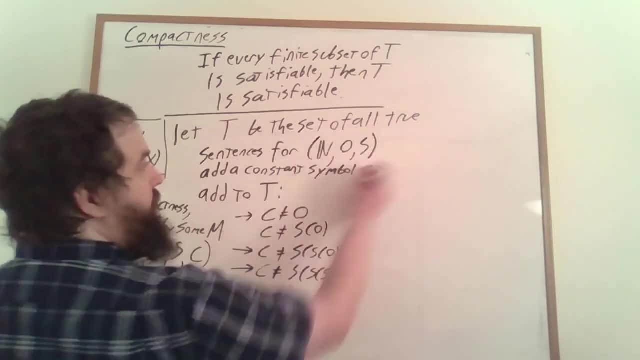 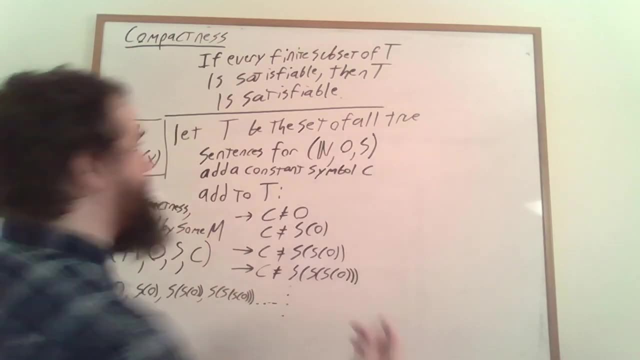 because within this original structure, we had the fact that, well, we had the basic sentence that the successor of zero is also an element of this structure. Additionally, we know that these are all different elements because within this original structure, we had the fact that, well, we had the basic sentence that the successor of zero is also an element of this structure, and the successor of the successor of zero is also an element of this structure. Additionally, we know that these are all different elements because, within this original structure, we had the fact that, well, we had the basic sentence that 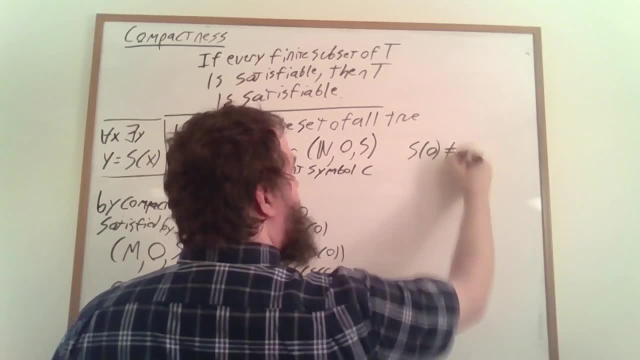 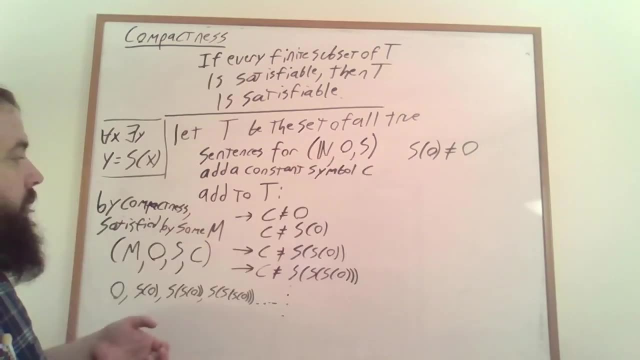 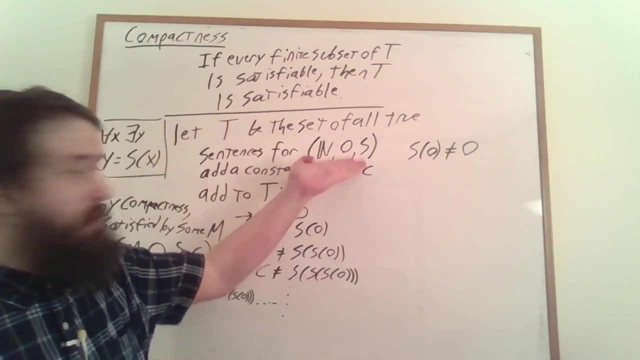 the successor of zero was not equal to zero, right. This is one of the sentences that's true of this particular structure, And so it's also going to be true of this structure here, because this structure has to satisfy all of the true sentences of this structure here. 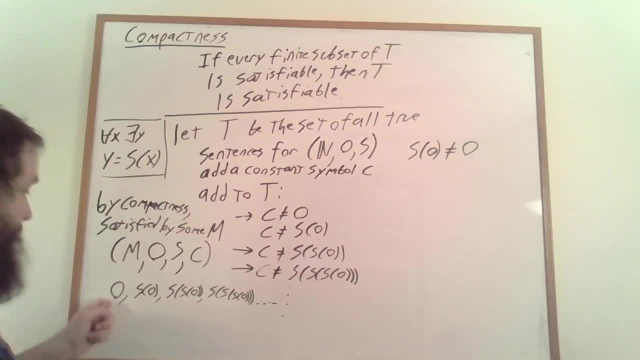 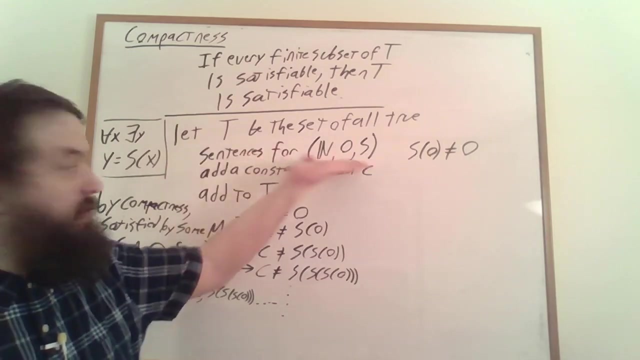 And similarly the successor of the successor of zero can't be equal to zero. It can't be equal to the successor of zero. None of these elements here can be equal to each other Because we have a sentence in T. it's a first-order logical sentence. that's true of this original structure. 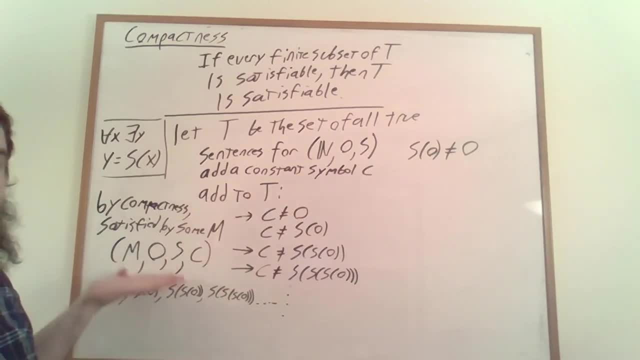 and so therefore has to be true of this structure as well. Additionally, we have an element C in this structure, And here's the thing: C is none of these elements here, None of these infinitely many elements. I guess, for succinctness, let's call these elements what they are: 0,, 1,, 2, 3, and so on and so forth. 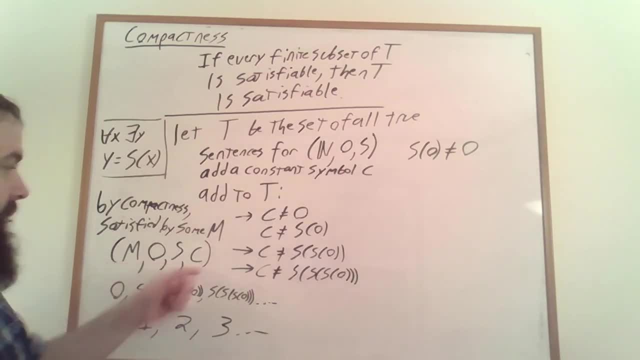 But then we also know that C is going to be an element of this structure and it's not going to be any one of these. So let's say that C is out here somewhere. Well, now we also have the successor of C. 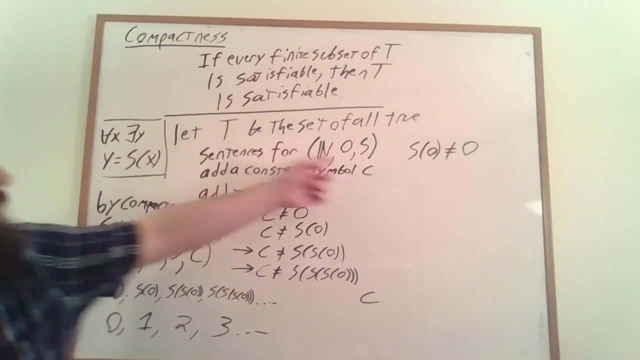 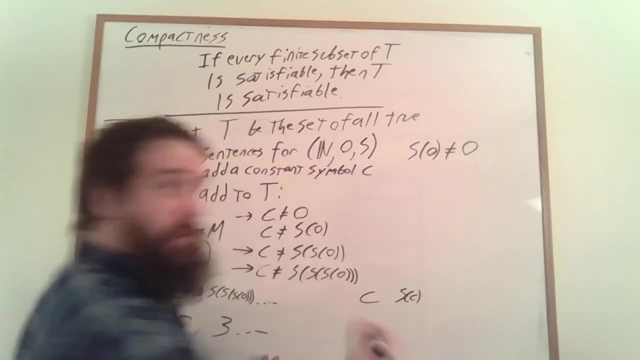 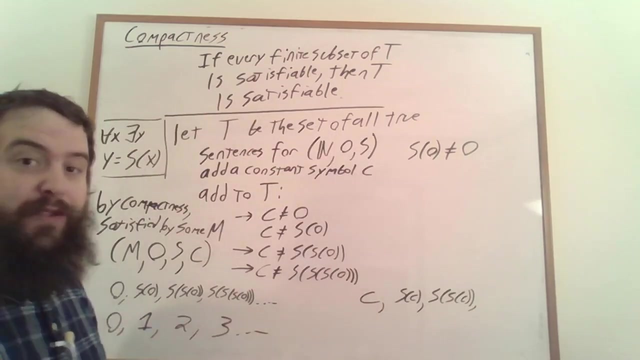 Again, this formula is true. It's true of this structure and therefore has to be true. It has to be true of this structure as well. And again we have the successor of the successor of C And the successor of that, and so on and so forth. 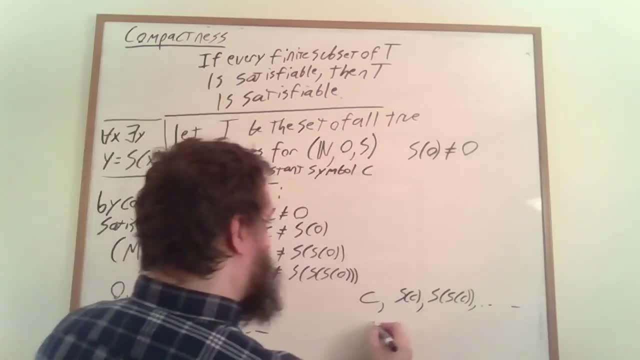 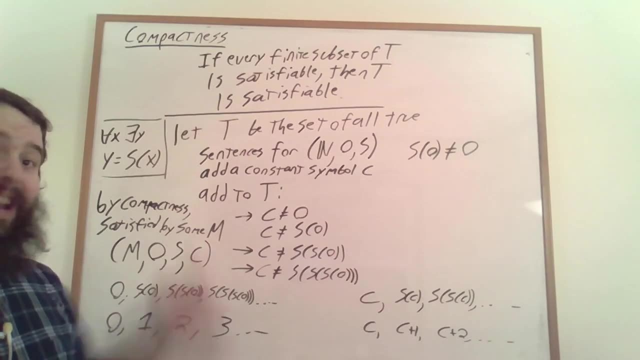 Let's call these elements what they are: This is C, this is C plus 1,, this is C plus 2, and so on and so forth. But now there's an additional property of this structure here that we need to take into account. 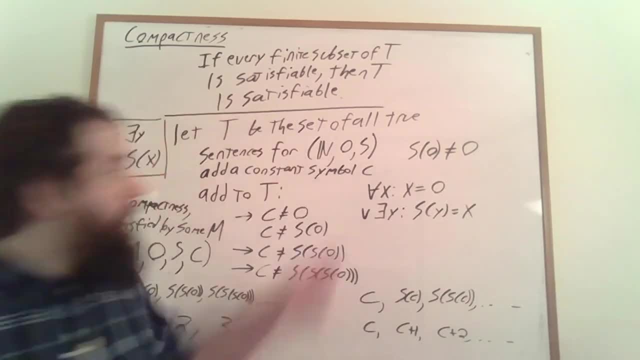 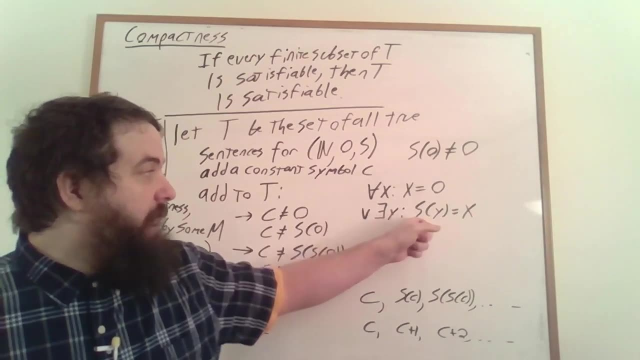 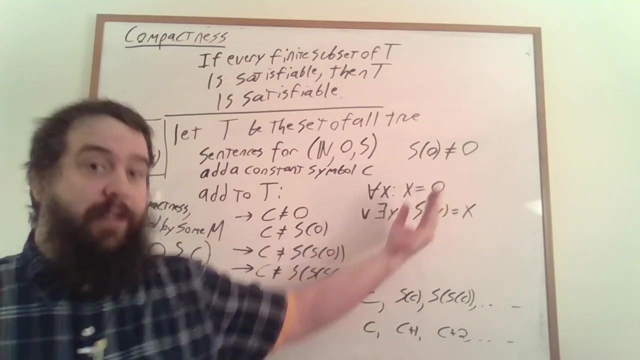 For any x, either x is equal to 0, or there exists a y, such that the successor of y is equal to x. So every element is either 0,, in which case it doesn't have a predecessor, or it does have a predecessor. 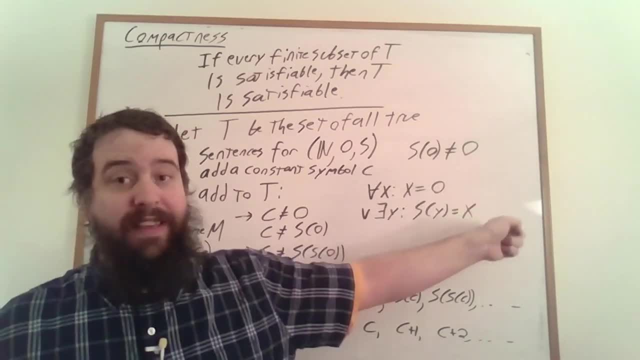 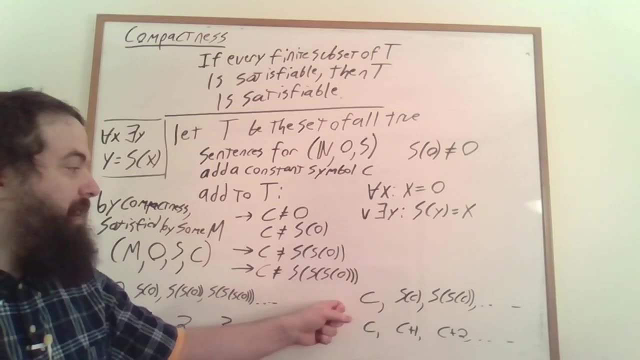 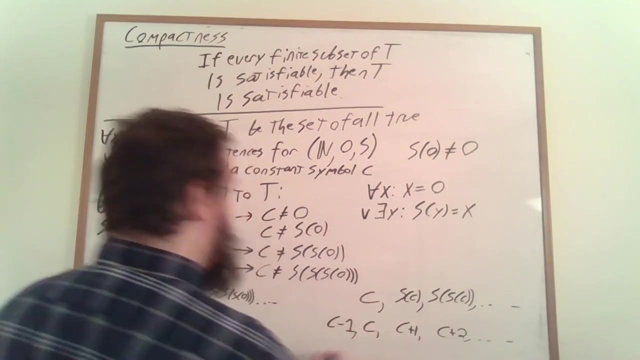 It has an element whose successor is x, has an element immediately before it, And so this requires us to add- Let's add in- an element that's immediately before C. Let's call that C minus 1.. And of course, that element also has to have an immediate predecessor. 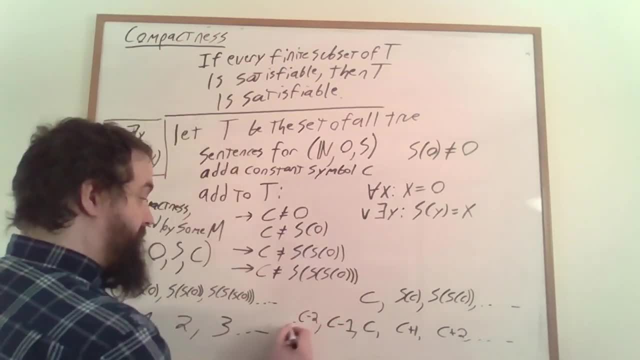 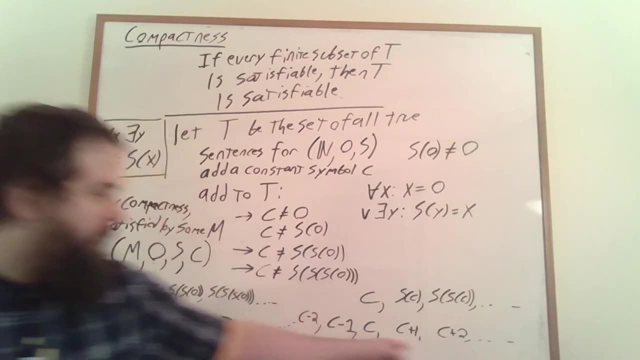 Let's call it C minus 2. And so on and so forth. Now here's the thing: At no point can any of these numbers be equal to a natural number, Because you could then do some tricky Proving and show that C then would have to be some natural number as well. 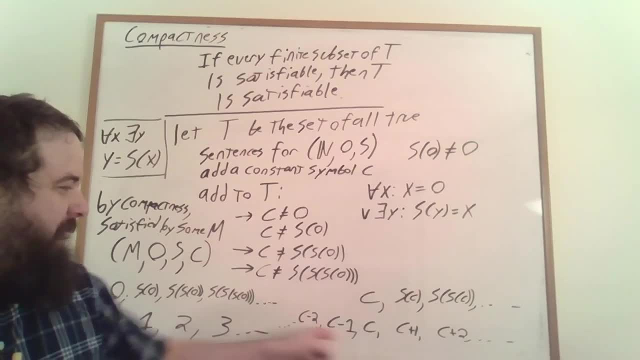 Right, If this number here was secretly 5, then this number here would be secretly 6, and this number here would be 7.. And we said that C was not equal to 7 within this list here. So all of these elements in our structure M that we're constructing have to be different from all of these elements here. 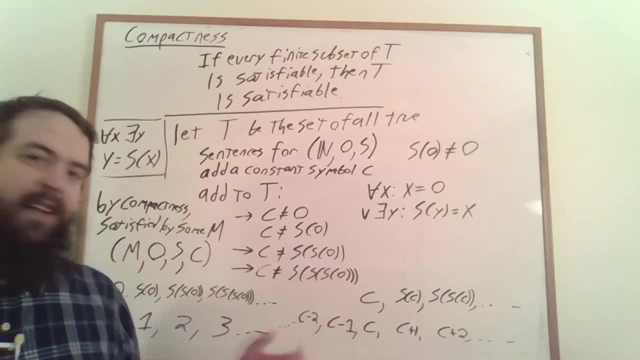 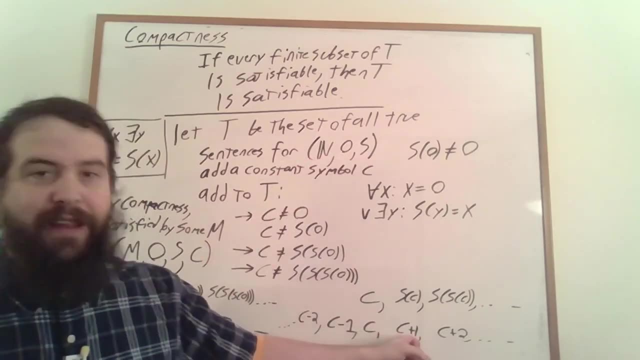 And they all have to be different from each other. Again, some sort of true fact About the natural numbers with 0 and successor, That every number is not equal to its successor, Is not equal to the successor of its successor, And so on and so forth. 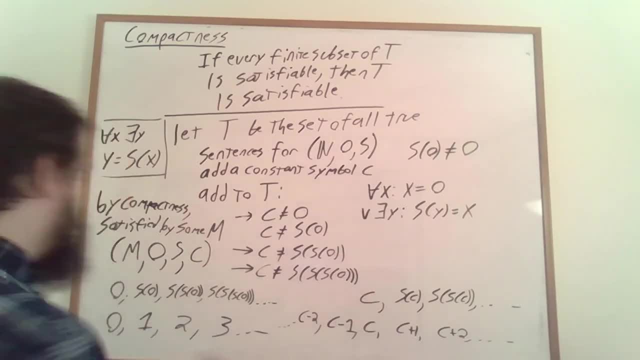 And it turns out we're actually done This structure here, This set of elements With 0 assigned to 0. The successor operation being what we intuitively think it should be. So for natural numbers, it takes us from one number to the next number in sequence. 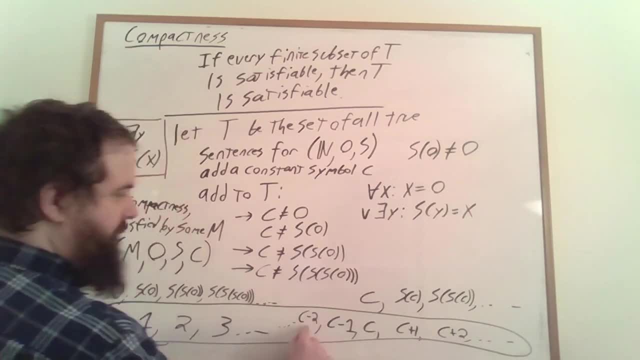 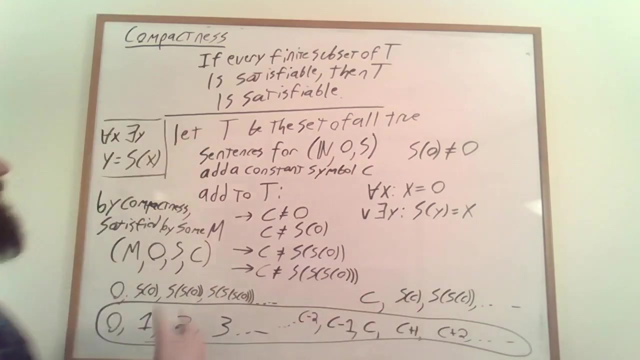 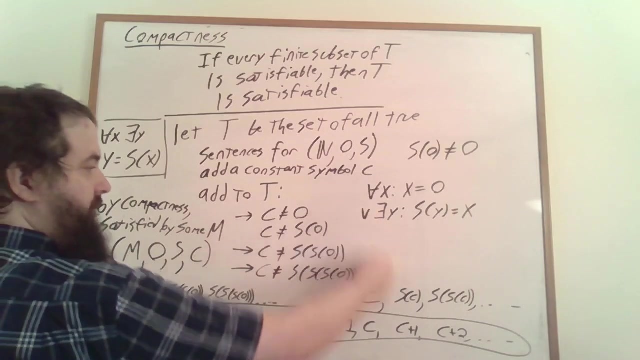 And then for these numbers it takes us from one element to the next in this list. And then C is a constant which is assigned to this particular element here, And together this structure here satisfies the set of all true sentences for this structure here And all of these sentences that we added to T here. 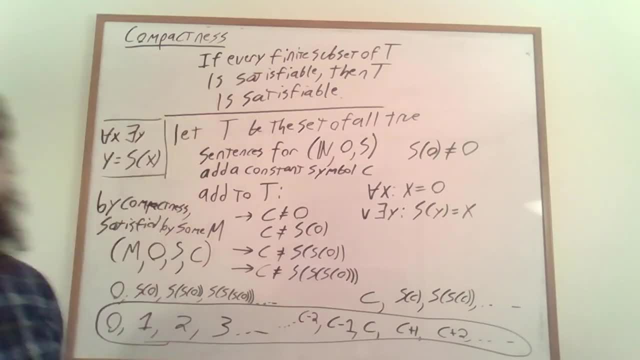 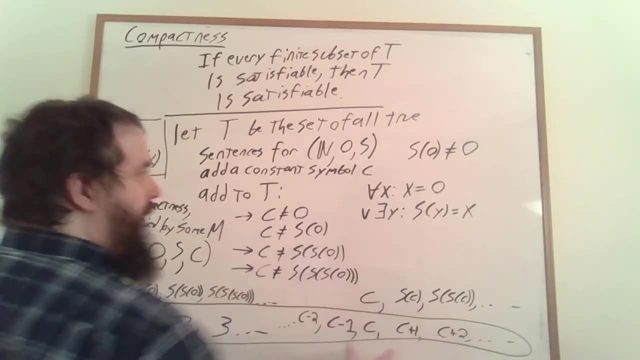 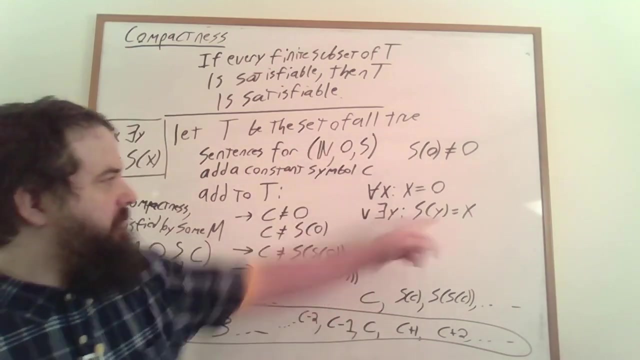 So this is the structure that the compactness theorem tells us exists. Of course, how do we actually know that we're done? How do we know that this structure here actually satisfies all of the true sentences for this structure here? We've only shown that it satisfies some of the basic true sentences of this structure here. 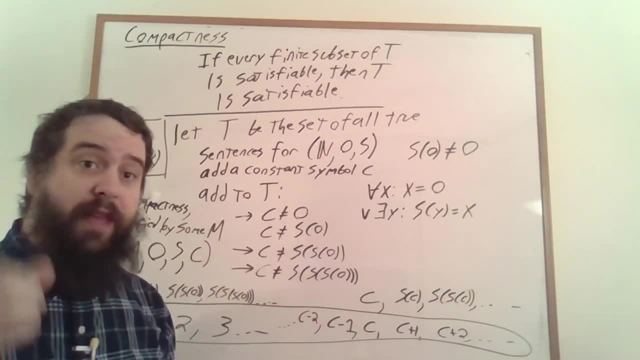 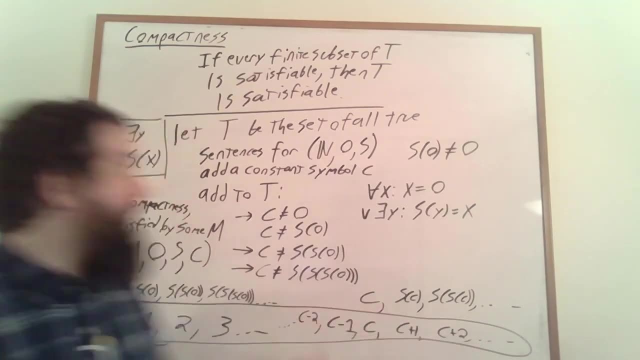 But how do we know that it satisfies all of them? Well, I'll explain that to you in the next video, But for now you're going to have to take my word that this structure does in fact satisfy the set of all true sentences for this structure here. 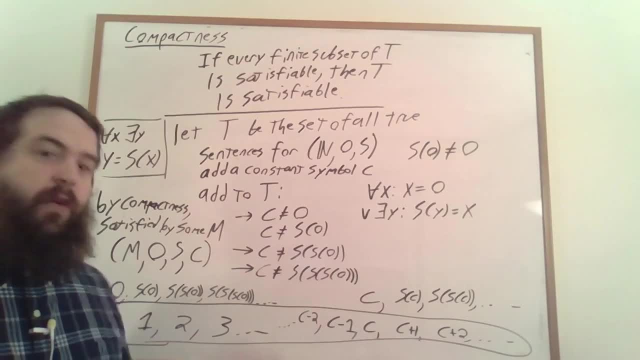 We don't have to add in anything else. So it turns out that this construction here actually can give you a little bit of an intuition for one of the proofs of the model existence theorem, This process of constructing our model by the model itself, Constructing our model by adding in things that we know have to be in the model. 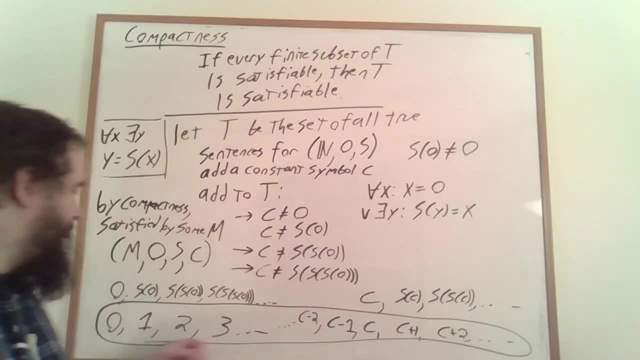 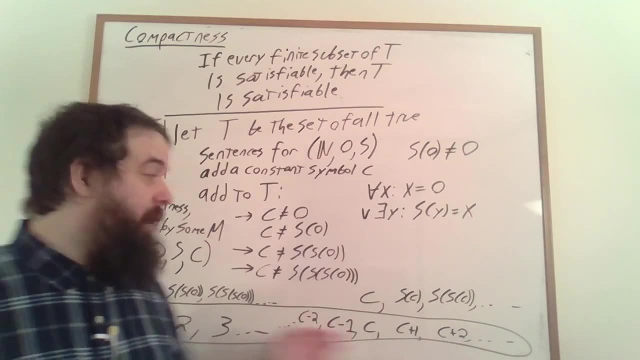 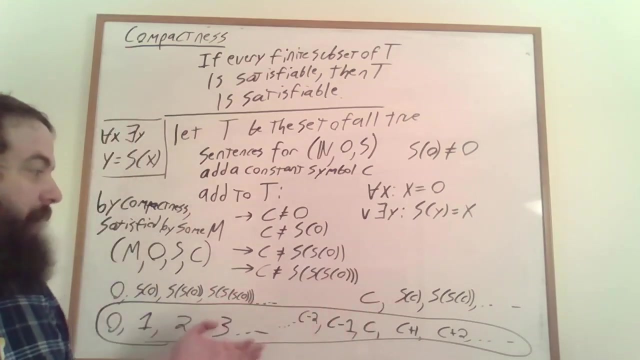 And then being careful about what things are equal to and not equal to other things in the model. And so if you add in all of the things that have to exist in the model and then are very, very careful, you wind up getting a structure that satisfies all of the sentences in your collection T. 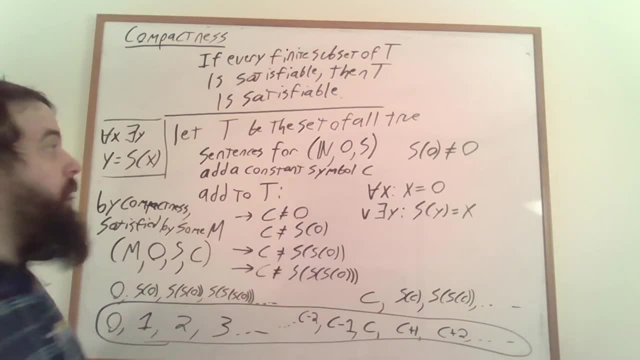 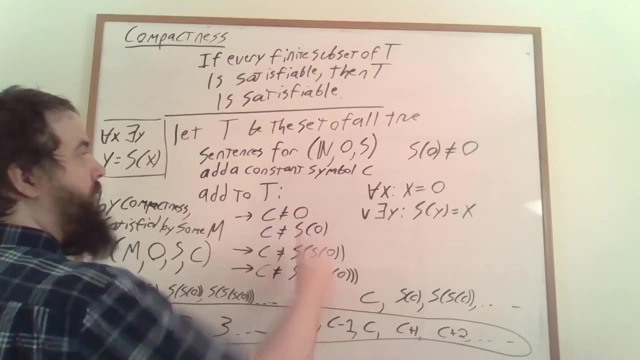 So let's take a moment to reflect on what we've done. We started out with a structure And we added a new constant symbol to that structure And we added a bunch of sentences to the theory of that structure specifying that this new constant symbol didn't represent any of the original elements of this structure. 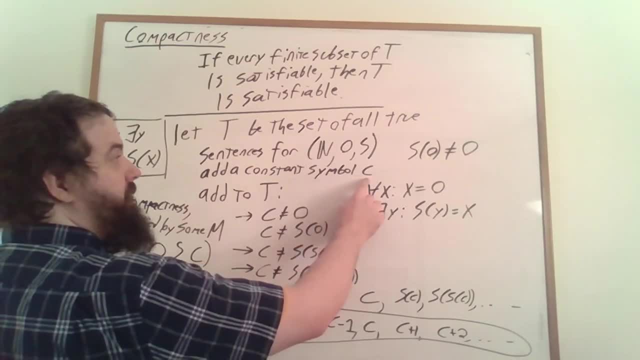 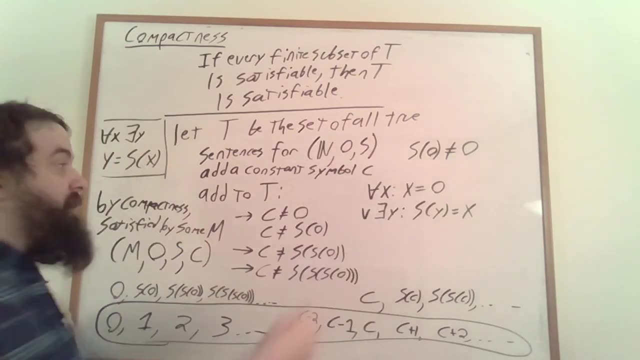 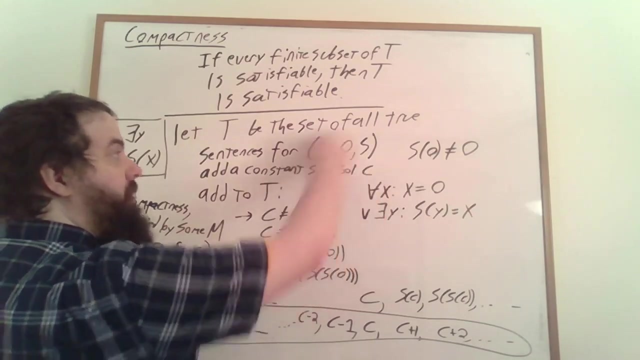 Of course that means that there's no assignment of that constant symbol for this original structure. that makes all of these sentences true, But if we only have a finite set of these sentences, then there is going to be an assignment of that constant symbol within this original structure. 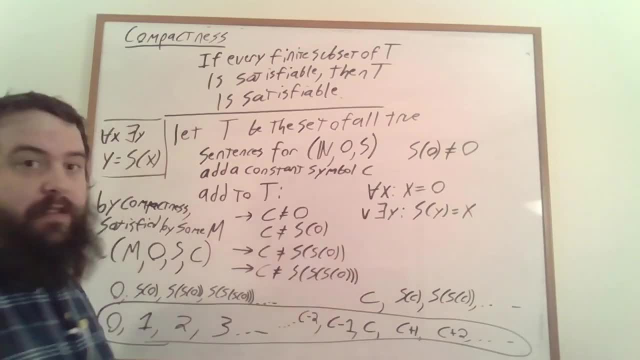 that makes that collection of sentences true. And so, by compactness, because every finite subset of T was satisfiable, there would be some other model that wound up satisfying our entire collection T, Some other model that had its own notion of C that wasn't equal to any of these things that we said it had to be unequal to. 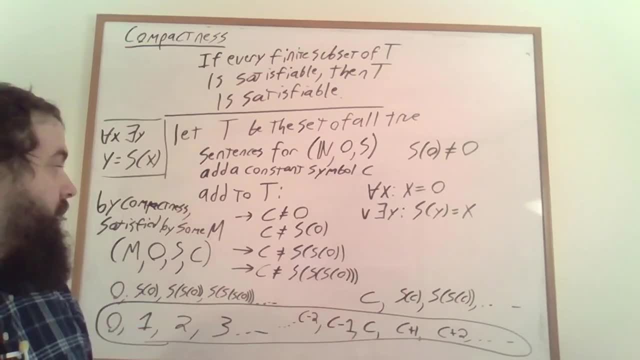 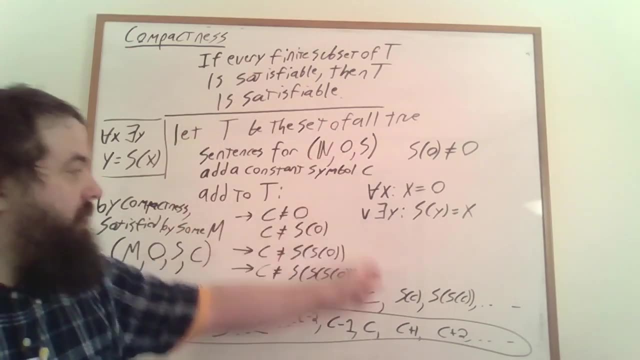 its own notion of C and this model satisfied all of the true sentences for this structure here and all of these sentences as well. Of course, in this model, as we can see, C is not 0,, 1,, 2,, 3, or any of the natural numbers. 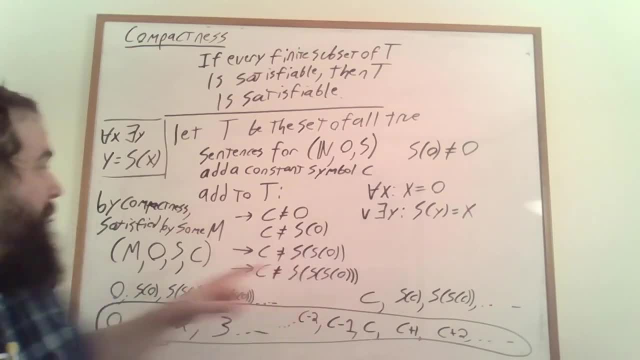 But notice what we did. We constructed a structure, a model that satisfied all of the true sentences for the natural numbers, with 0 and successor, Every first-order logical formula. that's true of this original structure by construction is also true of this other structure here. 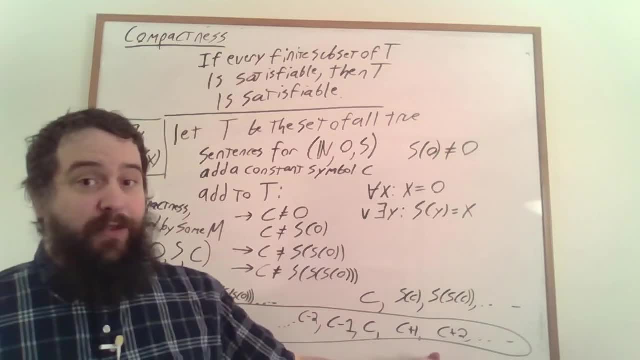 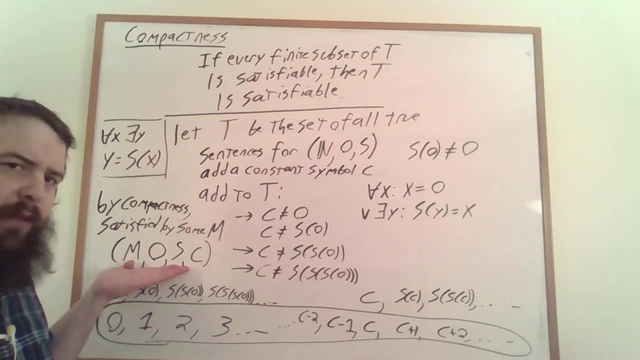 which is very clearly not the same structure. So we were able to create a structure that was- we use the term- elementarily equivalent. It's equivalent in terms of the set of first-order logical formulas, that it satisfies to the original structure, but it's a different structure. 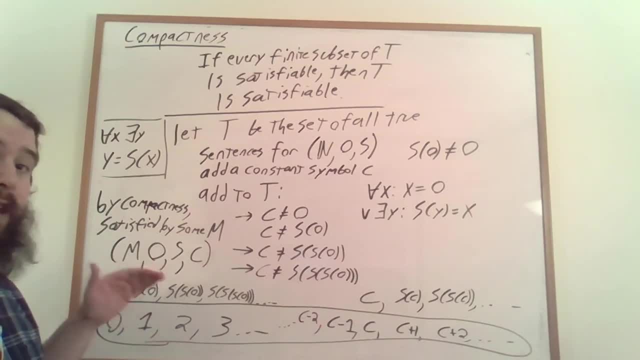 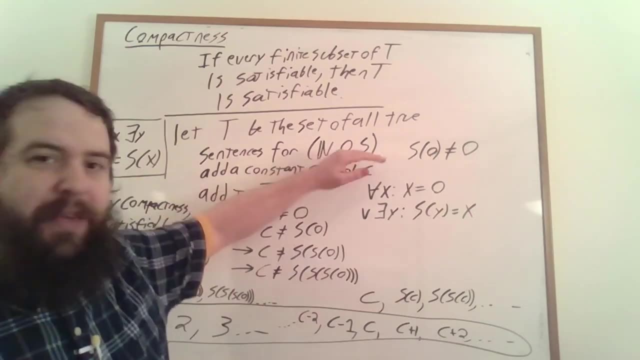 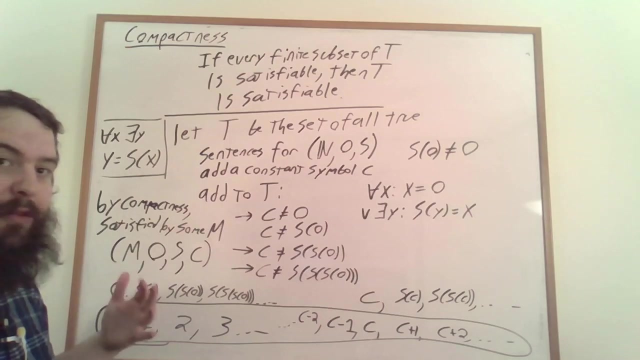 We also like to call these sorts of structures non-standard models. If there's some reason to believe that this is like the standard model, if there's something special about this structure, we like to call it the standard model. We like to call these structures that satisfy the same true formulas. 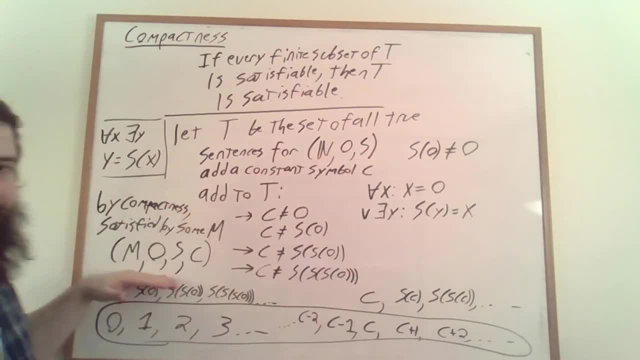 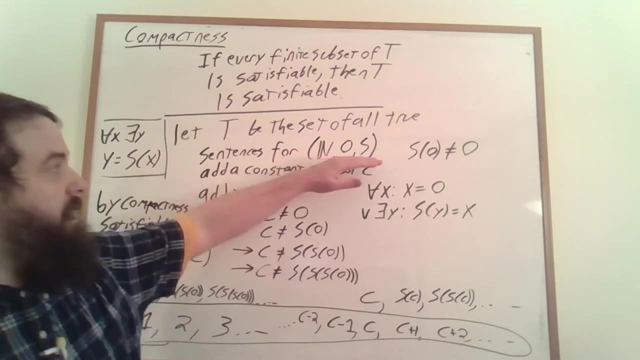 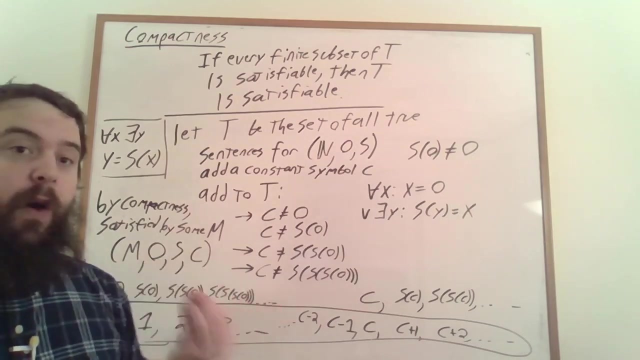 but aren't like the model. We like to call these non-standard models. One of the cool things that we can do with non-standard models is ask: how are they different from the original structure? How do these two structures which agree on whether all first-order logical formulas 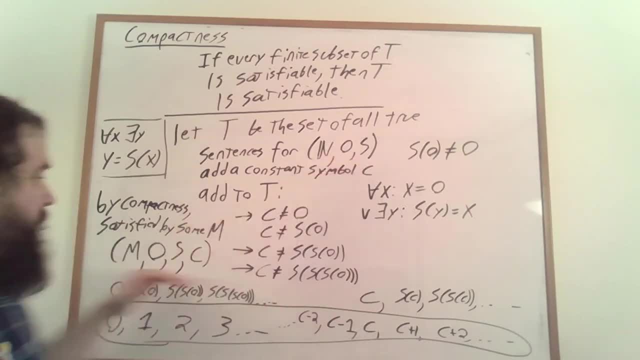 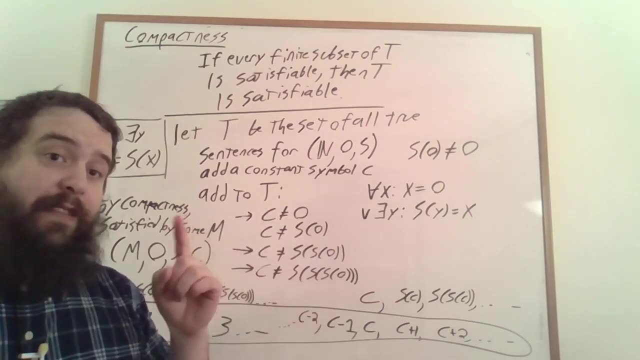 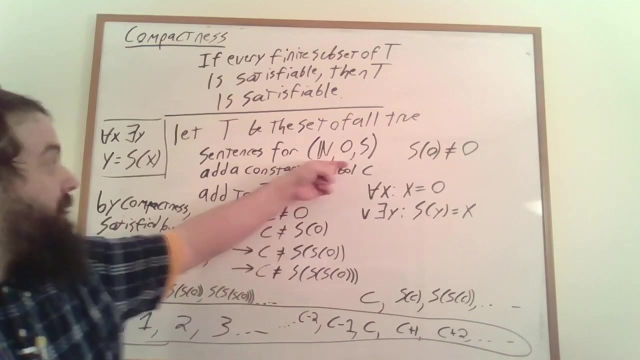 are true or false. how do these two structures, which agree, differ from each other? And the ways in which they differ necessarily are things that we can't express in first-order logic, Because if there was a difference between these two structures, that could be expressed in first-order logic. 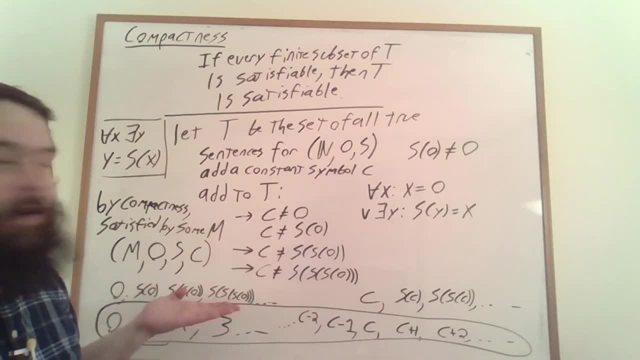 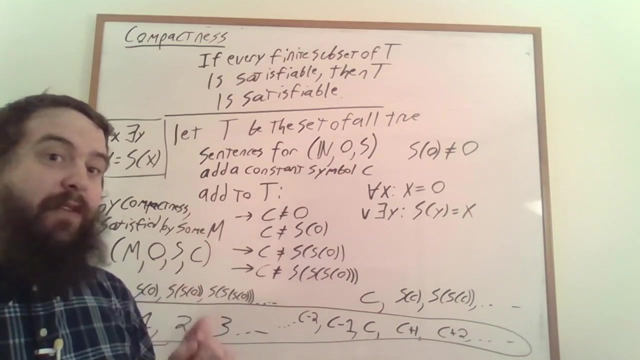 it would be a sentence that they disagreed on. But again, we said: all of the sentences that are true over here are true over here and vice versa. These two are logically indistinguishable in first-order logic, And so any difference that they have must be outside of first-order logic. 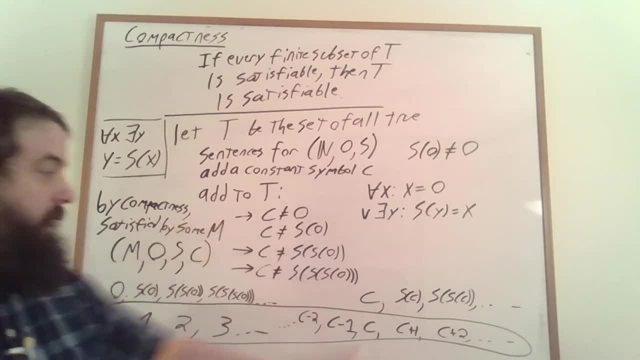 One of the key differences between these two structures is that this structure here has an infinite decreasing sequence of elements c, c-1,, c-2,, c-3, and so on and so forth, Whereas the natural numbers do not have an infinite decreasing sequence. 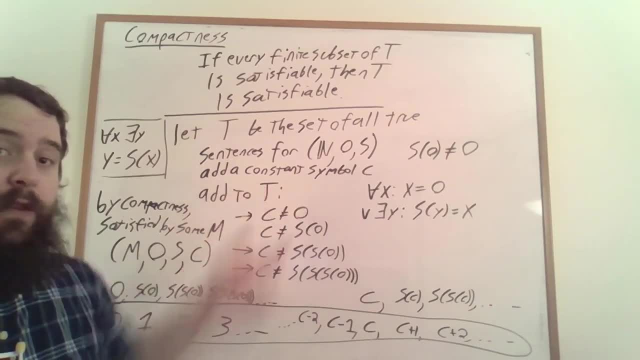 There is no infinite decreasing sequence of natural numbers. So this is a difference between these two structures. But remember, they agree on all first-order logical formulas And so that means that there is no first-order logical formula describing the existence of an infinite decreasing sequence. 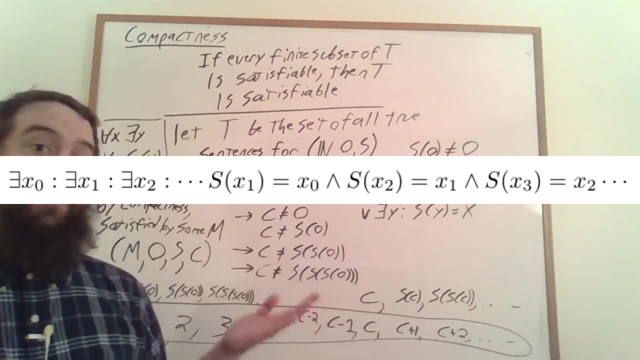 The naive way of expressing the existence of an infinite, decreasing sequence looks like this, And notice that it has an infinite number of quantifiers. Well, in first-order logic, we aren't allowed to have an infinite formula, So going about it the naive way. 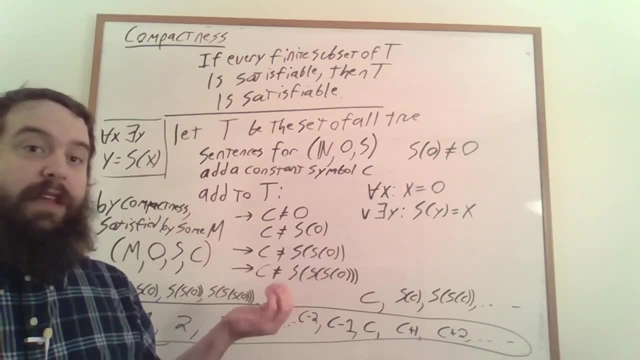 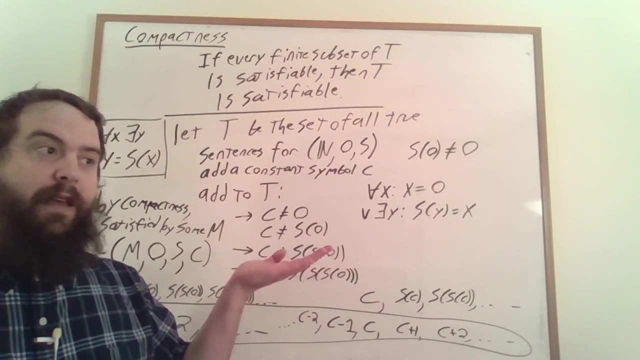 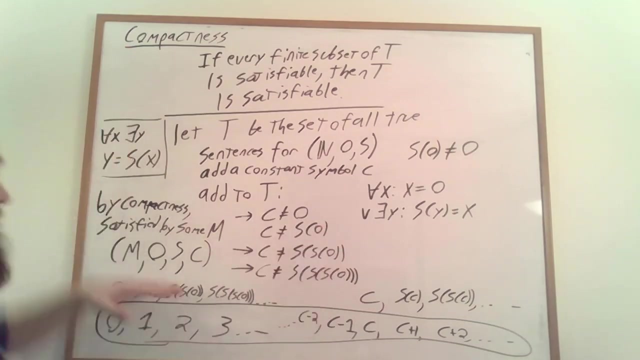 we can't express the existence of an infinite decreasing sequence in first-order logic. But maybe there's a clever way of expressing the existence of an infinite decreasing sequence in first-order logic. But then we would have a difference, a first-order logical difference. 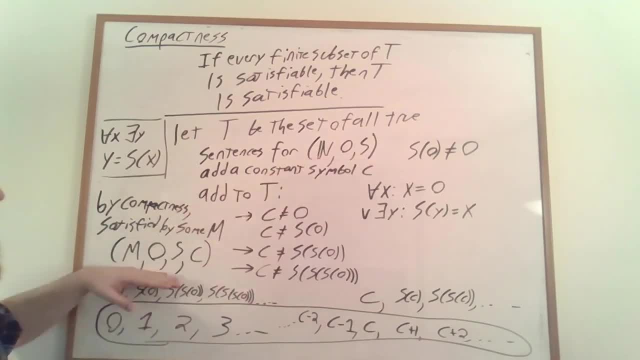 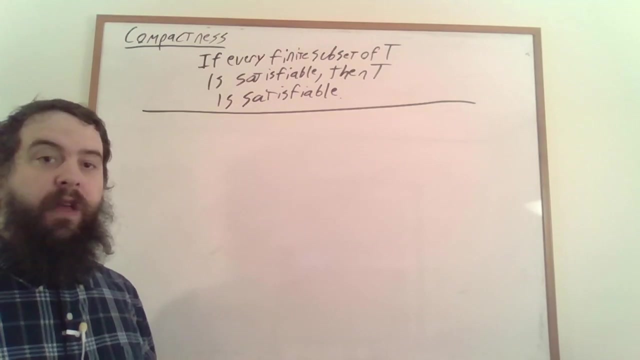 between this structure and this structure, We'd have this formula being true here and false here, And that's something that we can't have, Because these two structures are identical in terms of the set of sentences that they satisfy, While there are more advanced applications of the compactness theorem. 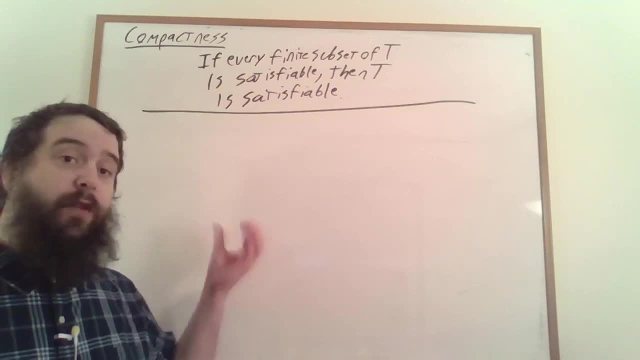 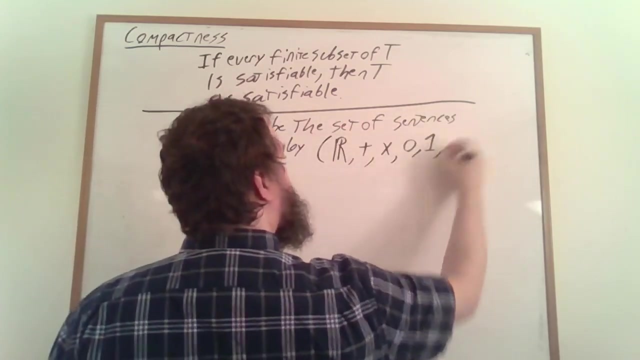 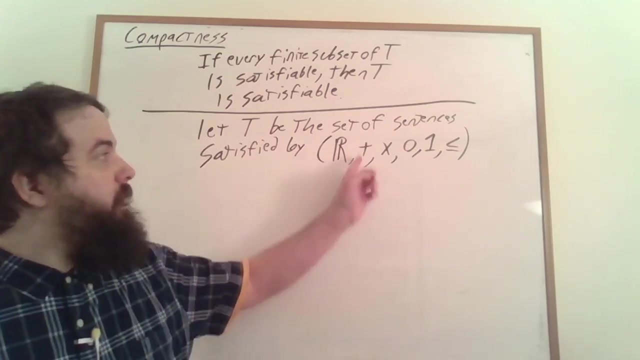 we can actually go incredibly far just by adding a new constant symbol and specifying a collection, an infinite collection of sentences that that new constant symbol has to satisfy. Let's let t be the set of all sentences satisfied by the real numbers with addition, multiplication, 0,, 1, and less than. 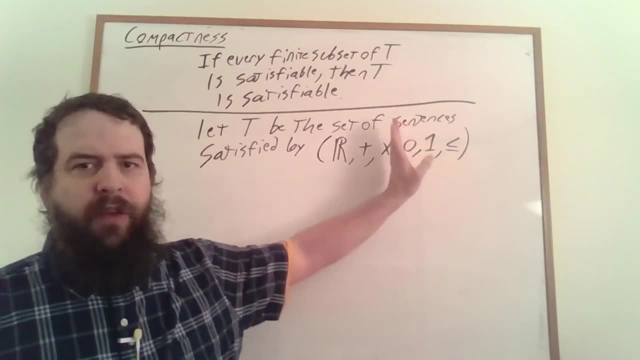 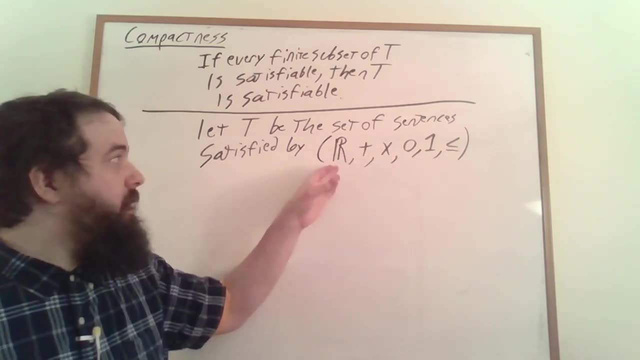 And it's worth noting, 0,, 1, and less than are redundant because they're all definable in terms of addition and multiplication within this structure. So really we could just be looking at the real numbers with addition and multiplication or the ring structure of the real numbers. 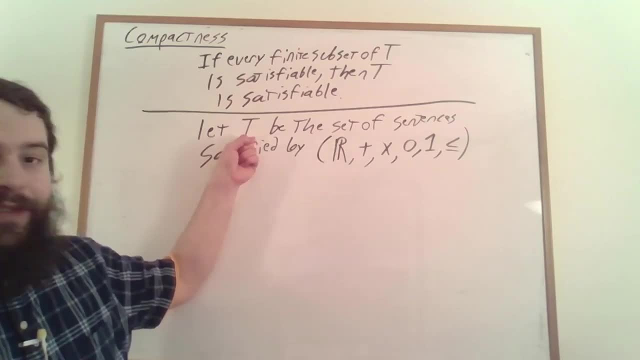 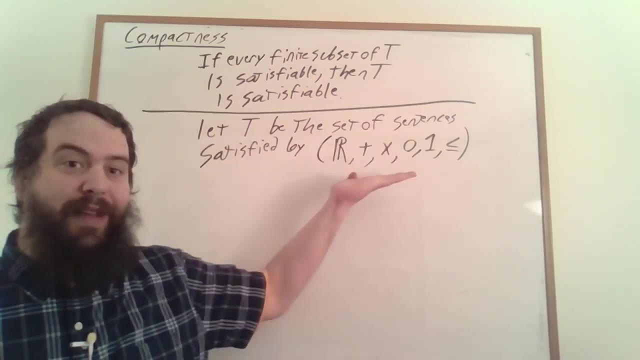 Again, this collection here, every finite subset of this collection, is satisfied by this structure here, because it's the set of all sentences that are satisfied by this structure here. It is the theory of this structure. So let's add in a new constant symbol. 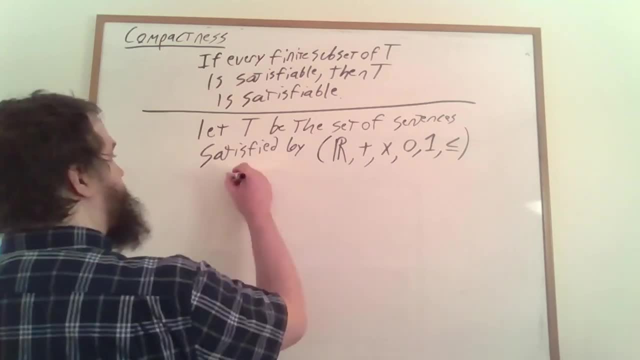 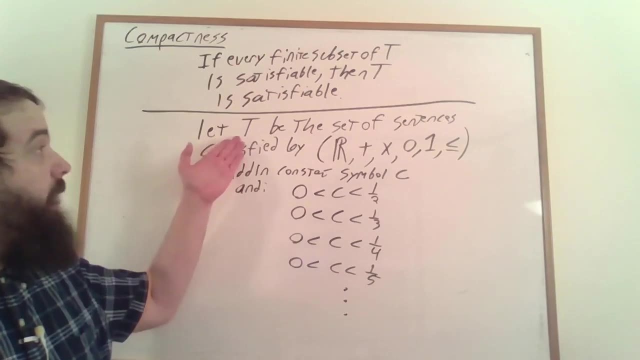 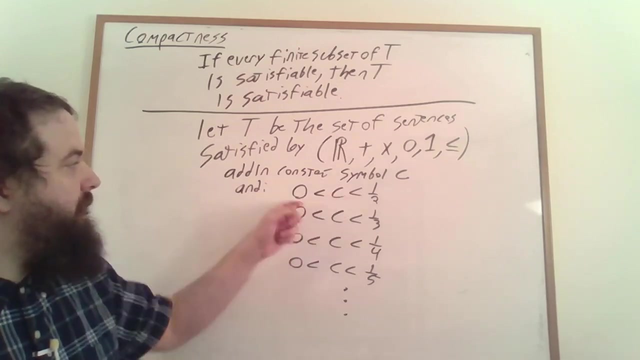 and an infinite collection of sentences to be satisfied. So to this collection t we're going to add in this infinite collection of sentences of the form c is strictly between 0 and 1 over n for various values of n, Any finite subset of this collection here. 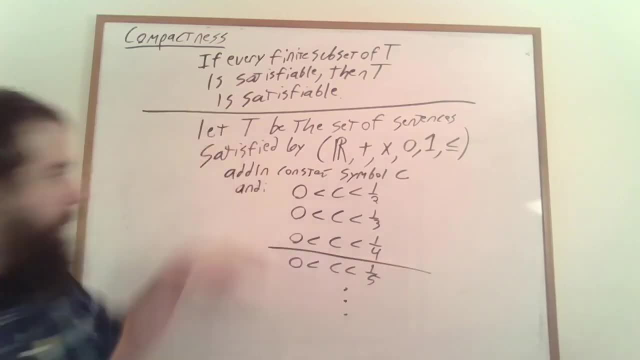 is going to cut off at some point where all of the sentences that are in our finite collection are above the line and there's nothing below the line in our finite collection. So if we have a finite subset of t, it's going to consist of: 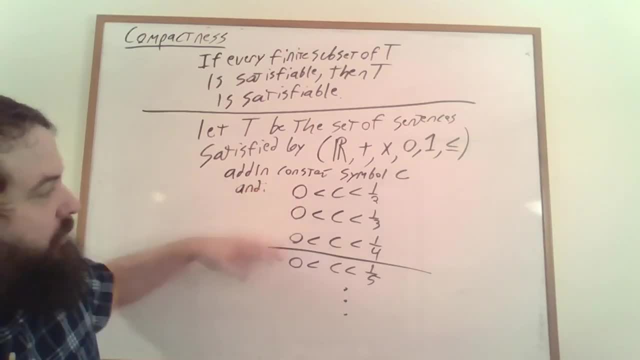 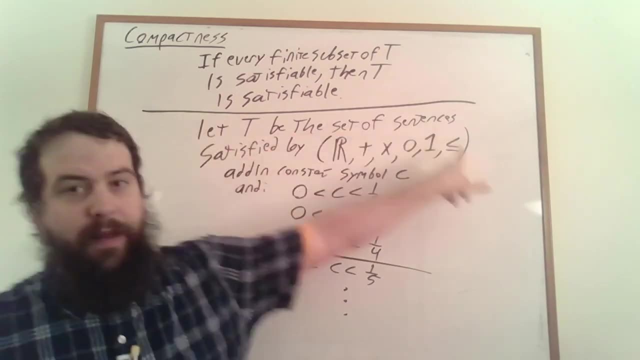 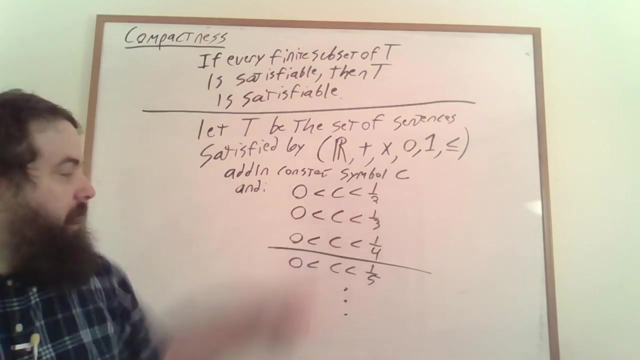 some finite collection of sentences from above the line here and some finite set of sentences that are just by default satisfied by this structure here, And so together they're going to be satisfied by this structure here, with c being equal to some appropriately small number. 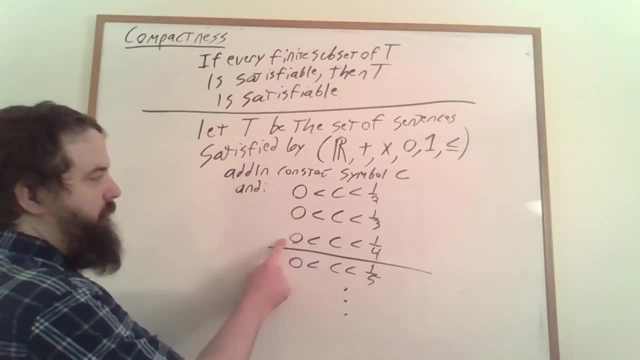 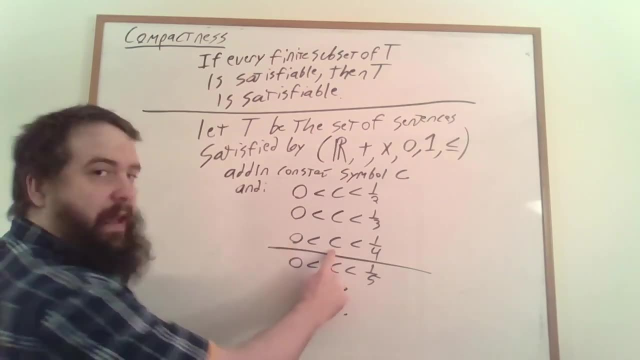 Right, if we just have to satisfy all of these formulas here or some subset of these formulas here up to this point, but nothing afterwards. we can just pick a c that's between 0 and 1. fourth, So we have a special constant c. 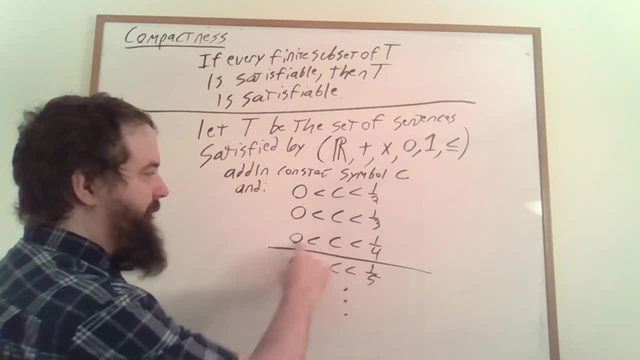 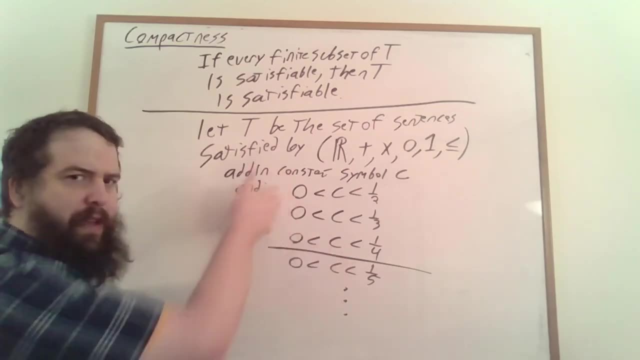 representing, let's say, the number 1, fifth or something like that, and that's going to satisfy all of these formulas here and therefore whatever finite subset of these formulas we wind up picking, And so any finite subset of this new collection that has both the theory of this structure. 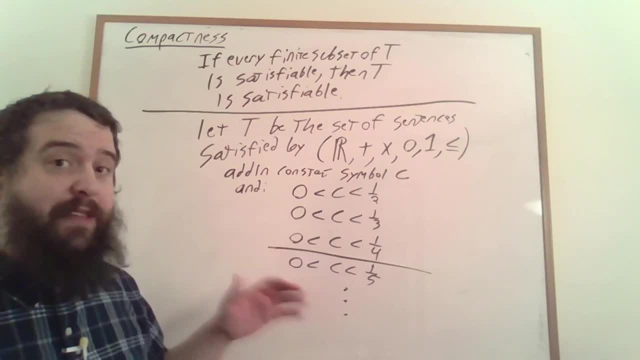 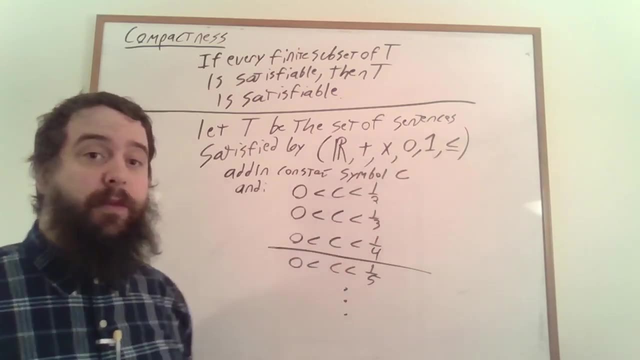 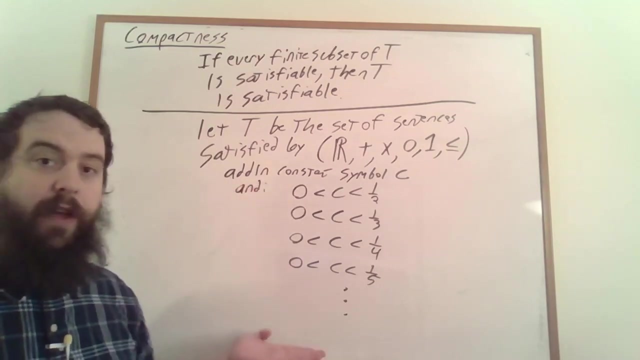 and this infinite collection of formulas. any finite subset is going to be satisfiable by this structure, here with an appropriate assignment to the constant symbol c. On the other hand, if we have the infinite collection, well, there is no assignment to the variable c. 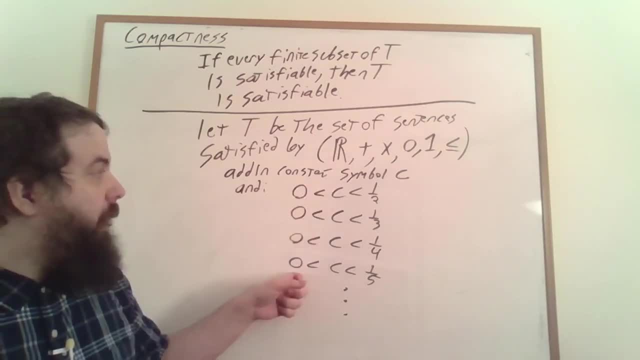 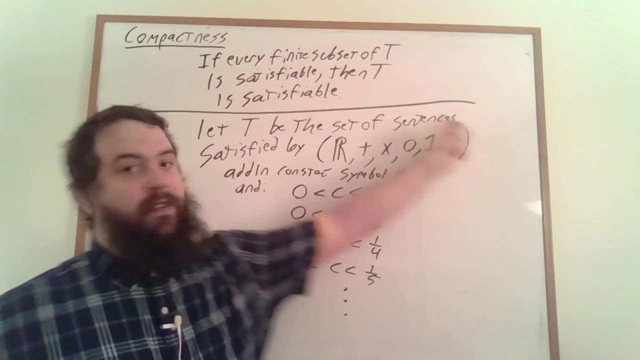 that's going to be strictly greater than 0, but also strictly less than 1 over n for every possible n. There's no way within this structure to assign the constant symbol c to make all of these true. But again, the compactness theorem. 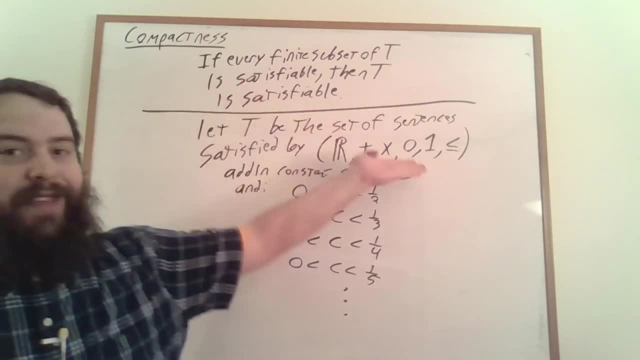 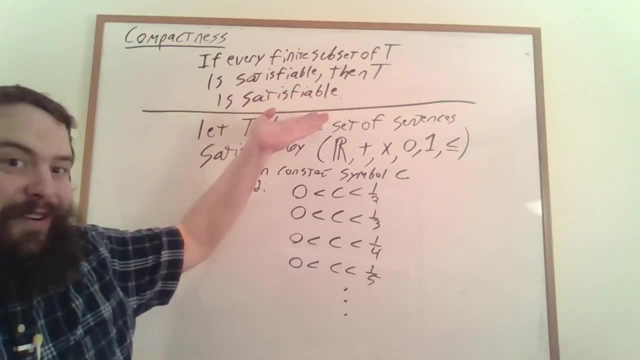 doesn't say: oh, it's satisfiable by the same structure. The compactness theorem says that this collection is satisfiable by some structure, and so what it's going to do is it's going to give us a new structure, a new model, m. 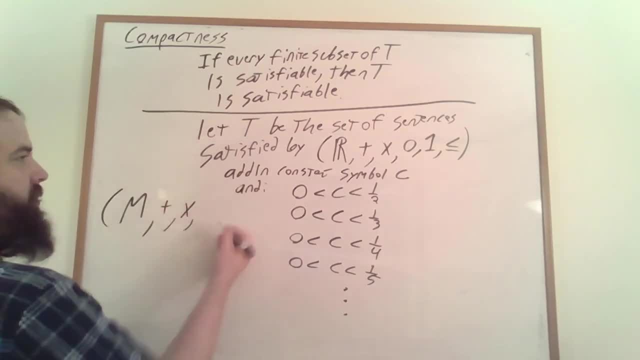 with its own notion of addition, its own notion of multiplication, its own notion of 0 and 1 and its own notion of less than, and it's going to also have a notion of the constant symbol c, some assignment of that constant symbol. 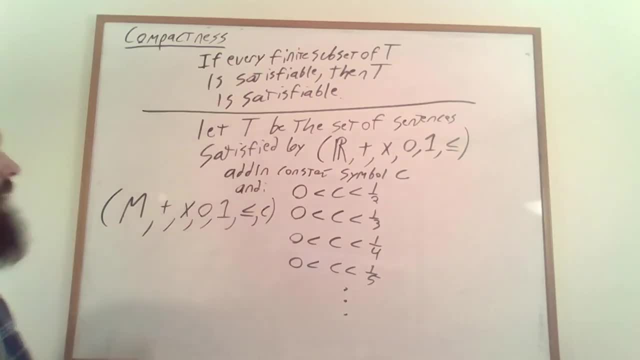 some interpretation of that symbol, satisfying all of the true sentences of this structure here, but also all of these sentences here. So what this structure is going to look like, it's going to look a lot like the real numbers It's going to satisfy. 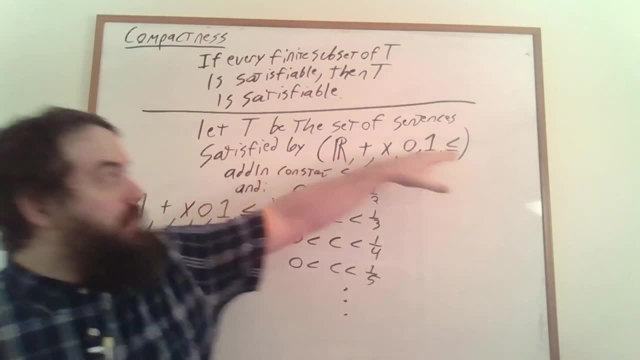 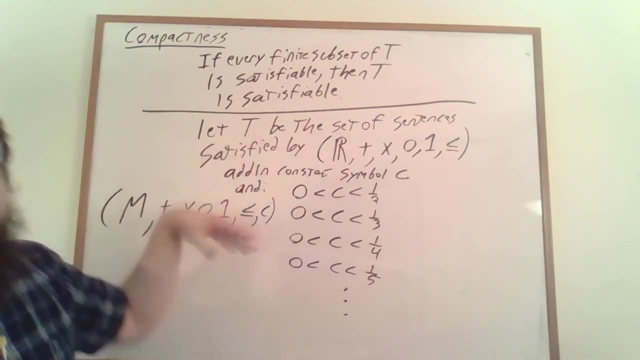 all of the same first-order logical formulas as this structure here. right, That's part of the construction. is that t? the set of formulas that we need m to satisfy is going to include all of the true sentences satisfied by this structure here? 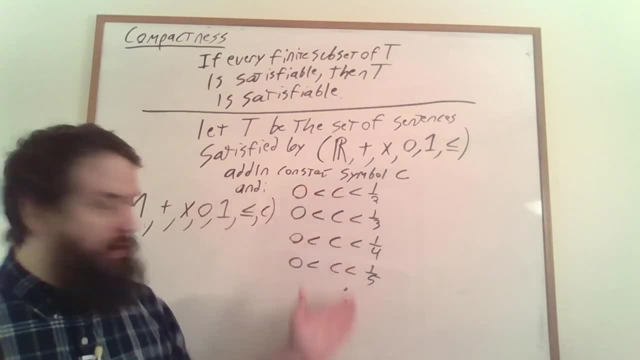 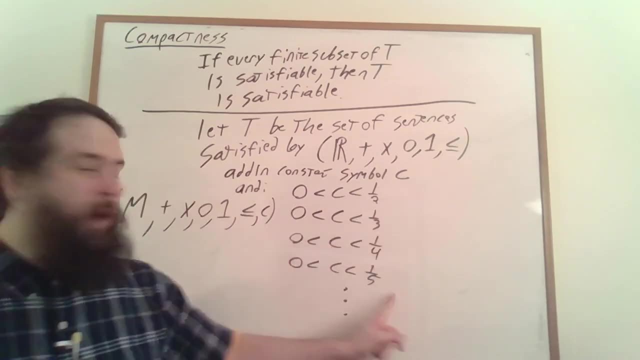 But additionally m is required to satisfy all of these formulas here, And so therefore m is going to have an element that's less than all of the 1 over n's, but strictly greater than 0. m is going to call that element c. 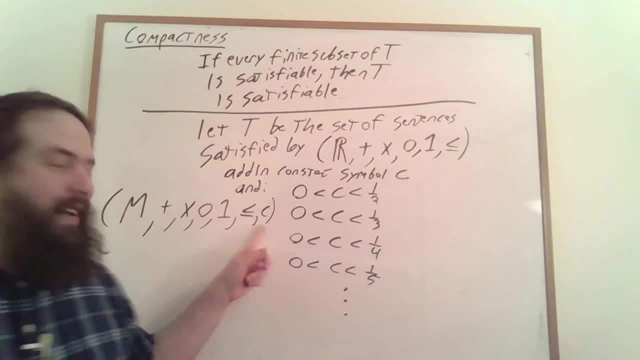 or usually we like to call this element epsilon. This structure is going to be a non-standard model of the real numbers. It's going to contain an infinitesimal element. It's going to contain what we intuitively think of when we talk about things like: 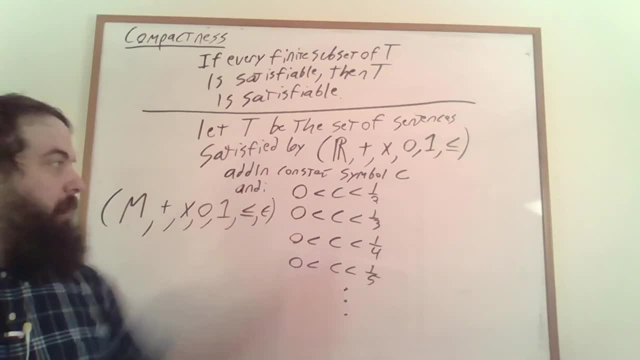 dx in calculus, some number that's infinitely small. And, of course, because we can divide by any number that isn't 0, we can take 1 divided by that element and get a number that's infinitely large. that also has to be in this structure. 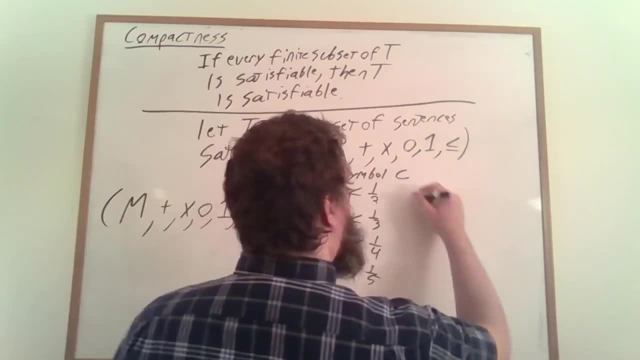 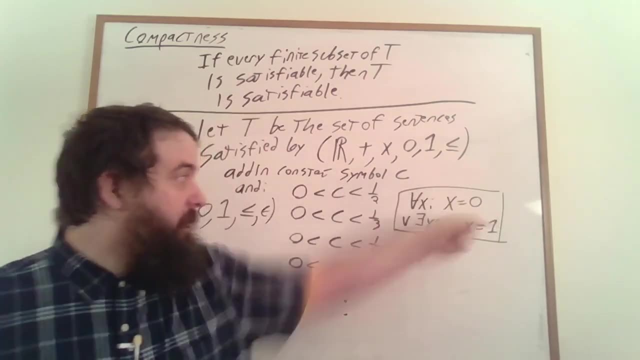 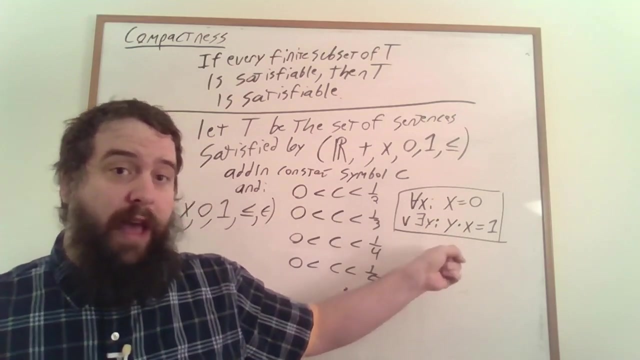 because in this structure, this sentence here is true For any x, x is either equal to 0 or there exists a y which, when multiplied by x, gives us 1.. We usually call that y, 1 over x, And so 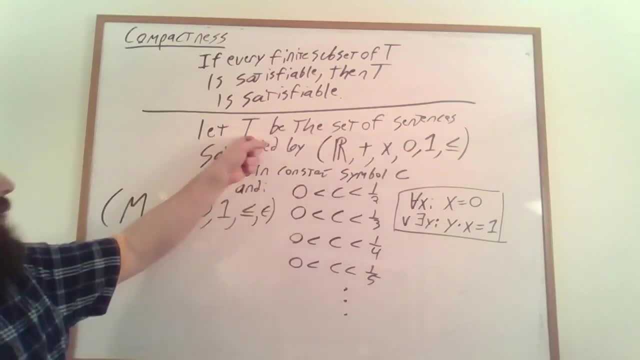 because this is true of this structure. it's true, it's an element of t. This sentence here is an element of t, And this structure here has to satisfy all of the formulas in t, And so it's going to satisfy this formula as well. 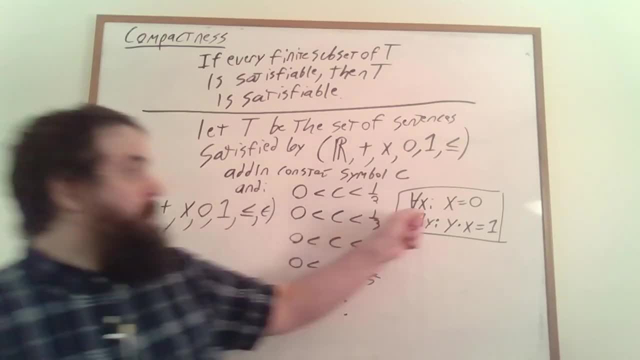 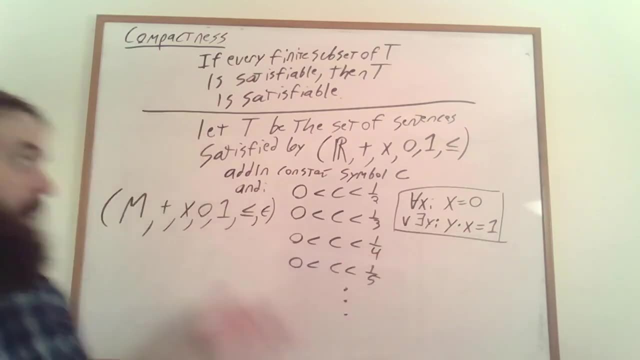 It needs to be the case that within m for every element, x. that's not equal to 0, there's going to be some y, such that y times that x is equal to 1.. There's going to be a 1 over every element here. 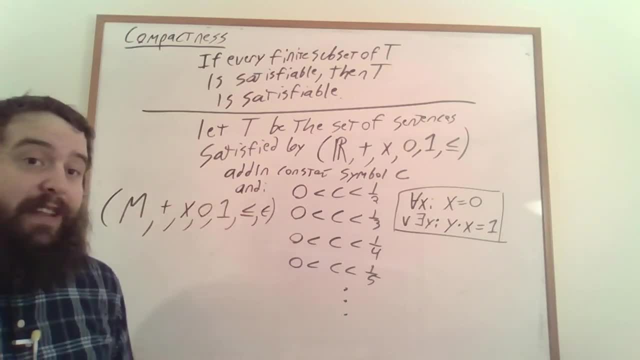 So there's going to be a 1 over epsilon, an infinitely large element, And you can actually prove that that element has to be infinitely large. It has to be larger than 1 and 2 and 3 and 4 and 5 and so on and so forth. 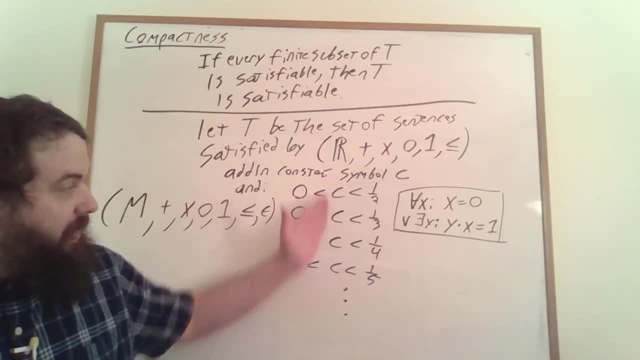 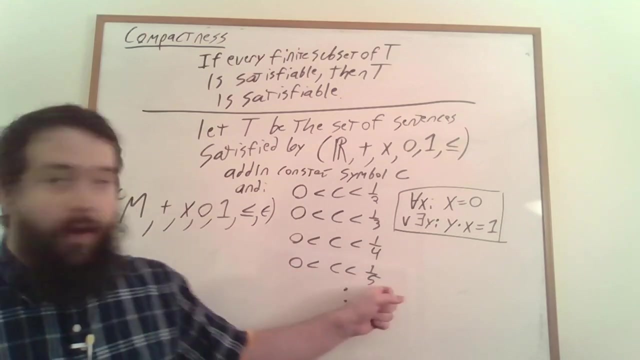 simply by taking these facts that we said about c, which we decided to call epsilon, and flipping them around. And the fact that you can flip these facts around, the fact that if c is between 0 and 1, fifth, then we know that 1 over c. 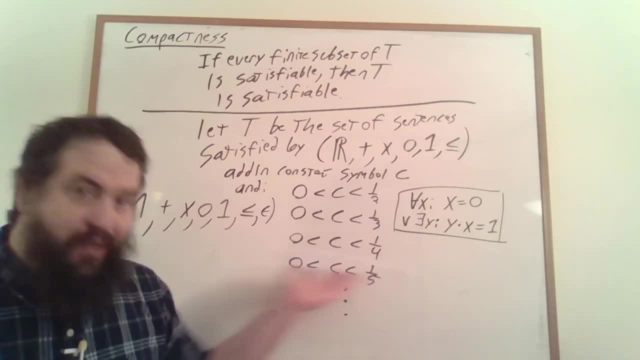 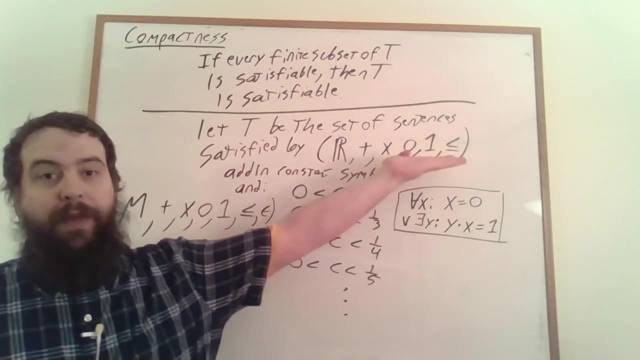 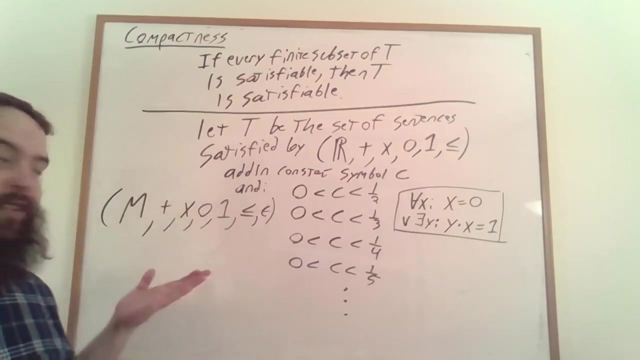 is larger than 5, we can do that flipping around, because that flipping around property is actually a first-order property, a property that we can express in the first-order logic of this structure here. So, in some very formal way, we have some structure. 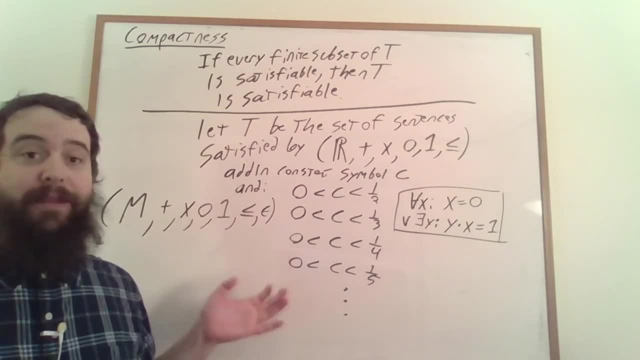 that has infinitesimal and infinite elements in it but otherwise behaves a lot like the real numbers. This forms the foundation of a field of study called non-standard analysis, And non-standard analysis was used to provide a concrete formal foundation to the intuitive practice of using infinitesimals within calculus. 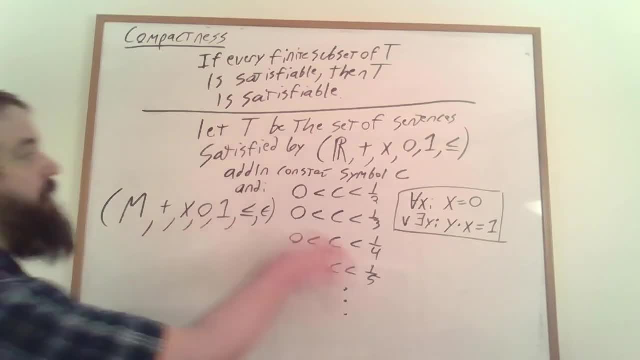 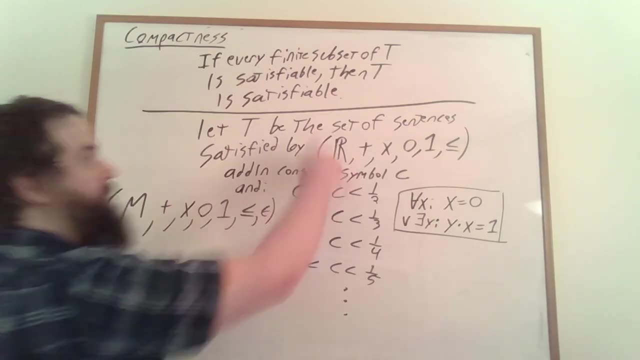 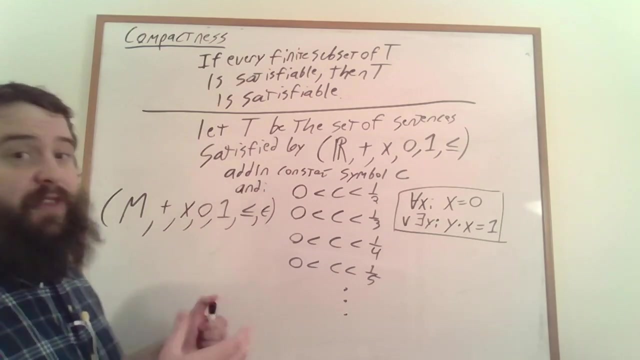 Interestingly, we can actually find an m satisfying all of these formulas here. that is countably infinite. In some sense. there's a bunch of elements of the real numbers that we don't need from the perspective of first-order logic, specifically a bunch of transcendental elements. 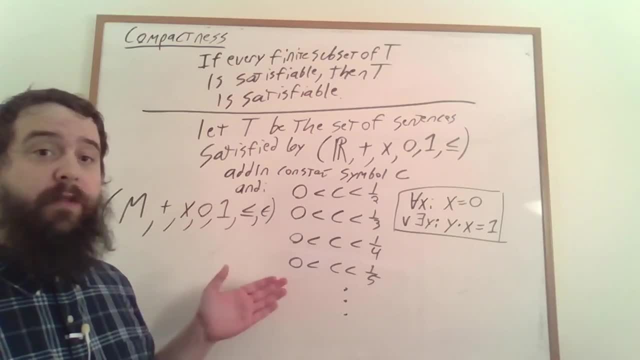 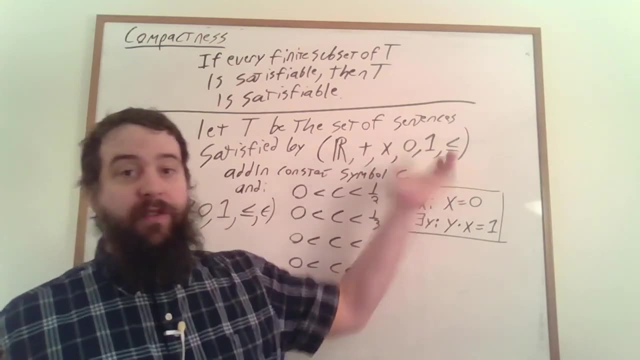 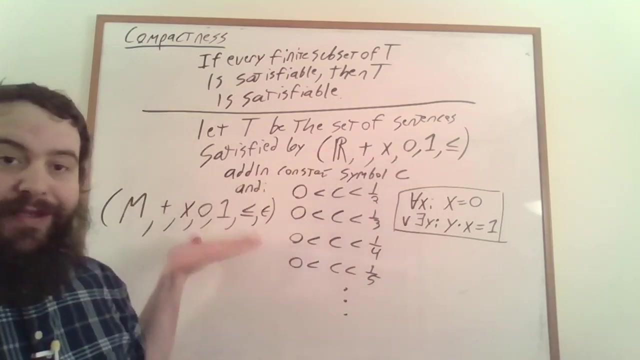 We can use this exact sort of process to produce non-standard models of all sorts of structures, models that satisfy all of the same set of sentences, all of the same first-order logical sentences, but aren't the same. They aren't the same structure. 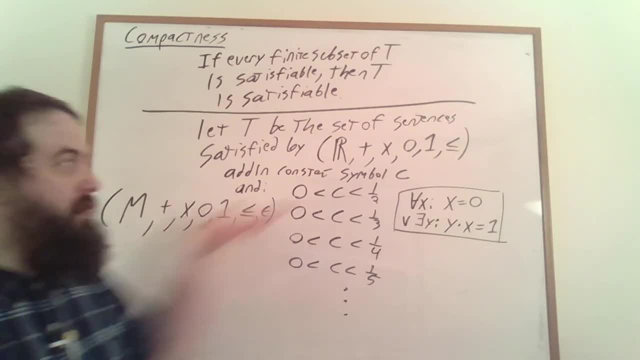 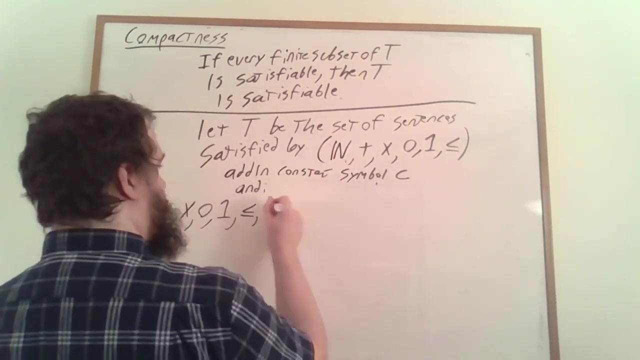 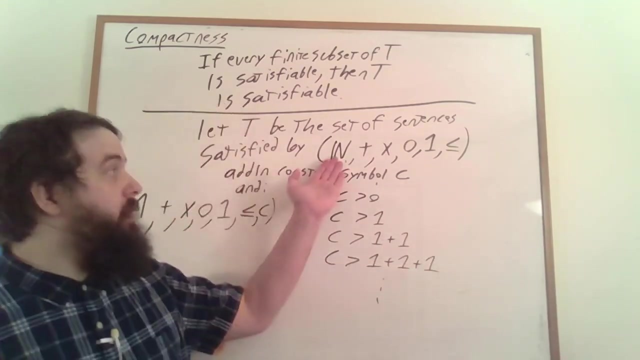 They're not isomorphic to each other. There's no way of going from one structure to another, because they differ in a very fundamental way. This one has infinitesimal elements and this one does not. Similarly, we can construct a non-standard model of the natural numbers. 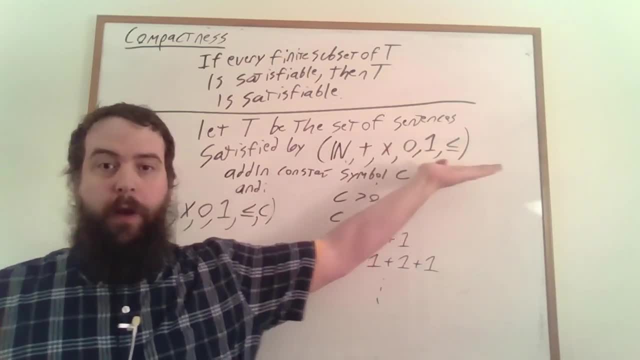 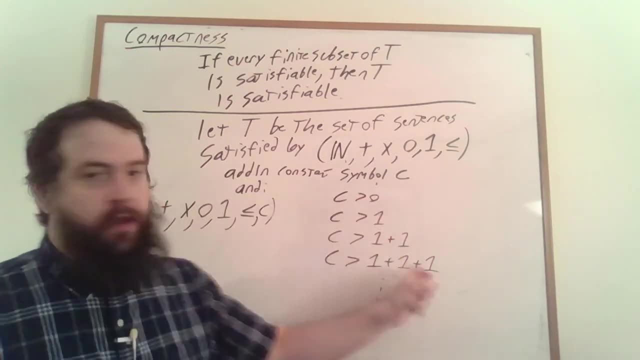 with all of the structure we could possibly want, with our infinite element c, which is greater than 0 and greater than 1, and greater than 2 and greater than 3, and so on and so forth. This set of sentences here, the theory of this structure. 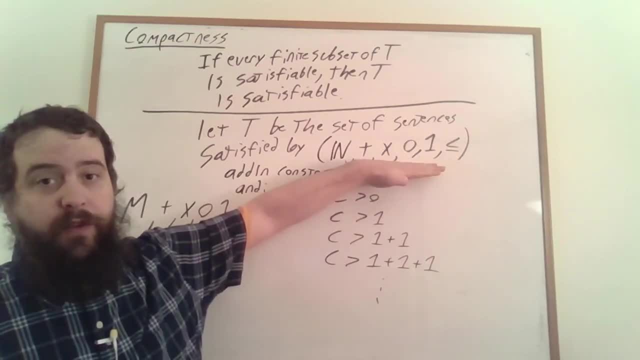 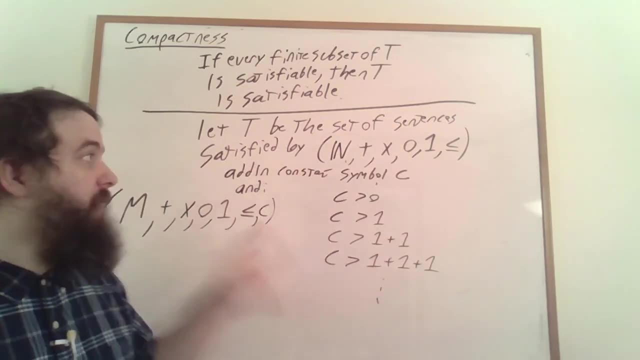 the set of all true sentences of this original structure here, along with this infinite collection of sentences here. any finite subset of that is going to be satisfied by this structure here with an appropriately large assignment of the value c And so therefore by compactness. 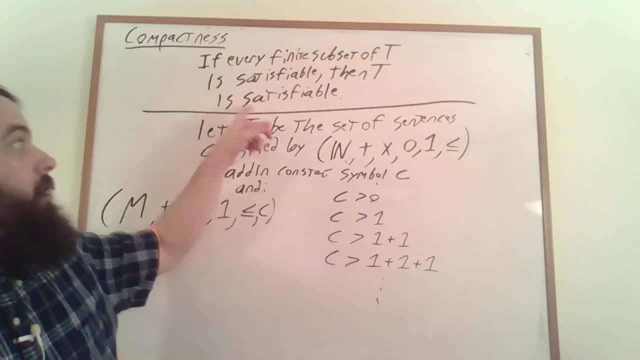 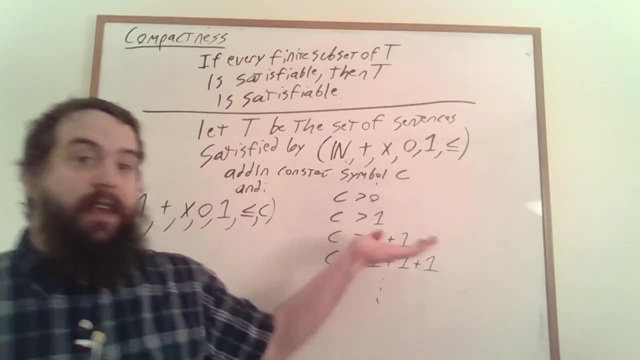 the entire collection is satisfiable by some model, But it's not going to be this model with a particular assignment of the value of c. It's going to be some other model where c is required to be some infinite element, And so we've gone beyond. 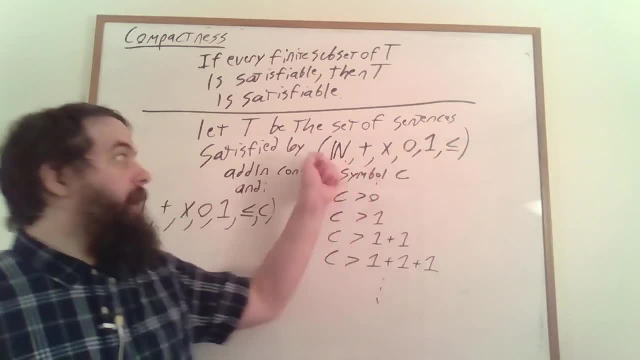 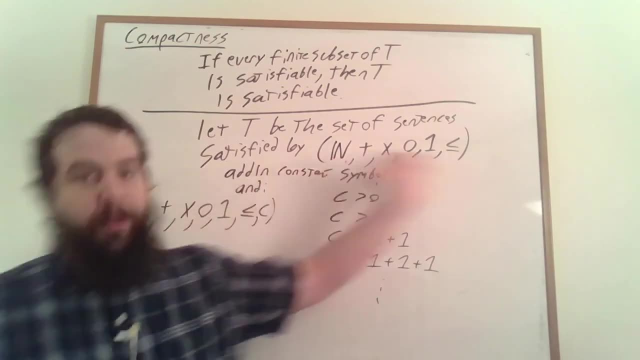 just showing that there's a non-standard model of the natural numbers with a notion of successor. We've shown that there's a non-standard model of the natural numbers with a whole bunch of things, That there's some structure which is different from this structure. 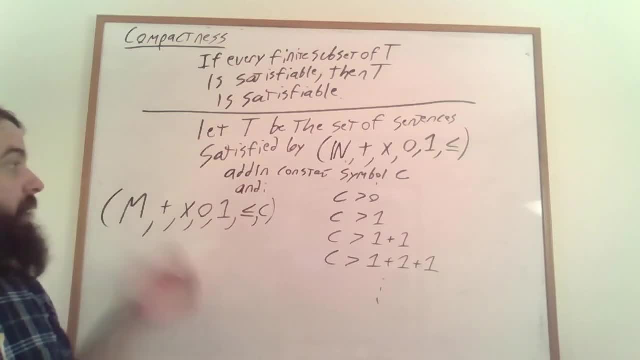 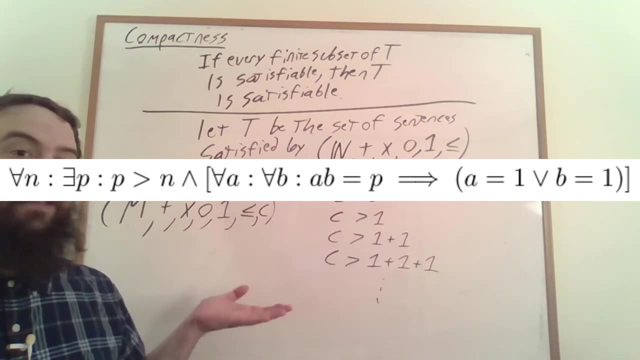 because it has infinite elements but nonetheless satisfies all of the same first-order logical properties, Including really complicated properties like the unboundedness of the prime numbers. So this structure here is actually going to have to have some infinitely large prime numbers in them. 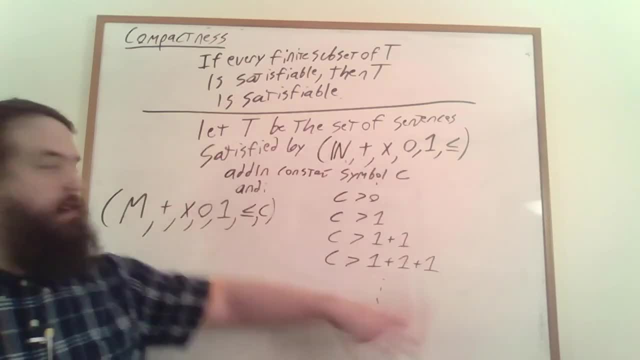 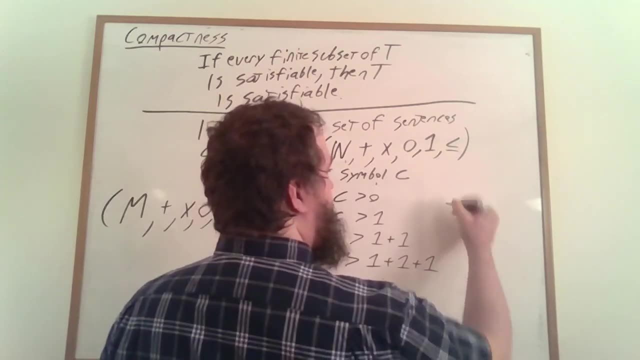 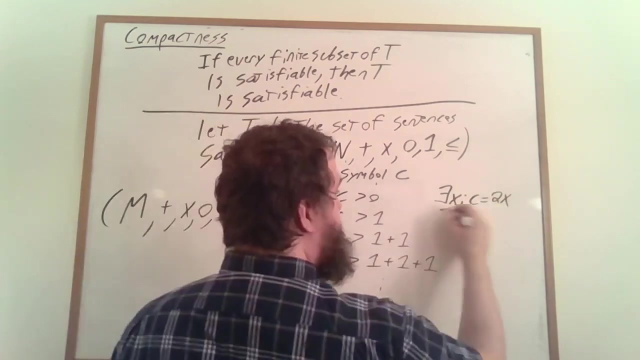 We can even go a step further in this construction and add to our collection that we're slowly collecting up here of formulas, a sentence that says that c is an even number And is divisible by 3. And is divisible by 4. And so on and so forth. 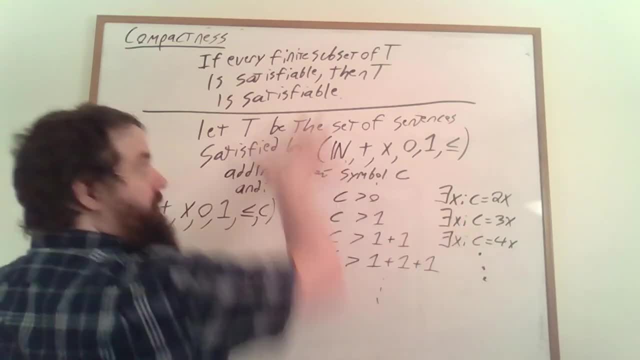 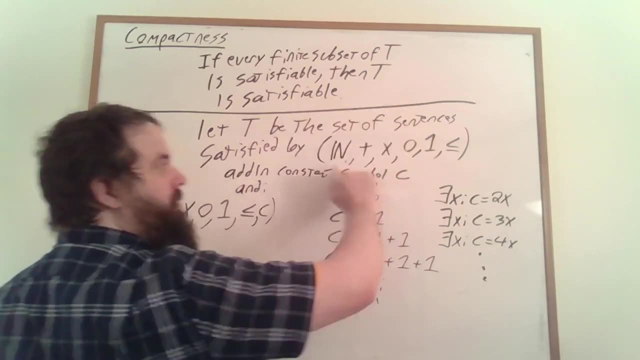 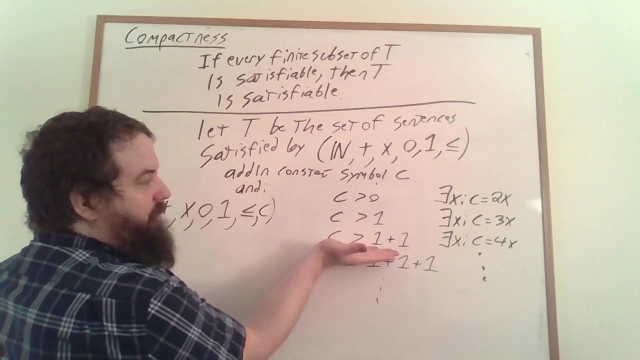 Any finite subset of this entire collection here. this entire collection t is going to consist of some finite number of sentences that are satisfied by this structure here, Additionally, some finite number of these sentences here. so it's going to cut off at some point. 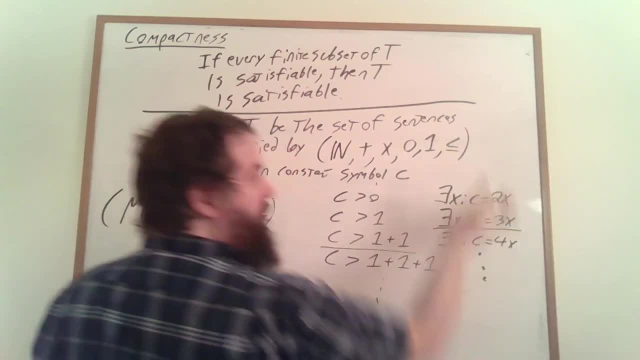 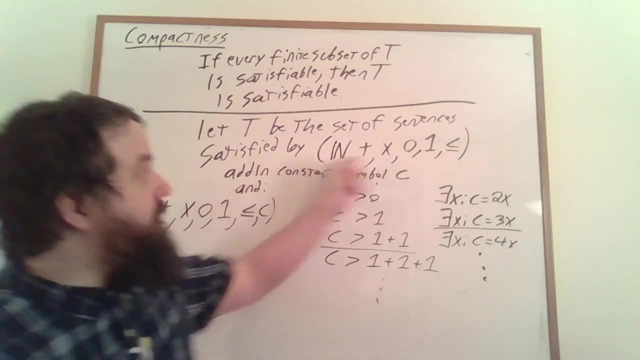 And some finite number of sentences from this list as well. And again there's going to be some assignment of c within this original structure that's large enough and divisible enough in order to satisfy this finite collection here. So every finite subset of this large collection here. 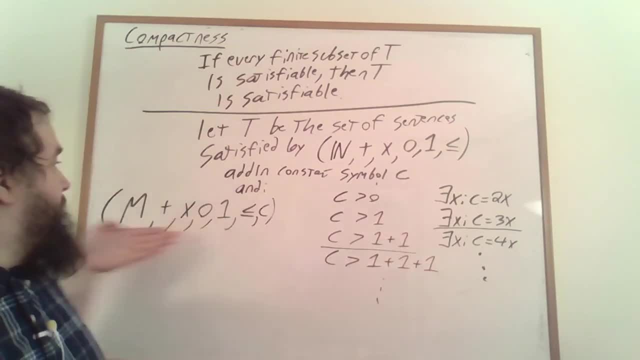 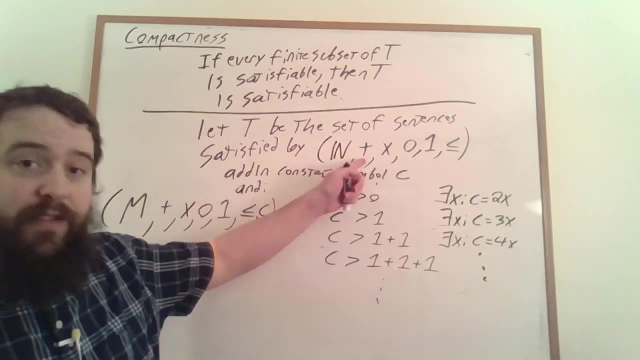 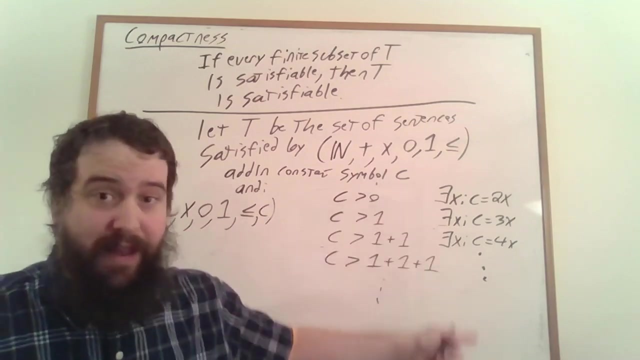 is satisfiable, And so there's going to be a model that satisfies the entire collection. Again, it can't be this structure with a particular assignment to the constant symbol c, because that's just not going to work with infinitely many of these sentences here. 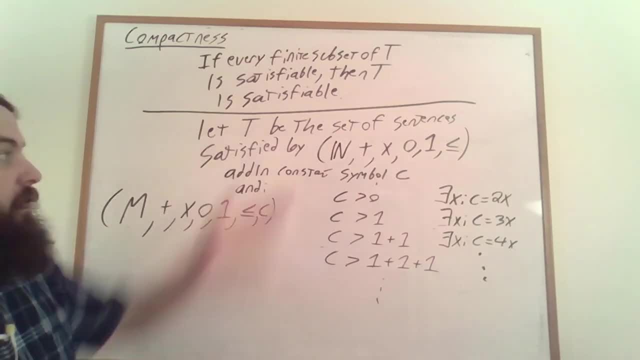 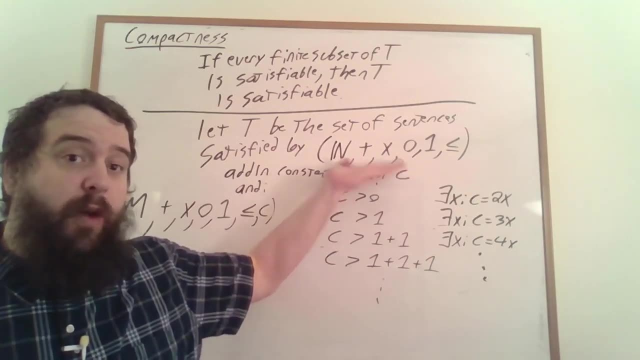 It has to be some other structure that's for the most part identical to the natural numbers. It's identical in the set of first-order logical properties that it satisfies, But it has an element c which is not only larger than every natural number. 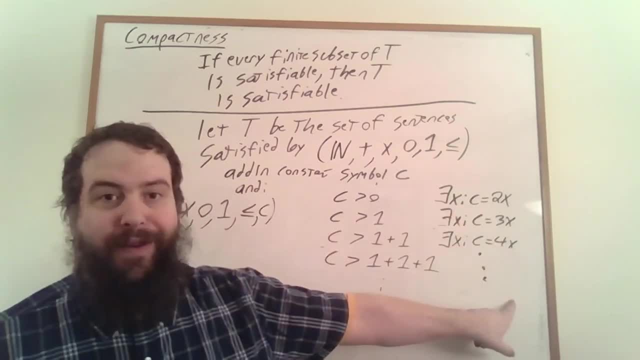 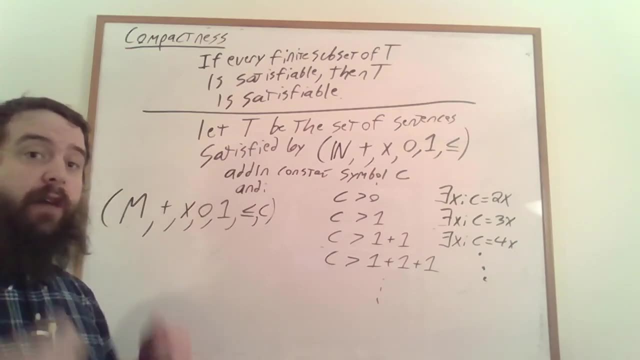 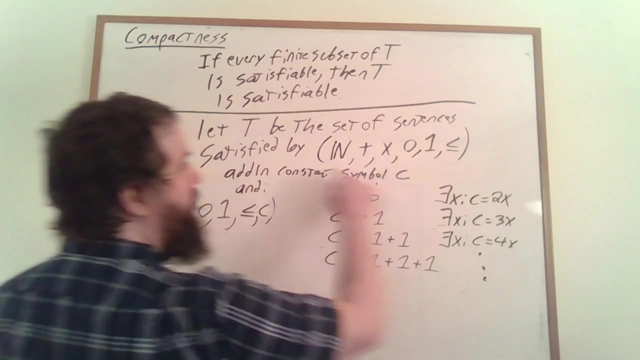 but it's also divisible by every natural number. It's worth noting that, while we were able to get a really tight handle on the non-standard models of the natural numbers, with just 0 and successor non-standard models of this structure, here the natural numbers- 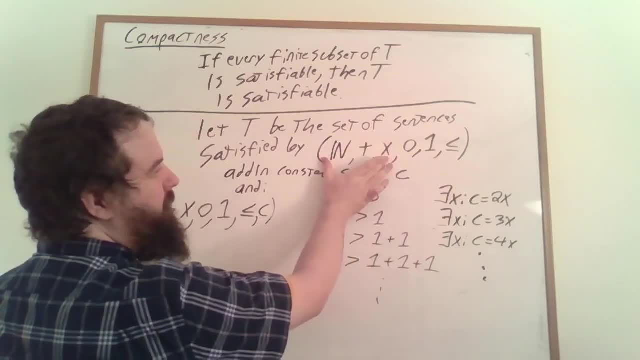 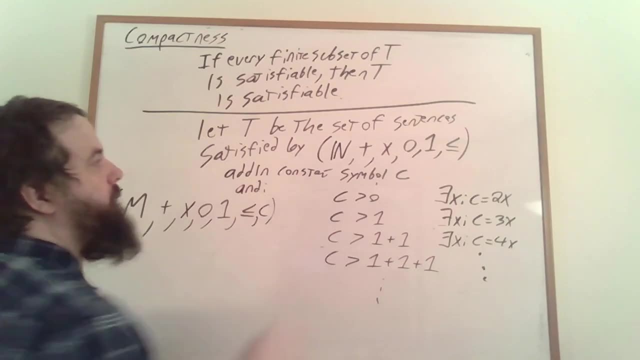 even if we're just looking at the natural numbers with addition and multiplication- because again, these are kind of redundant things that we can syntactic, sugar our way out of- even if we're just looking at the natural numbers with addition and multiplication, finding a non-standard model of that. 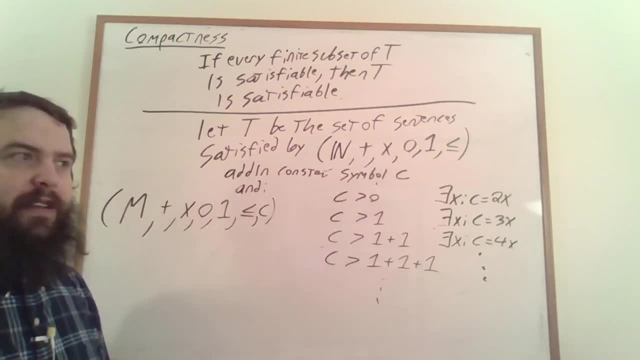 actually constructing. that is not something that you can really do in a constructive, computable way. The compactness theorem says that there is a model that does this, but it doesn't give you much of a handle on what that model actually needs to look like. 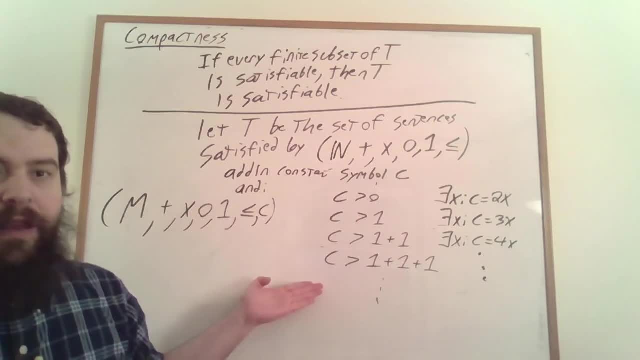 It's going to wind up having this infinite element in it, but it's also going to wind up having, like that infinite element divided by 2 rounded up, or I guess that infinite element is divisible by 2, so we can just say: 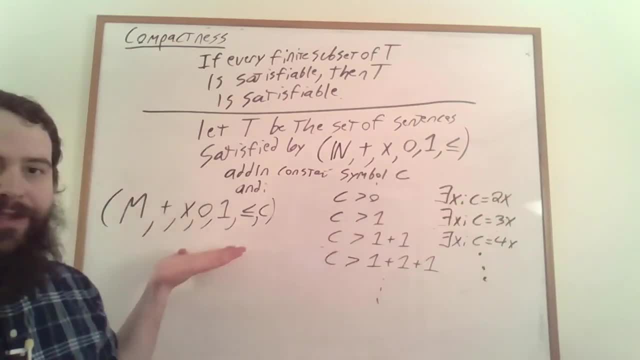 that infinite element divided by 2 is going to be in this structure here, or that infinite element divided by 3. There's going to be, or that infinite element times itself. There's going to be a whole bunch of stuff that we're going to have to add in here. 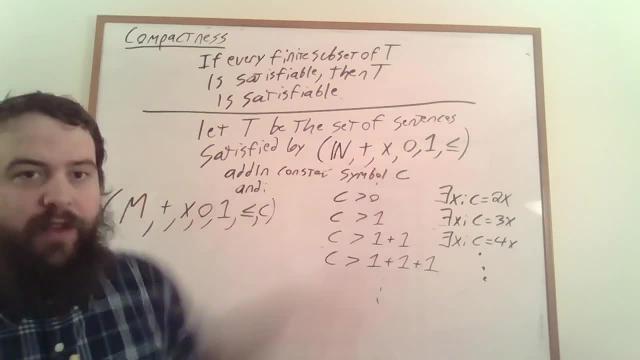 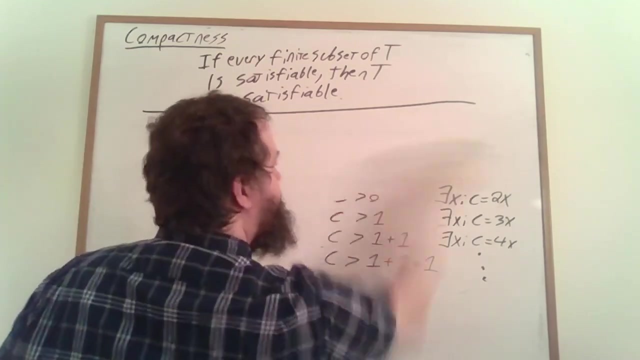 because we have more stuff in this structure in order to get this to satisfy the same first-order logical properties, and it turns out that the resulting structure is just. it's really gross. It's not something that you can get a nice concrete, computable handle on. 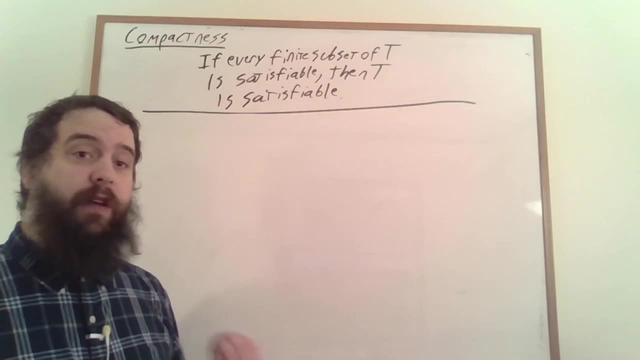 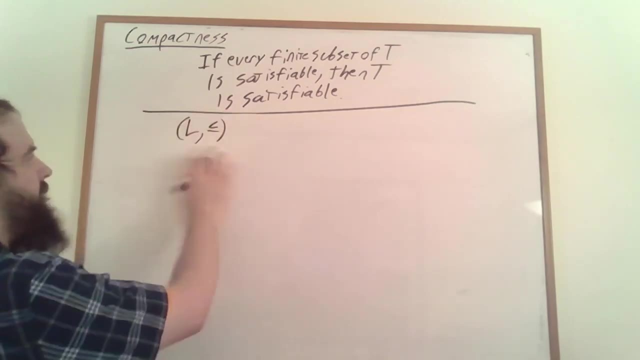 Finally, let's do one last application of the compactness theorem. Let's say that we have a structure L, which is some linear ordering, and that means that we have a set of elements and a notion of ordering on them that satisfies these axioms here. 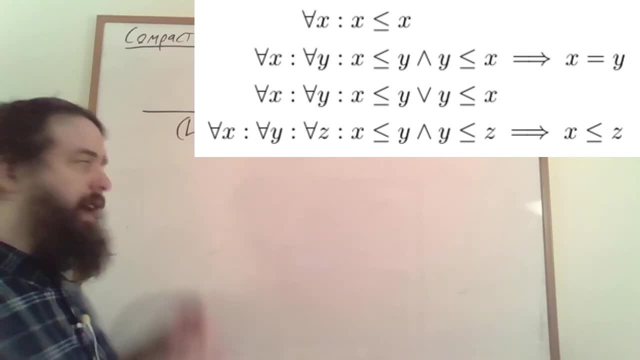 Intuitively, we can view the elements of the structure as falling along a number line where elements further to the right are larger than elements further to the left. Of course, these structures might be grossly infinite in ways far beyond the traditional number line. 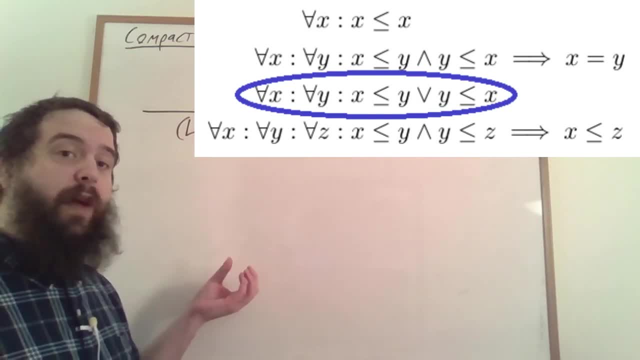 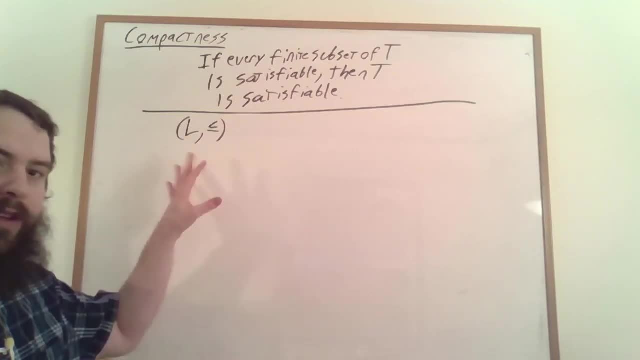 but the fact that we can compare any two elements really gives it this linear structure to it. So we're going to start off with this linear ordering and we're not actually going to do compactness to it. We're going to use it to do compactness again. 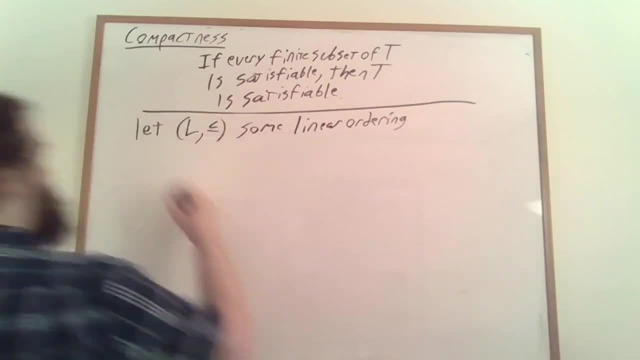 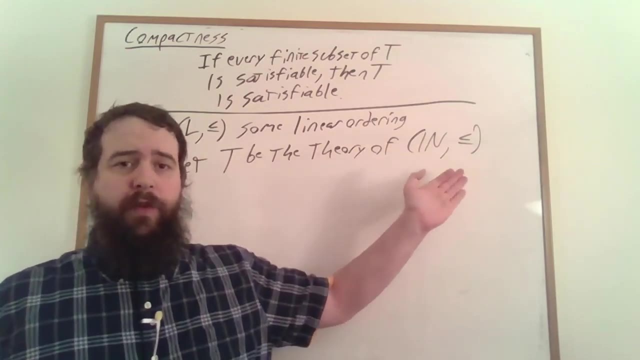 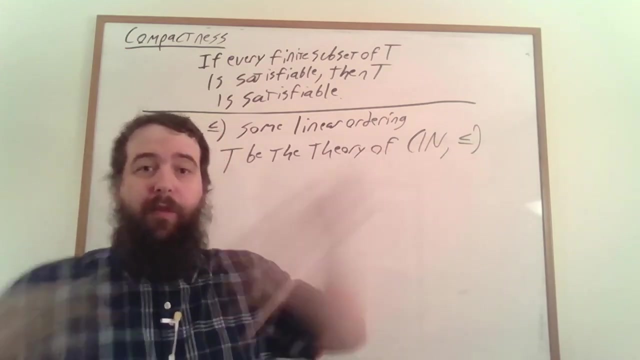 to the natural numbers, And here we'll just have the natural numbers with less than or equal to, to avoid having tons and tons of formulas that we can write. The more things that we have here, the more formulas that we can write, the more things. our non-standard models. 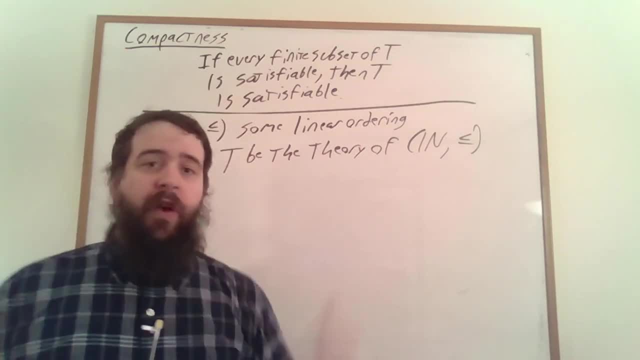 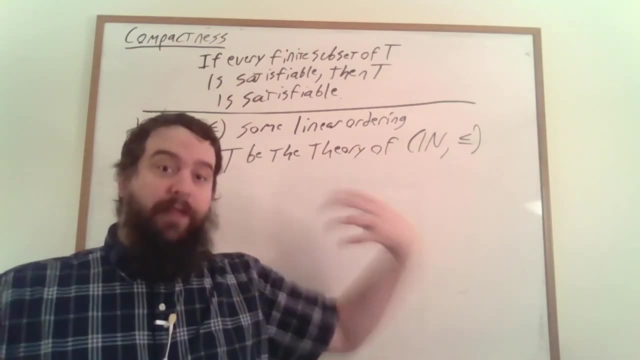 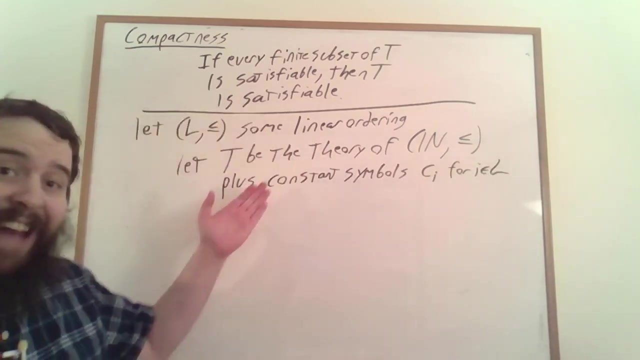 the models that are constructed by compactness are going to have to satisfy. So the fewer things that we have, the easier it's going to be to construct these models that compactness tells us must exist. Plus, we're going to add an infinite number of constant symbols. 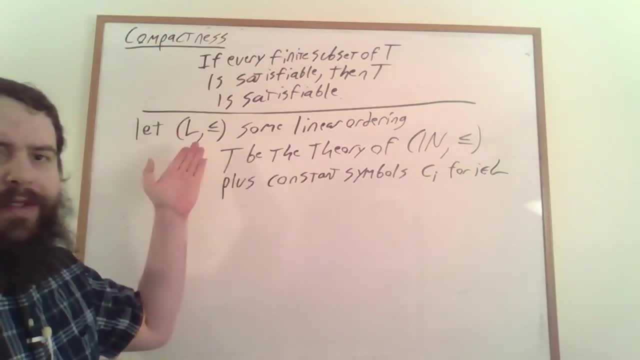 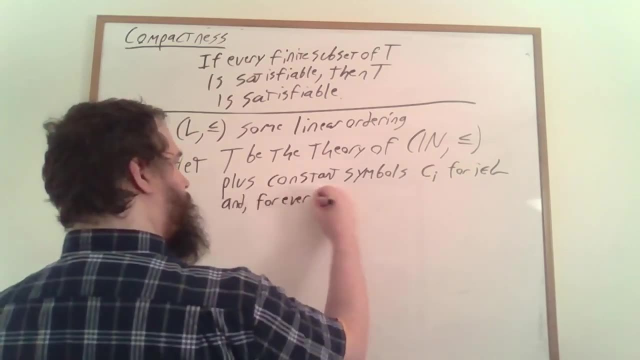 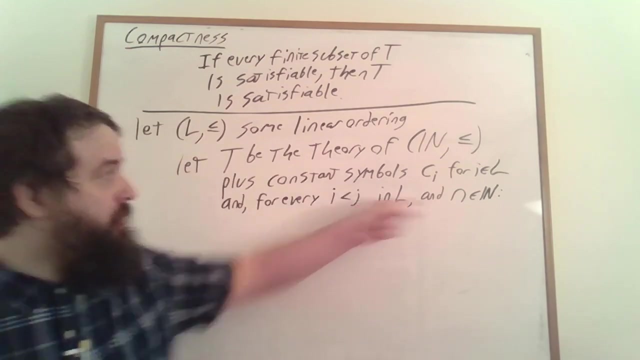 Potentially, It depends on what our original linear ordering is. We're going to add one constant symbol for every element of our original linear ordering And we're going to add in a formula for every pair, i and j in L and every natural number n. 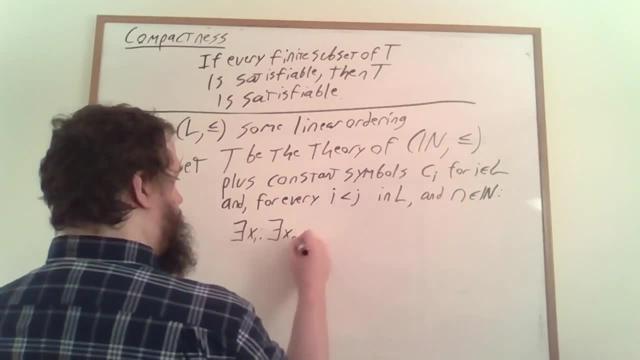 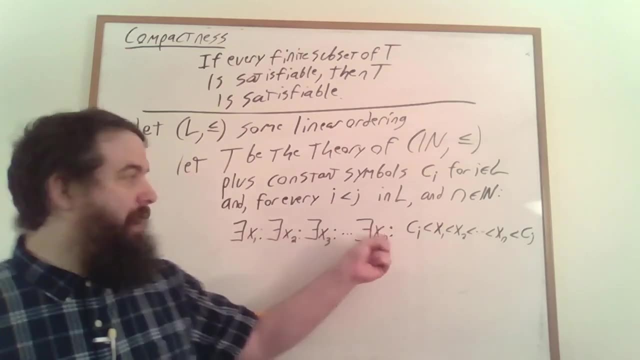 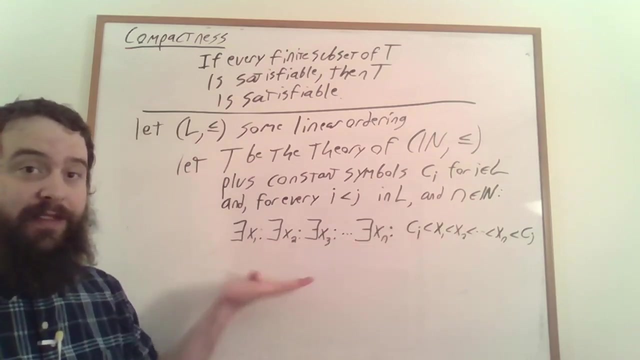 Some formula that looks like There are n elements, and we can do this because n is actually an actual finite number, So we can actually construct a formula that looks like this and toss it into our set. There are at least n elements, strictly between c, i. 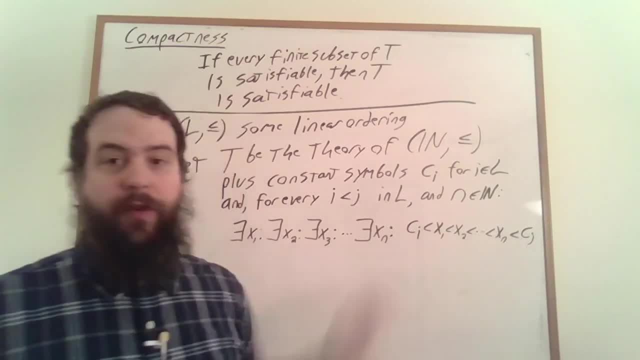 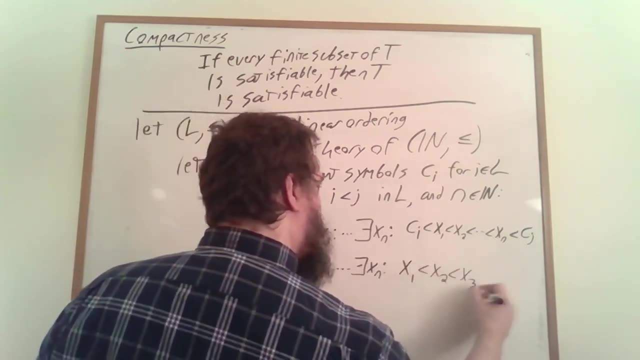 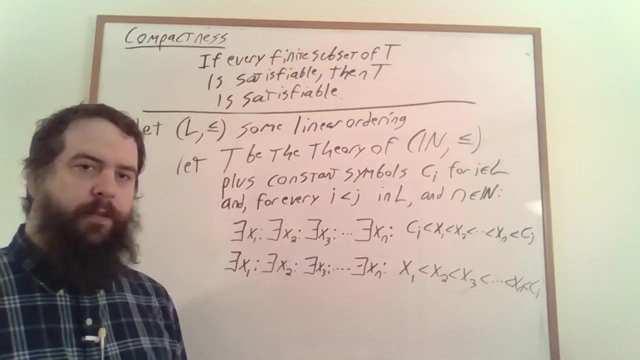 and c j, and c j is larger than c i, And we're also going to have to require that that c i is strictly larger than at least n different elements. So we have one infinite collection of formulas here and another infinite collection. 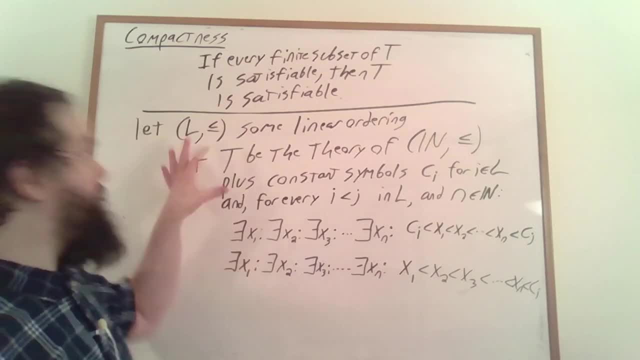 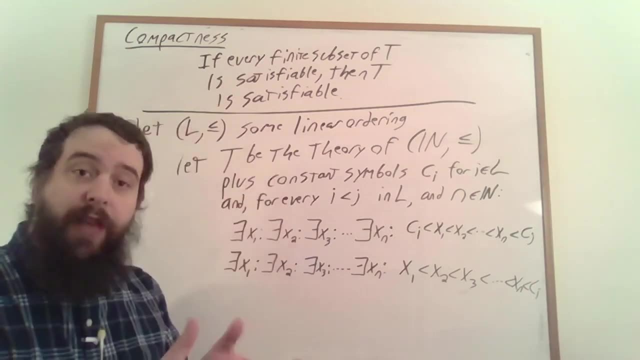 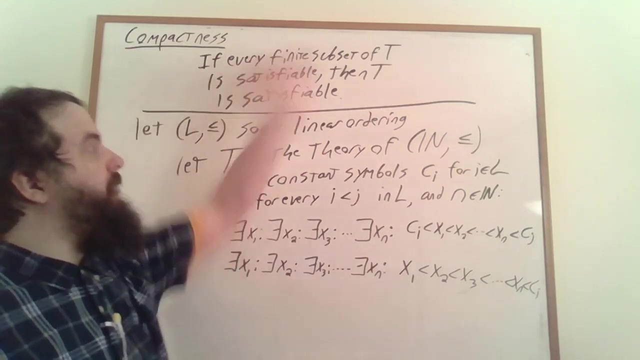 of formulas here, and then, of course, another infinite collection of formulas, which is the theory of the natural numbers with less than or equal to. We union together all of these infinite collections and we run it through the compactness theorem: Every finite subset. 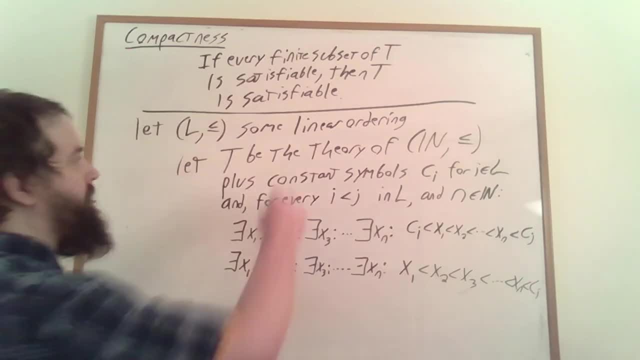 of this collection here is going to be some finite set of sentences that are true of the natural numbers with less than or equal to. some finite collection of sentences here and some finite collection of sentences of this form here. Together, these are only going to refer. 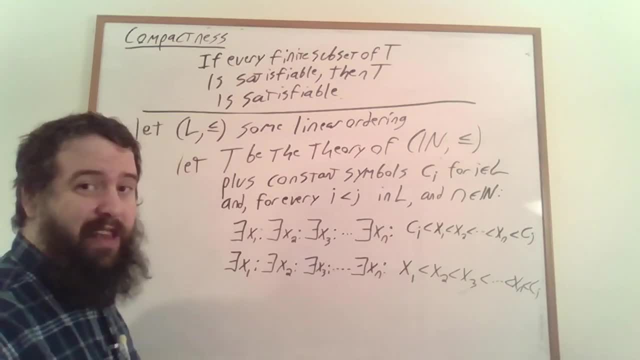 to finitely many of the c? i's Right. There's only going to be finitely many of the c i's that are referred to by formulas of this form. There's only going to be finitely many of the c i's. 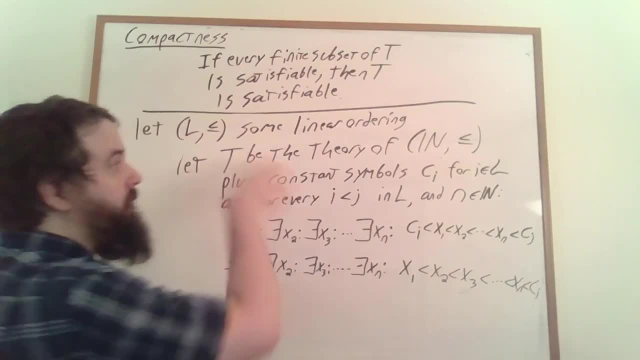 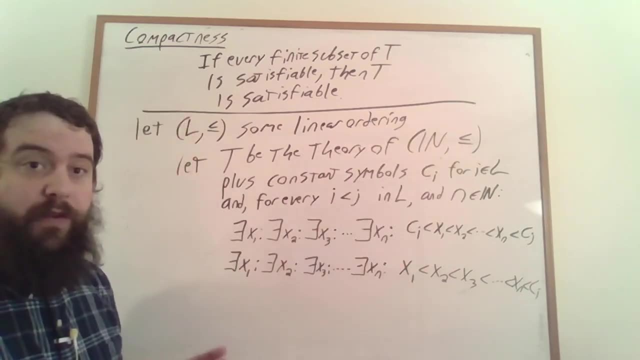 referred to by formulas of this form, And there's only going to be, Well, formulas from the theory of the natural numbers with less than aren't going to refer to c? i at all. So we have a finite subset here, Only finitely many. 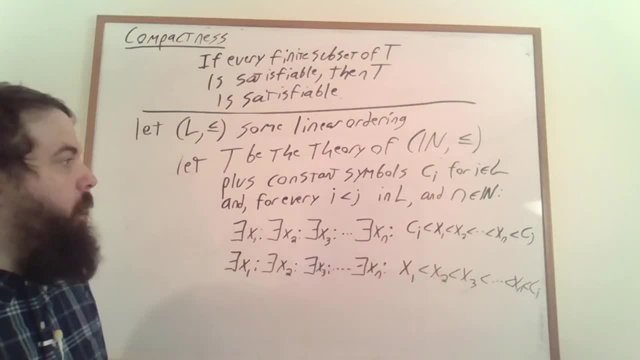 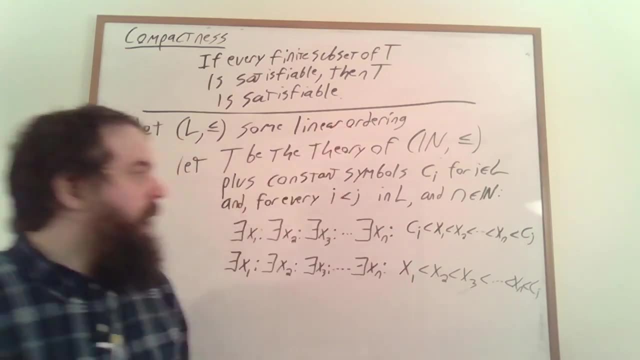 of the c i's are going to be referred to. We'll assign all of the other c i constants to just be 0 or pick a random number, And then we have to be a little bit careful about the c i's that actually get referred to. 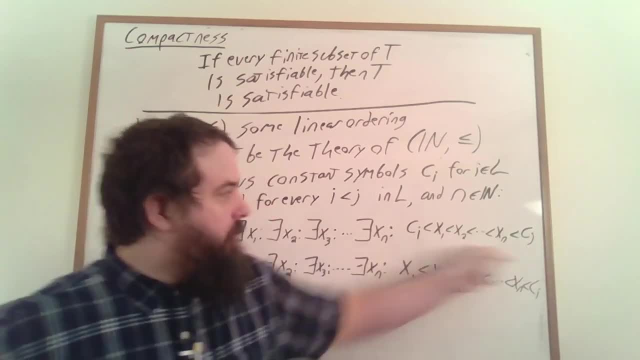 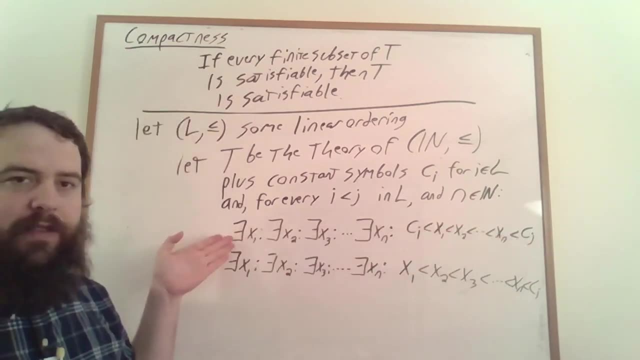 They're going to have to be far apart from each other. But again there's like a maximum n that's going to show up in any formula of this type from our finite collection that we're looking at, And a finite n which is the maximum. 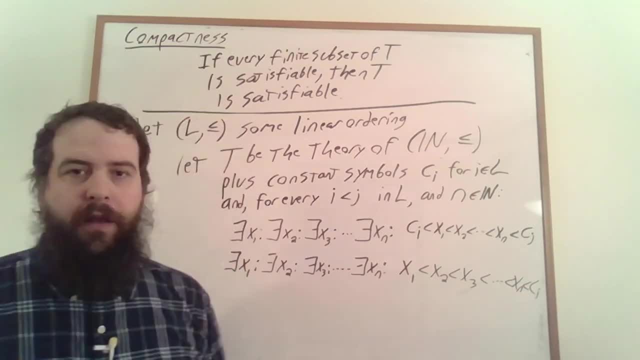 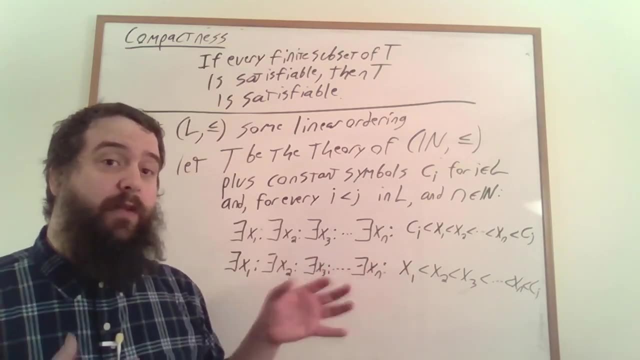 that shows up in formulas of this type, requiring that c i be far away from 0. And so, by picking the finitely many c i's that actually get referred to, carefully and far apart from each other, but assigning them to some finite numbers, 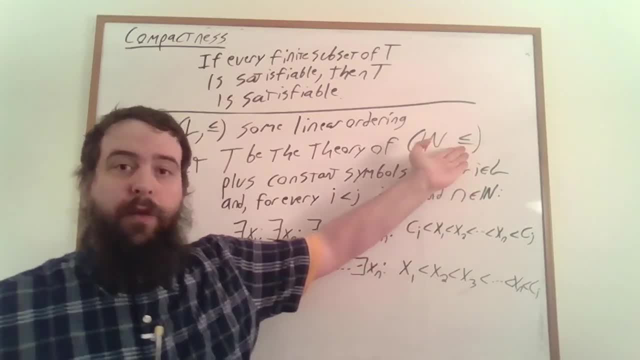 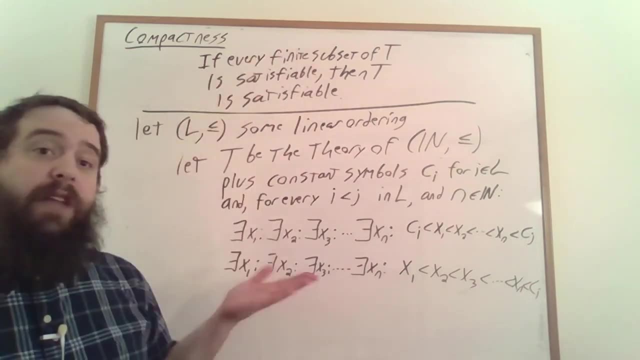 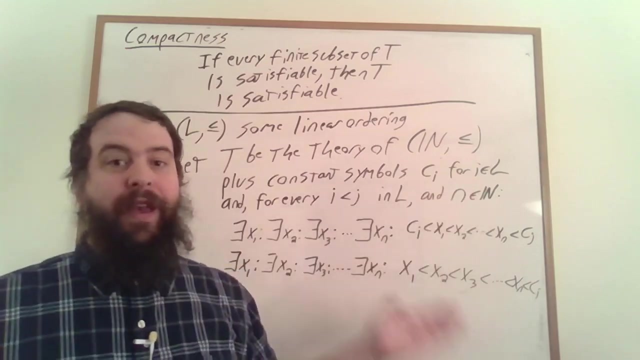 in the natural numbers with less than or equal to, then we can find a way of satisfying our finite subset of t, And we can do this for every finite subset of t, And so, by compactness, this entire collection of formulas has to be satisfiable. 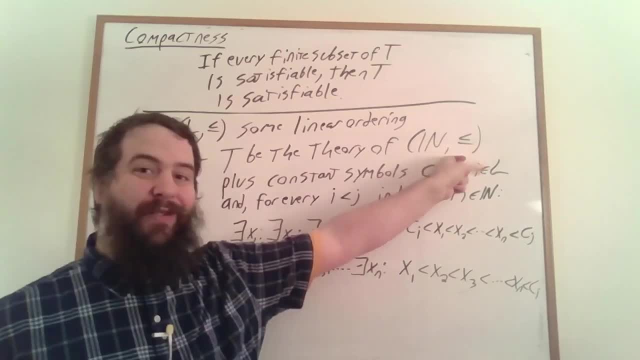 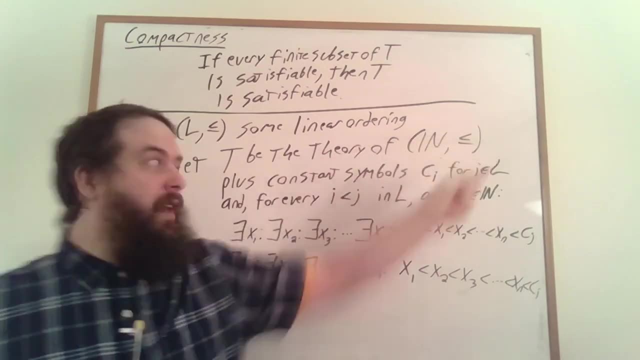 But again, it's not going to be satisfiable by this structure here. It's going to be satisfiable by a structure that shares the same theory, the same first-order logical formulas, but it's got a bunch more elements so we can do this assignment. 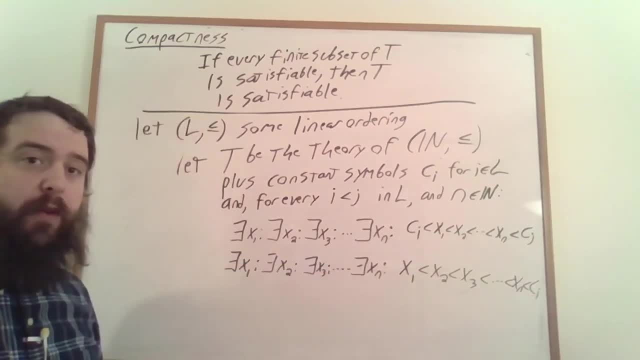 of the c i's. Let's be really concrete for a moment, and let L be the set containing 0,, 1, and 2.. This is a linear ordering under the standard notion of ordering, And so we're only going to add in. 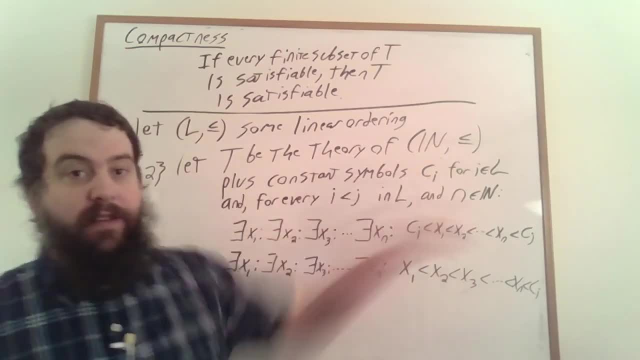 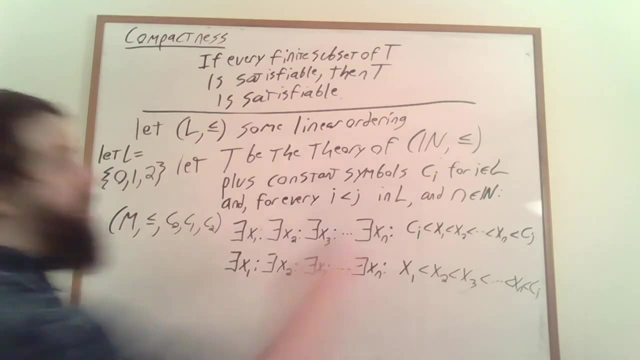 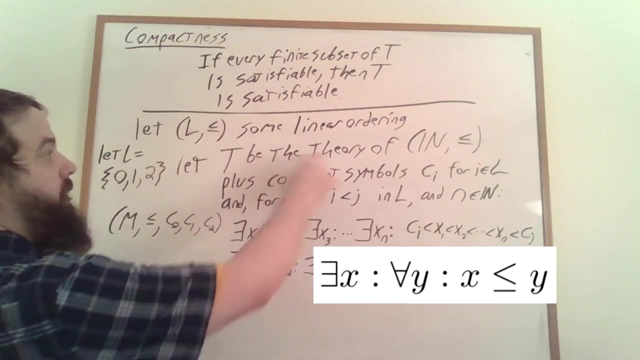 three constant symbols: c 0,, c 1, and c 2.. This structure here, that compactness gives us, is necessarily going to have a smallest element, because this structure has the smallest element, and so therefore, this sentence is in the theory, and so therefore, in t. 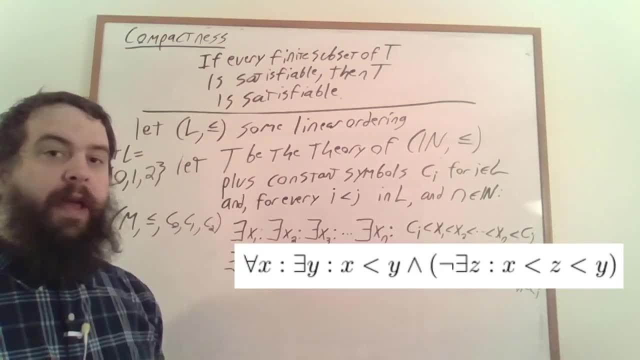 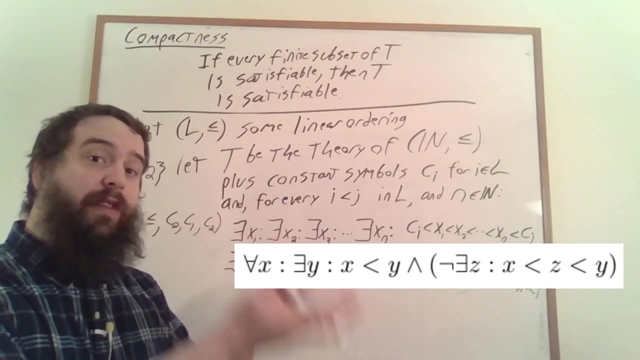 So this structure has a smallest element, and every element of this structure has an element immediately after it which we can write like this: Therefore, this formula is within the theory t, and so therefore also has to be true of this structure here. So we have an element. 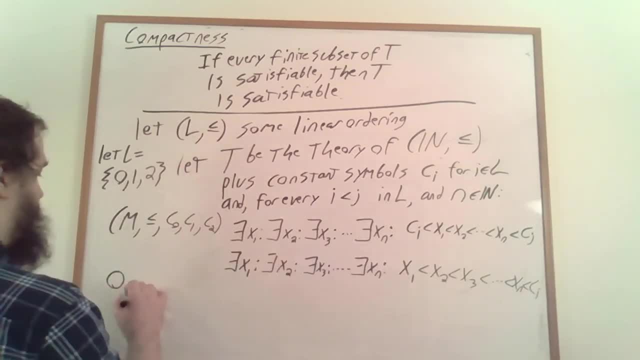 that's immediately after 0, and that's going to be 1 and 2 and 3 and 4 and so on and so forth. We're going to have elements immediately after each one, Because the c- i's all satisfy these formulas here. 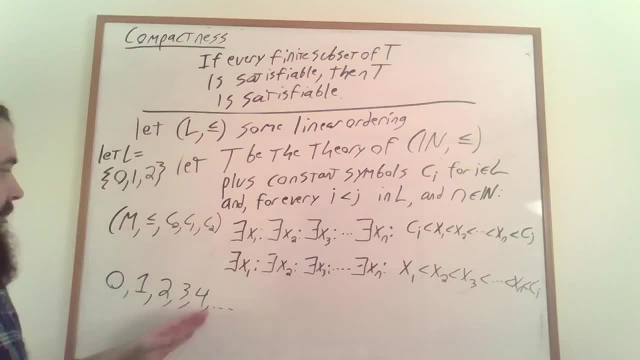 for all n, c. i can't be assigned to any of these numbers here. It's going to be the case that c 0,, c 1, and c 2 are all going to be larger than all of these elements here. Additionally, we required that. 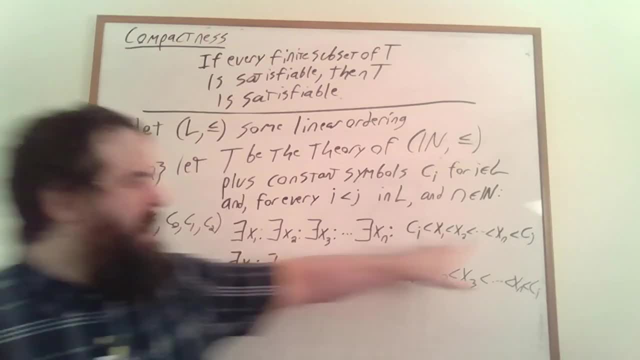 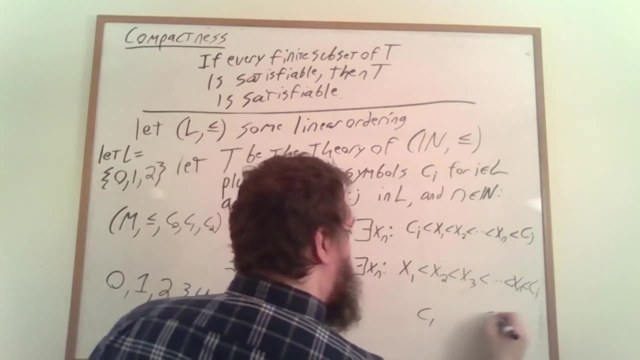 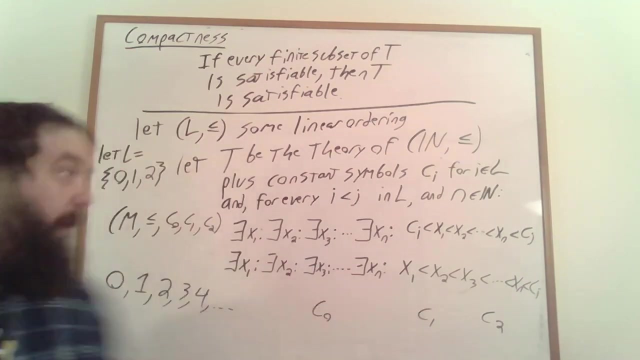 if i is less than j c, i is less than c- j, so we have an element c 0 here, c 1 here and c 2 here in this order. This is the order that they're going to show up within this structure here. 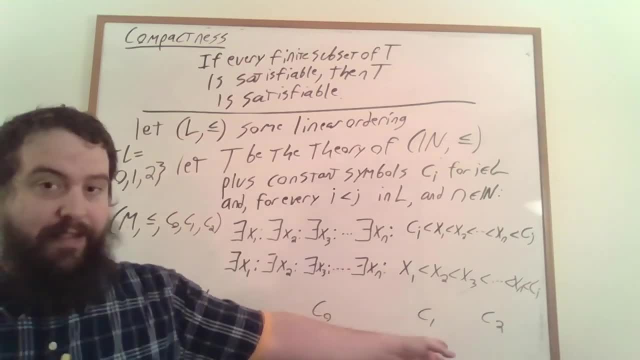 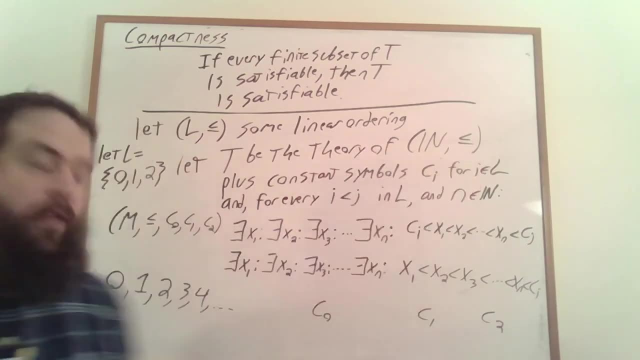 It's necessarily the case that c 0 is less than c 1 and that c 1 is less than c 2.. Again, within this structure, every element has a successor, so we also have c 0 plus 1, c 0 plus 2,. 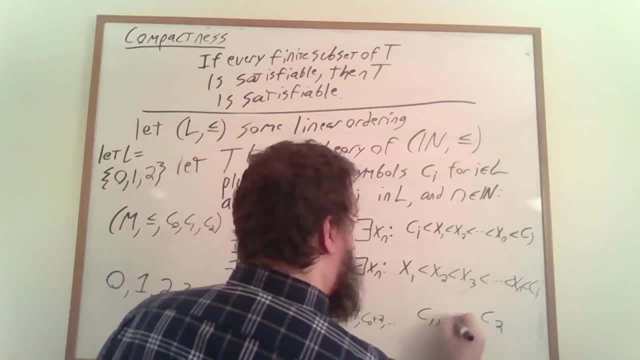 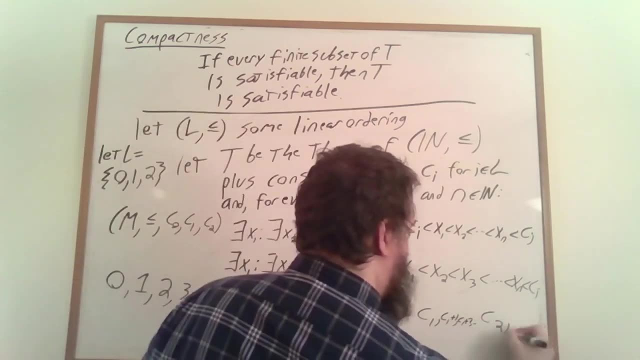 so on and so forth: a c 1 plus 1, a c 1 plus 2,, so on and so forth. and a c 2 plus 1, c 2 plus 2, and so on and so forth. 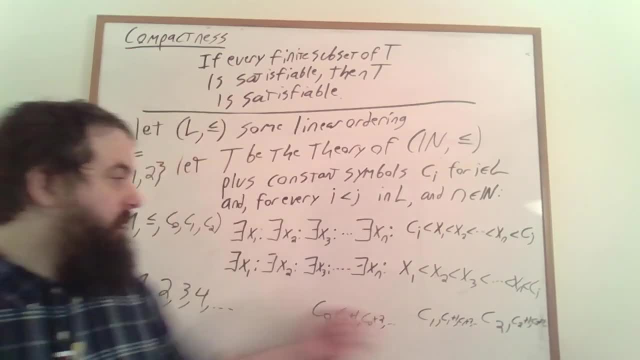 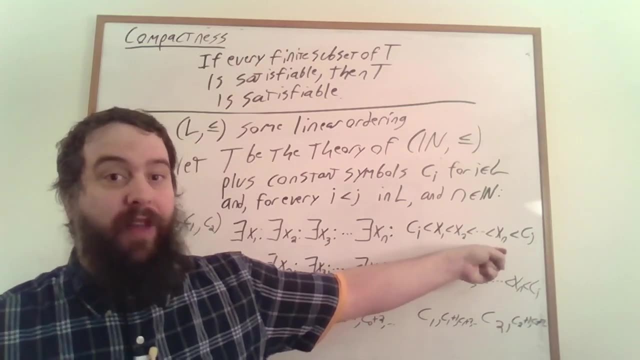 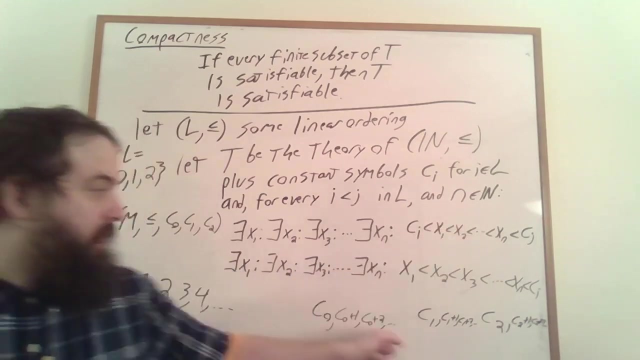 None of these elements are equal to each other, because c 0,, c 1, and c 2 are more than n elements apart from each other for all natural numbers n. so they're infinitely far apart from each other. So none of these new elements. 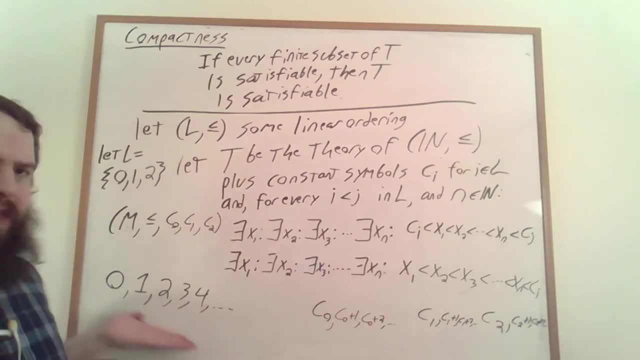 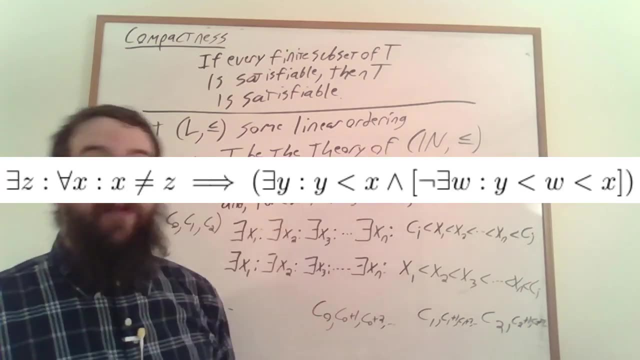 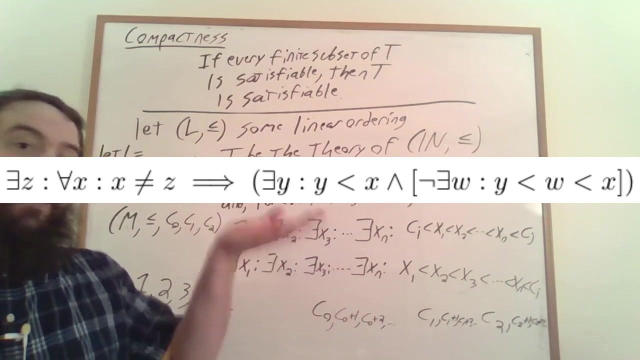 are any of these or any of these? That would be kind of weird, because everything's in this order. Additionally, in this structure, every element has an element immediately before it other than 0, which we can write like this: So again, this formula here: 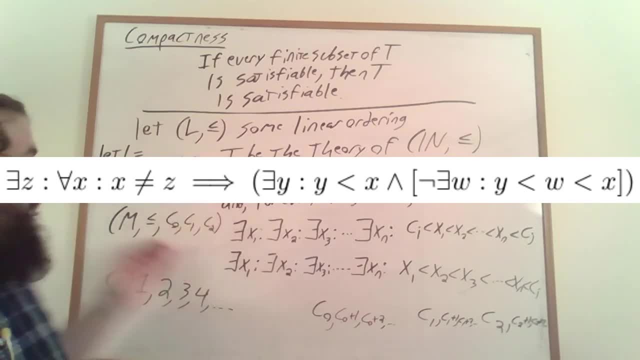 is within the theory and therefore is satisfied by this model here, and so therefore this model had better satisfy that every element has an element immediately before it. So that's going to give us c 0 minus 1, and that element has an element. 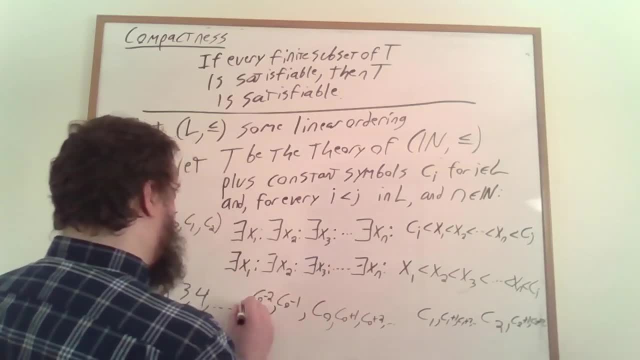 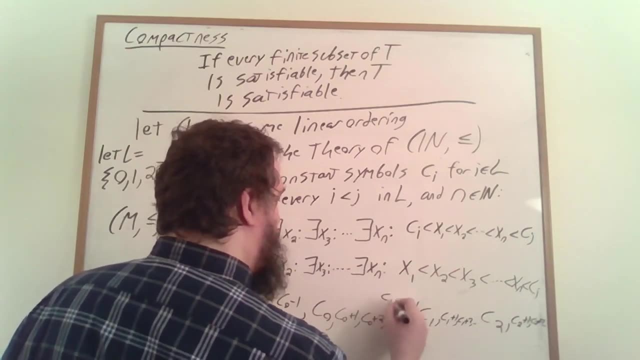 immediately before it c 0 minus 2, and so on and so forth. c 1 is going to have a c 1 minus 1, a c 1 minus 2, and so on and so forth, and c 2 is going to have. 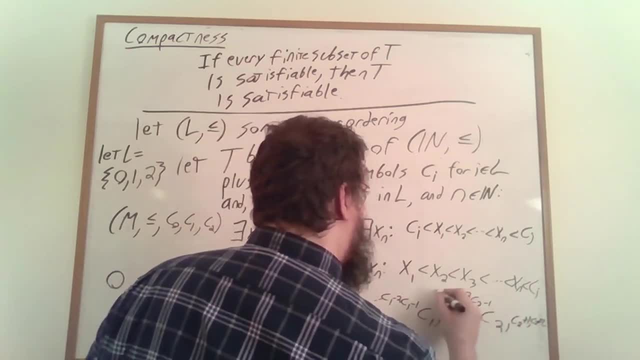 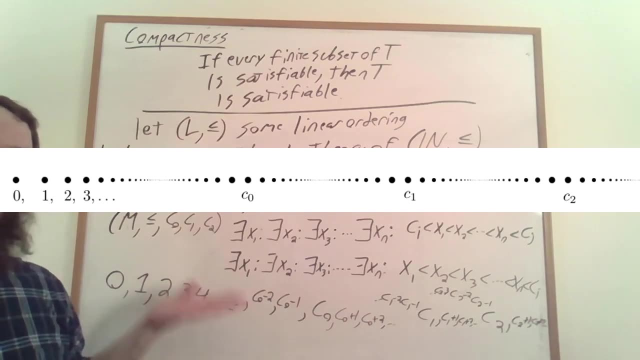 a, c 2 minus 1, c 2 minus 2, c 2 minus 3, and so on and so forth. I'll put a picture on the board of what this linear ordering is supposed to look like. and this turns out to be it. 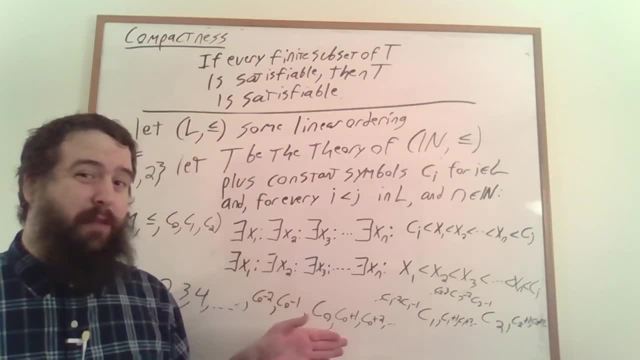 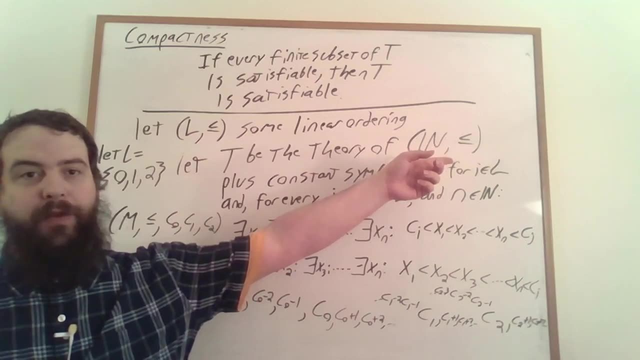 Although, again, why do we know that this winds up being it? Why do we know that this structure here actually does wind up satisfying all of the true sentences of the natural numbers with less than? You'll have to watch the next video to find out why. 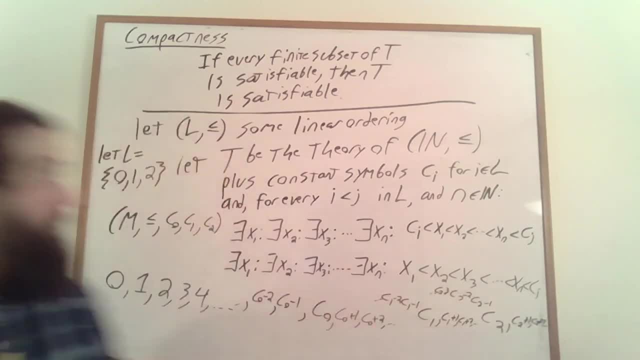 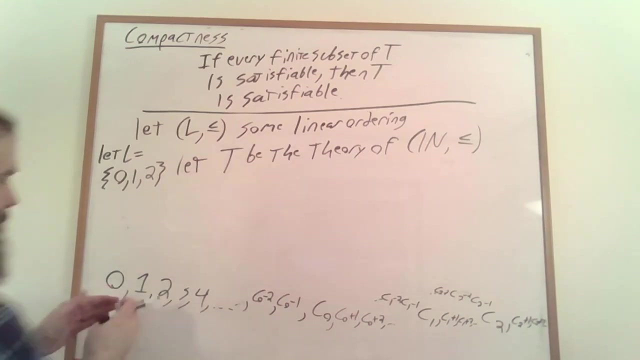 but this structure here satisfies all of the sentences within T. It is a structure that satisfies all of the same first-order logical sentences as the natural numbers, but is obviously not the same structure. It's a different structure. In particular, this structure looks like: 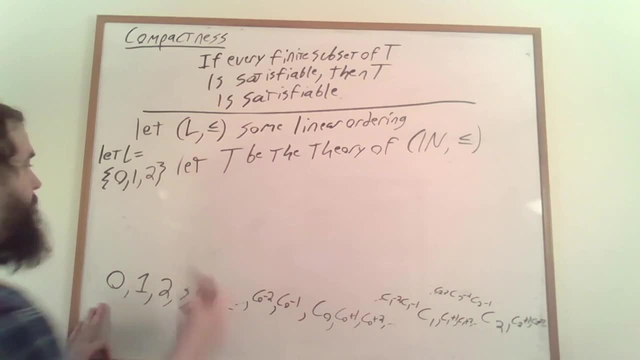 a copy of omega, a copy of the natural numbers followed by: in terms of linear orderings, we use plus to indicate that something is followed by something else, followed by this ordering here, which looks a lot like the integers right. 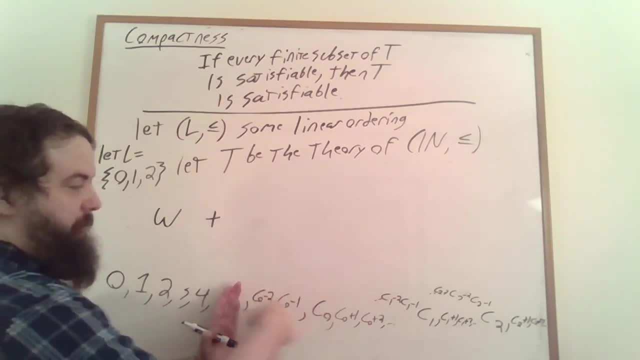 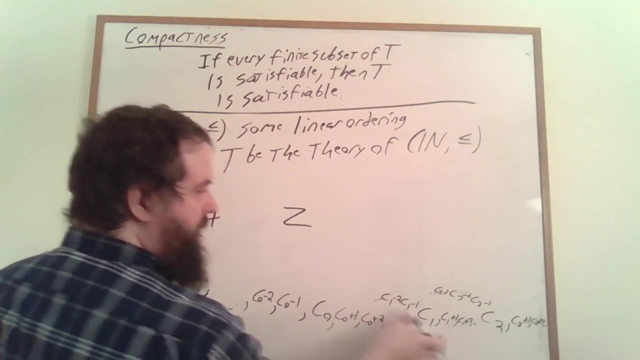 It starts off at zero. It goes infinitely backwards, infinitely forward. You can take a step forward and a step backwards. So we have one copy of the integers, We have another copy of the integers for this bit. here again, these aren't going. 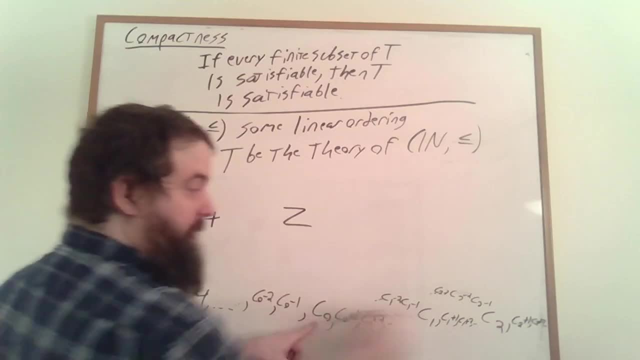 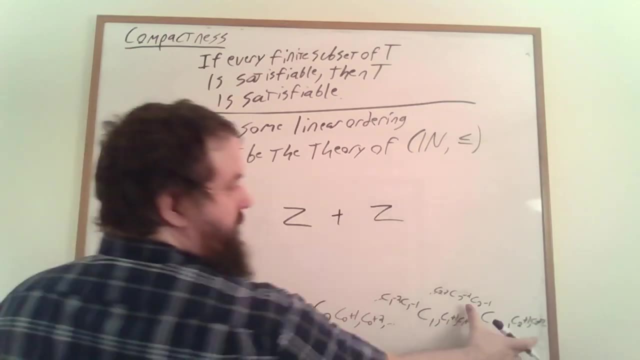 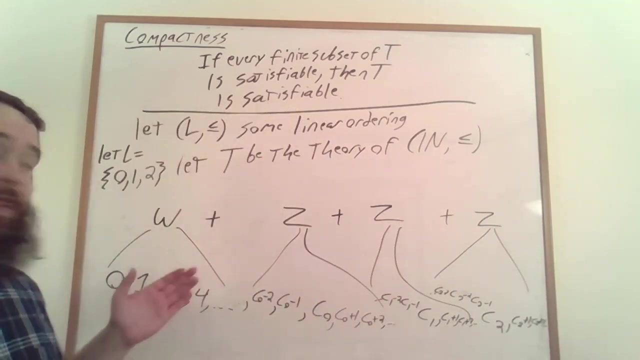 to be connected to each other because we required the ci's to be infinitely far apart. There's going to be another copy of the integers and another copy of the integers- It's helpful to think about this as omega- followed by one copy of the integers. 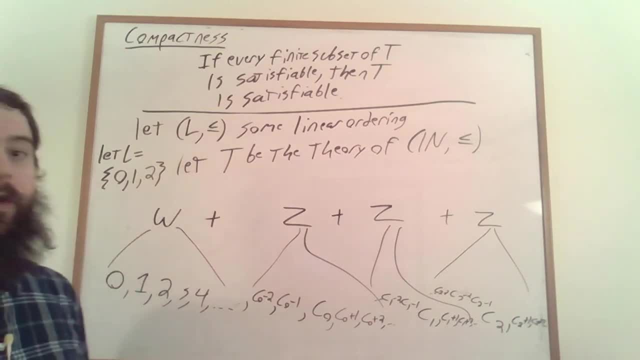 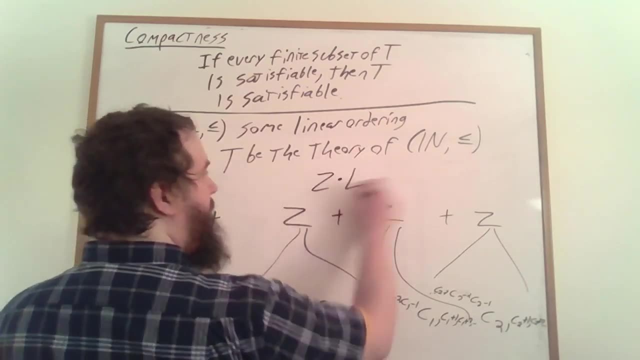 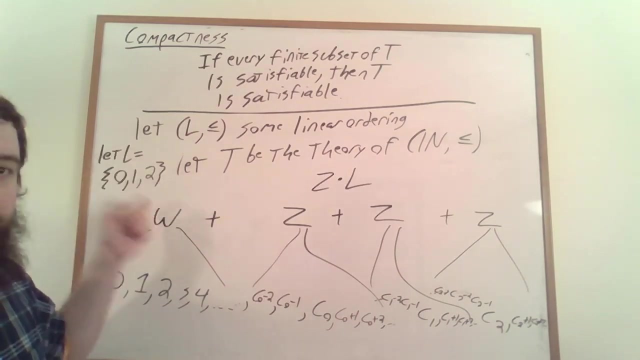 for each element of our original linear ordering L, which we like to call z times L. So in this case, our original linear ordering had three elements. Sometimes we call this linear ordering three, and so we can call this z times three. And, of course, 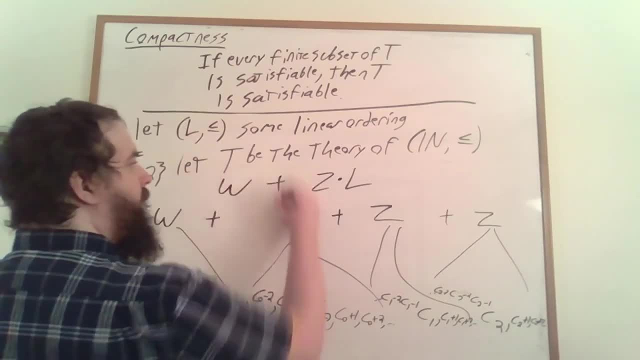 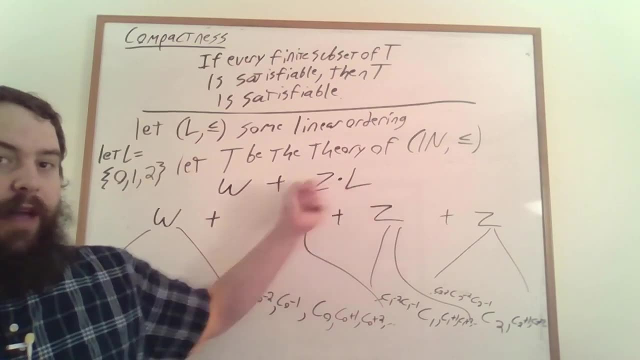 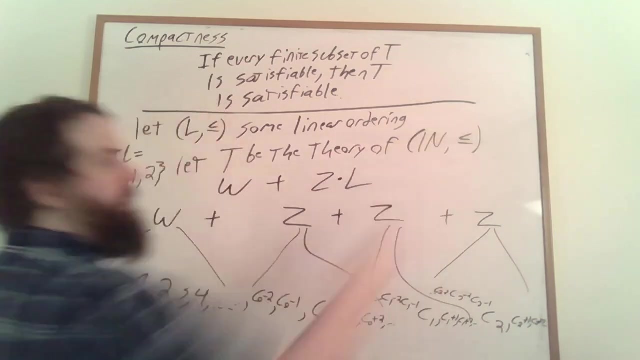 don't forget this- omega plus. And so we have this structure of the form omega plus z times L, L copies of z, which is a non-standard model of this original structure. here It satisfies all of the same first-order logical formulas as this structure here. 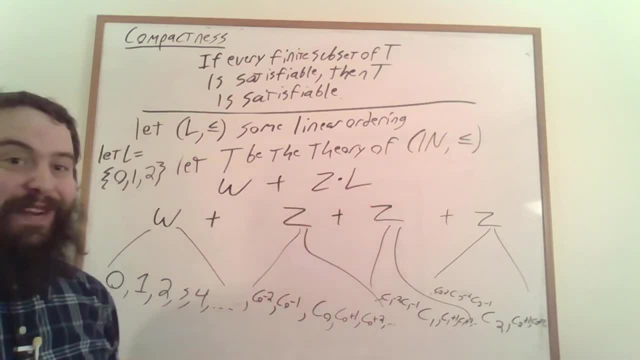 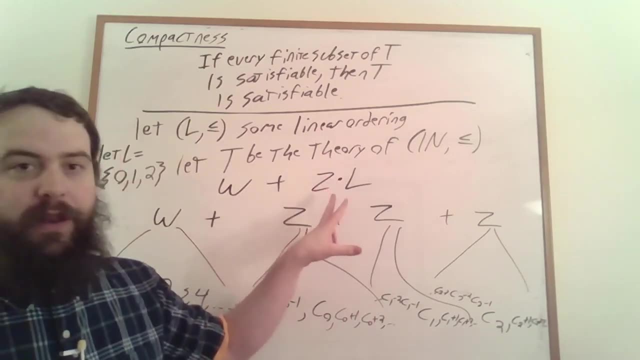 And, of course, it's not the same structure. It's very different. I like to call these linear orderings woozles, because I kept getting confused about the way that multiplication of linear orderings works, And this reminded me that this is. 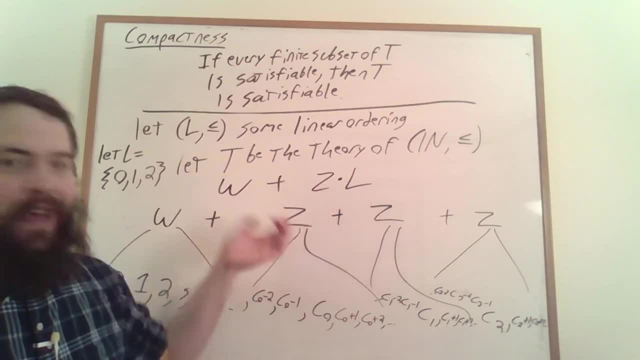 this is how multiplication of linear orderings works. It's omega plus L copies of z, And you can do this for any L and you can get a different, non-standard model of the natural numbers with less than or equal to. But why? 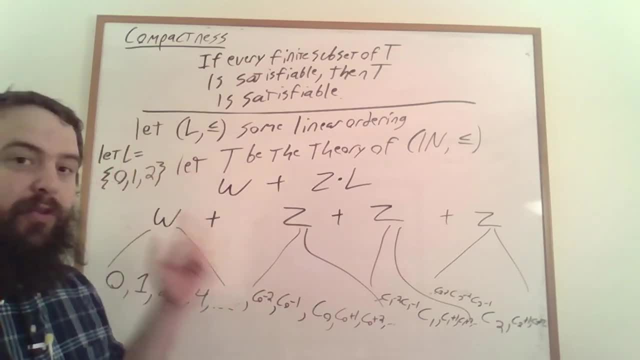 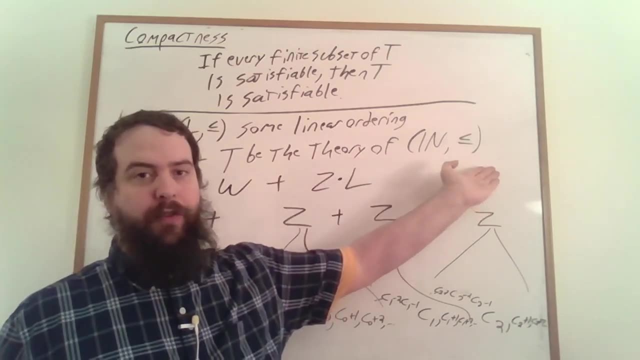 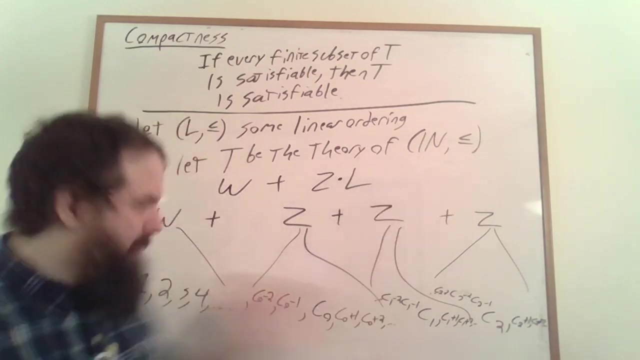 I want to stress that we haven't proven that this structure here satisfies the same first-order sentences as this structure here. It may be the case that there's some first-order sentence here that tells us that there have to be even more elements in this structure here.